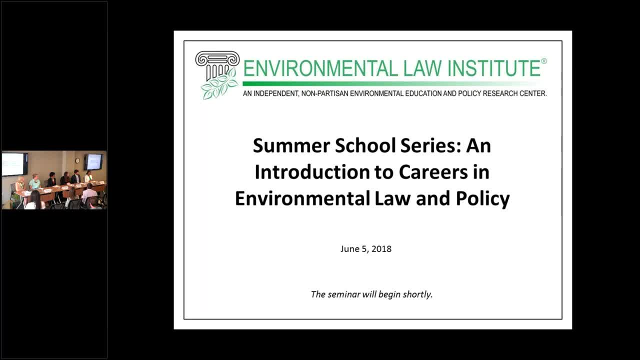 the Director of the Associates Program for Environmental Law and Policy and beyond Their career journeys. current work and role in environmental law and policy are diverse and significant. Full speaker bios are posted on our website, wwweliorg, and each panelist will share. 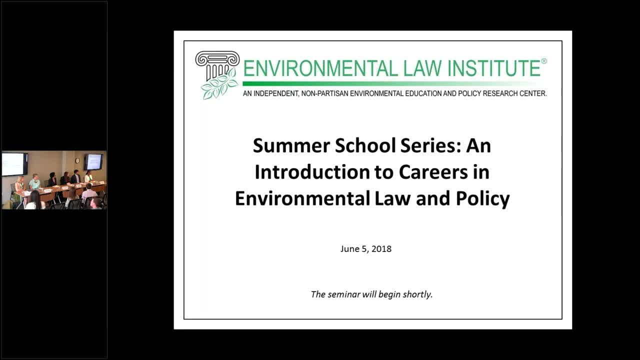 more about their path with you today. So with that, I'd like to let Colby, Bishop of National Geographics, start us out and we'll go through the panel. Thanks for joining us. Okay, Hi everyone, and thank you, Caitlin. 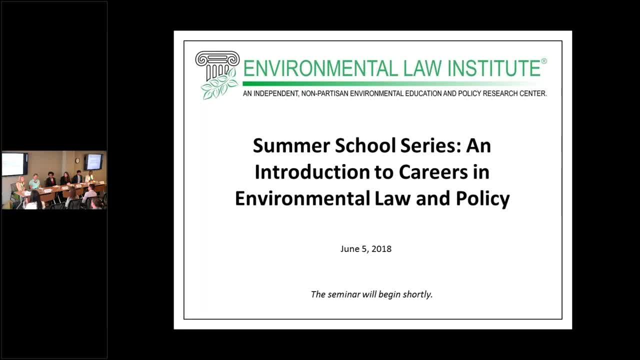 As she said, my name is Colby Bishop. I am the Director of Wildlife Programs at National Geographic, which is just half a block down. that way, If you guys haven't been there, we've got a great museum. You should come. Come on in Check it out. A new Titanic exhibit just 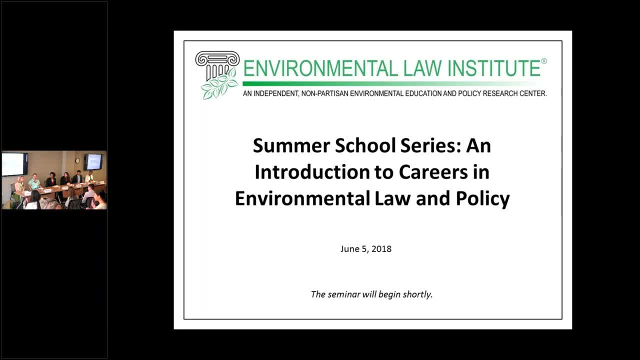 opened actually, Yep. So I thought I'd just tell you a little bit about my background, how I got into National Geographic. I've worked there for about 11 years in July, which is hard for me to believe. Time flies when you're having fun, to say the least. 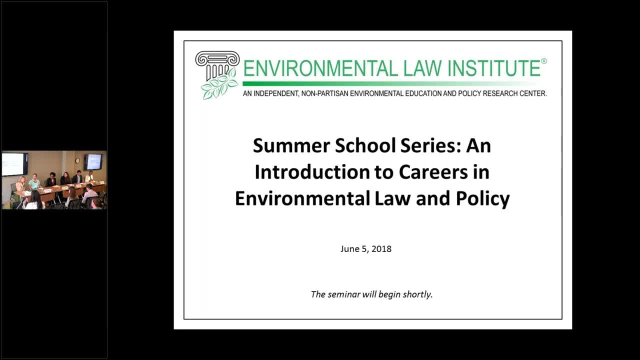 And talk about challenges, exciting updates and how environmental law fits into all of this, of course. So I'm from upstate New York originally, Actually, and I'm kind of a rural upstate part of New York near the Ithaca area. It's called Elmira New York, where I'm from. 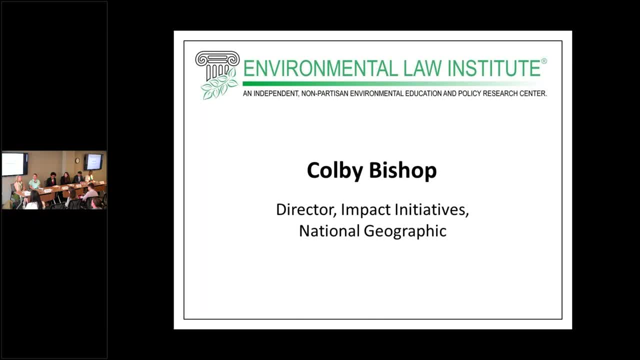 When I was in third grade, someone from National Geographic, from the MAPS division- it was somebody's family member, like an aunt- came to my third grade classroom and brought all of us these Blow up beach ball globes. This one I just tried to blow up, but they actually aren't better than. 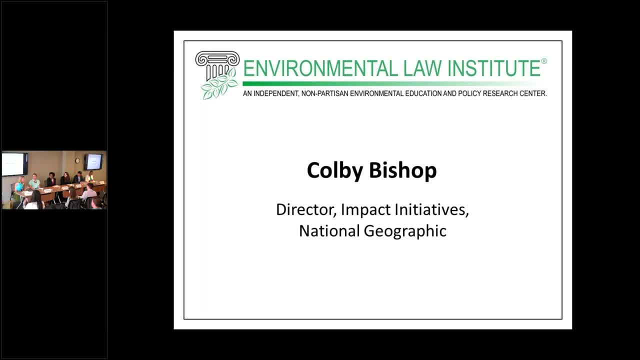 this And I loved the globe and I was so inspired by her and National Geographic. So, oddly enough, that all comes full circle here as I'm holding this globe. So I actually still have the globe she gave us. They're very durable. I guess It's at my parents' house at home. This is not. 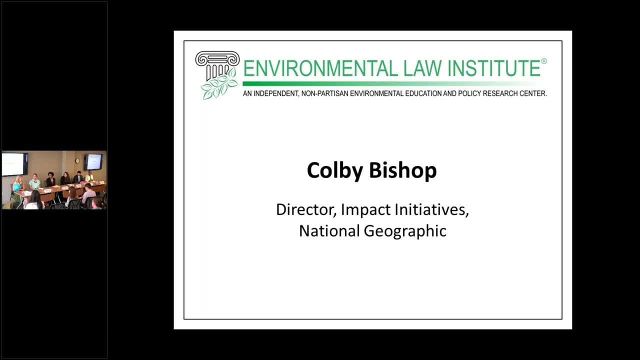 the original globe, but it looks very similar. But when I started my career at National Geographic I said: how much money do we have? What can I order? globes to hand out to students. So anyway, that's the story behind this half-inflated globe. 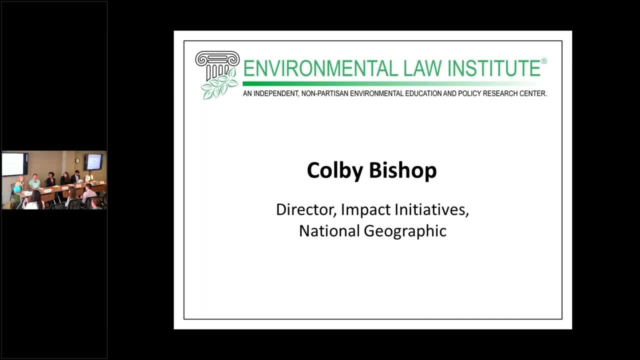 I went to college at Hamilton College, a small liberal arts school in upstate New York. I majored in world politics and Spanish. I was really interested in getting international experience, So I studied abroad in Chile for six months, Loved that, Got an undergrad, was able to. 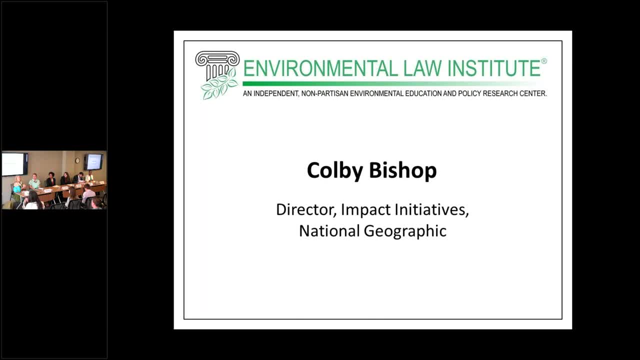 speak Spanish pretty fluently after that, so added Spanish as a second major. But the reason I chose politics was that I really liked the idea of international relations and working with global partners, global audiences, that kind of thing. So after college I was dead set: I'm moving to DC. 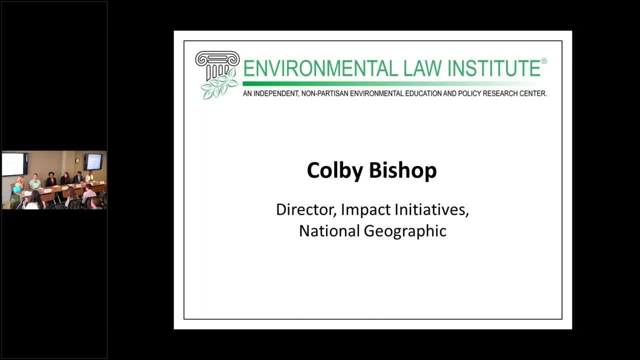 Now you guys are all here during the summer. It's a beautiful day now, but it is not all summer long. It gets pretty humid out, But anyway regardless. so I moved to DC with some of my friends from college. We lived in a group house, had lots of fun, But I got a job, most importantly, at the 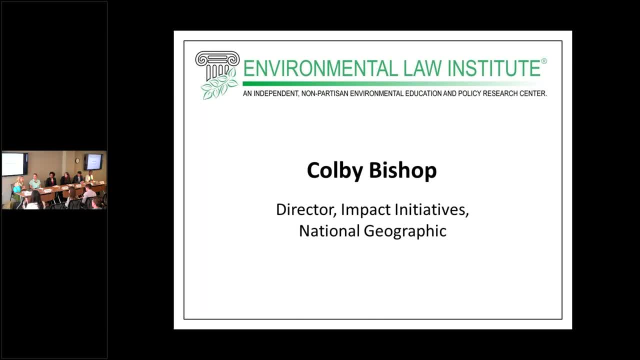 Rand Corporation. Rand is a think tank. It's over in Pentagon City in Arlington, Virginia. I was an admin assistant to some of the researchers. It was a great first job. In college I actually didn't have an internship like all of you smart people. I was a waitress at a local winery and it was lots of fun And 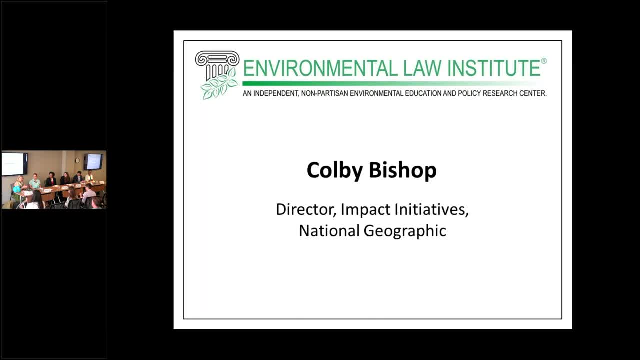 actually, I would recommend, if any of you have a chance to ever wait- tables. it gives you a great base in learning how to talk to people, learning how to deal with issues You know the same thing as working with a scientist and something goes wrong. is you know if somebody? 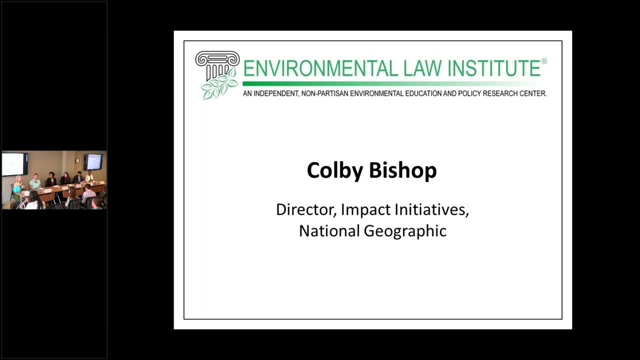 got like a steak. that's way too rare or something. You can fix that problem usually a little bit faster, But it was still a pretty valuable experience and I think I still use those people skills. Everything I do is talking to people or working with partners. I think I still use those skills today. 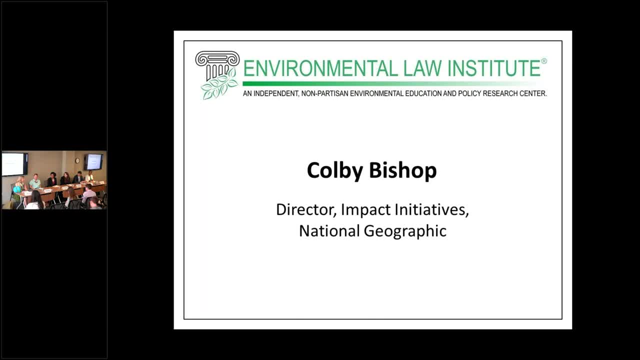 So anyway, I got a job at Rand once I moved to DC. I worked there for about a year as an admin assistant to five of the researchers. It was a great first job. I learned like what it is like to be in an office. 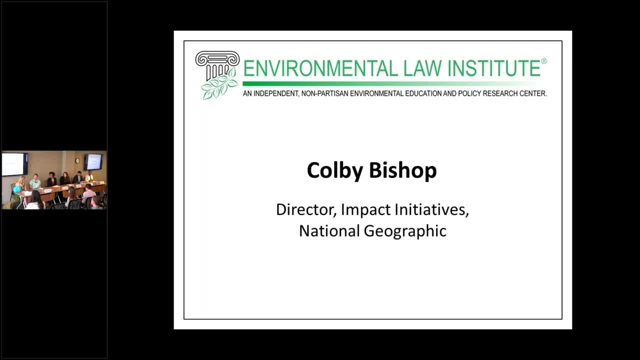 how to write an email, how to format a document, all of those important tasks that you have to do, regardless of what level you are in an organization. If I wanted to stay on and get my PhD and be kind of in academia, that would have been a great place to stay and grow, But I decided. 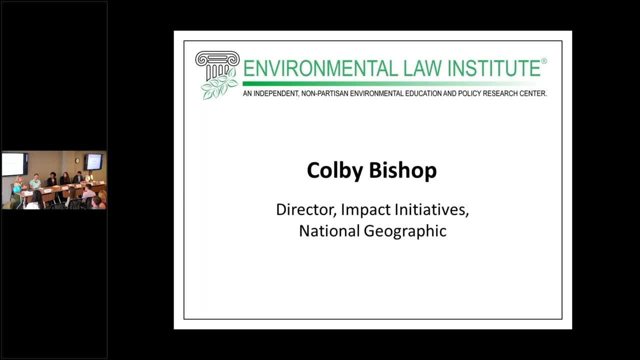 I wanted to do more. you know more, maybe program project-related things- And all of a sudden I found out through my trusty little globe that National Geographic was actually based in DC. So I started looking at jobs there and I got a job as the coordinator of the Genographic project. 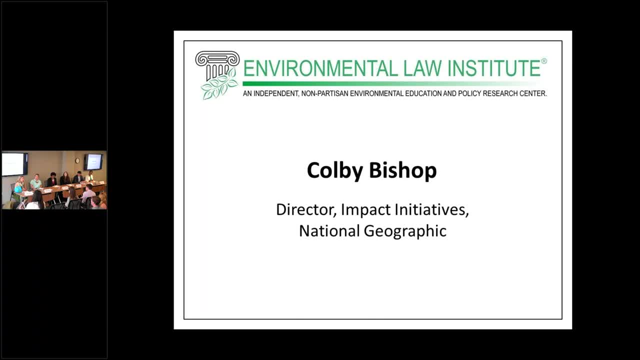 So this was about 11 years ago now. The Genographic project was a – is it continues today – is a – basically we were tracing human ancient ancestry. You guys have probably heard of like ancestrycom and 23andMe and all of those. We were actually the first to have a consumer. 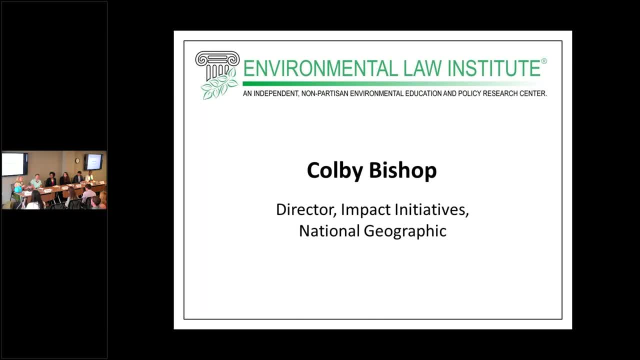 genetic testing kit. So we sold these kits. but then we also had a research component to the project. We had 12 different research centers around the world working with indigenous populations to actually collect the data, because their DNA hadn't been mixed too much like all of ours. for 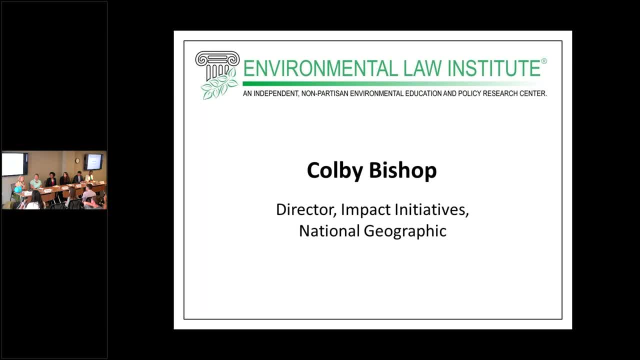 the most part. So those were. that's actually the science that helps drive a lot of these consumer genetic kits today. So I was the coordinator on that project. We had the 12 research centers and my job was just to keep them all happy, make sure they had everything they need. They had the money. 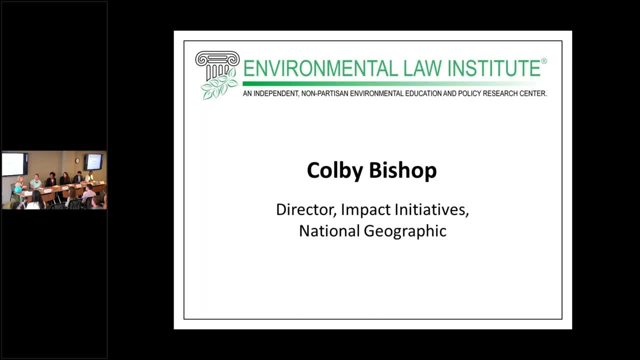 they needed the equipment they needed. We'd have annual conferences every year in glamorous places all over the world, So there was some fun travel involved. My first day on the job was in Shanghai, actually, which was fantastic. I'd never been to China before, So that was a fun, a fun perk. 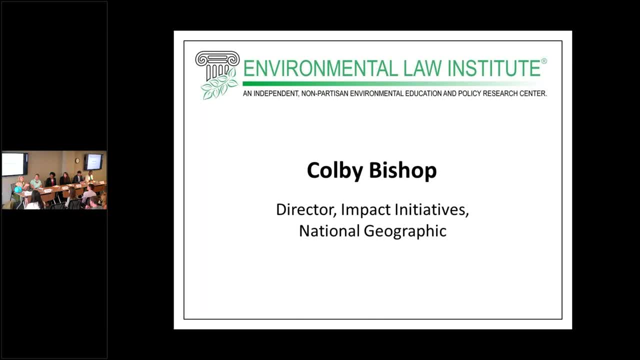 And since then kind of my role expanded. I got interested in working more on the marketing and communication side. So I did a lot of that for the genographic research center And then I did a lot of that for the project. Some additional programs started popping up as my boss's job kind of expanded to manage. 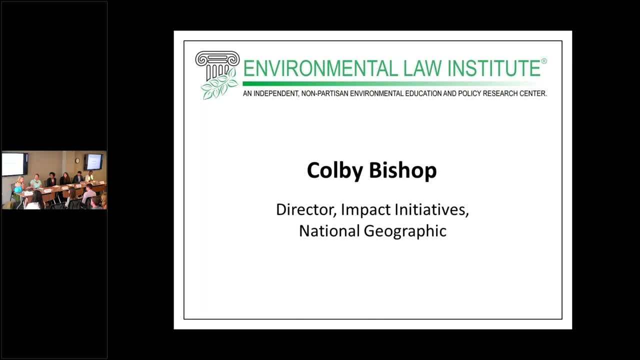 these large scale programs. Then I started working on others as well And as I kind of started to think about, what do you want to do when you grow up? And if you ask me that question now, like I probably wouldn't be able to tell you the answer because I think it changes, But I really liked my 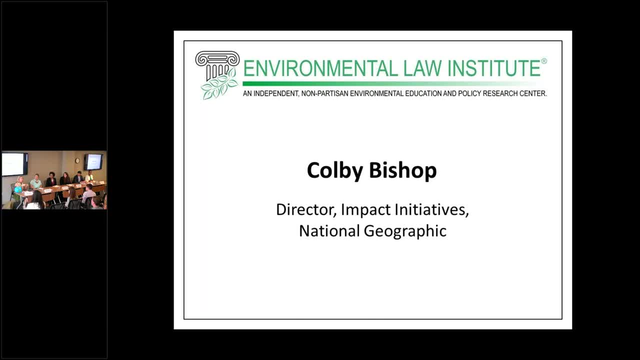 boss's job like overseeing these large scale programs with multimillion dollar projects And having clear outcomes that you are, you know you are at you're tasked with to achieve by X date. So I decided my background at going to liberal arts school. I didn't have much of the business. 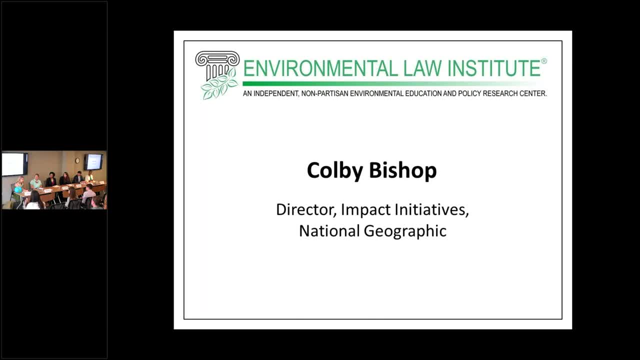 like accounting, those kinds of classes. So I decided to go back to school part time. I went to the University of Maryland and got my MBA. It was part time, So I continued working in my role at Nat Geo and was going to school. 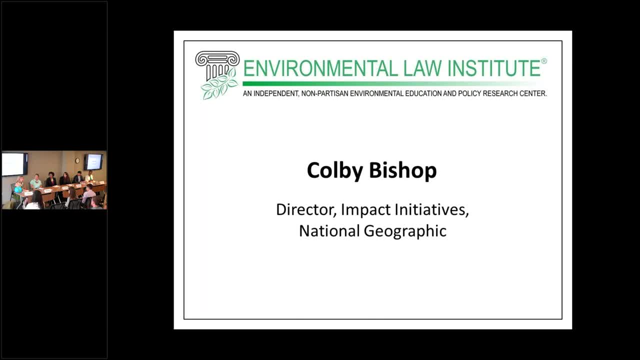 like night school. it was a three year program which is like it's a lot of work, but you just do it, You know, and my life like didn't end, I still have social life. So I did that And it ended up. 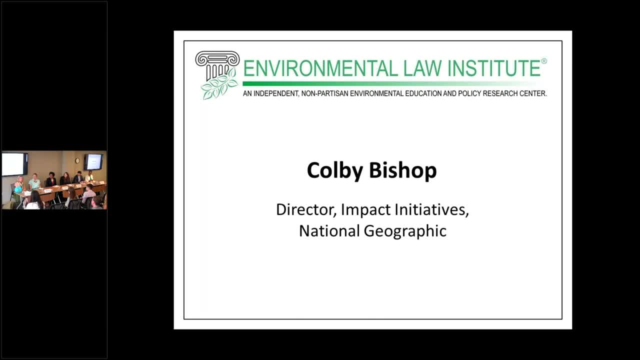 being great. One of the perks of going part time is that you still have a job when you're done with school, So that's great. You don't have that pressure. But also all the people that you go to school with. they all stayed in DC because they all also had jobs and a life here and all of that. 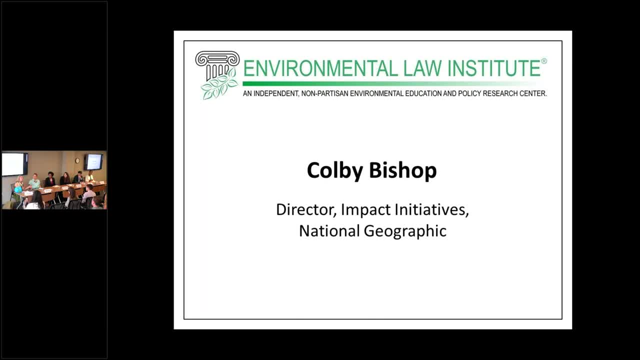 So now I have this new network across DC, working in all different disciplines, And so that's been a big benefit as well, And I think that's been a big benefit for me, And I think that's been a big benefit for me. So after school, after I finished my MBA, my role did expand across programs At that same time. 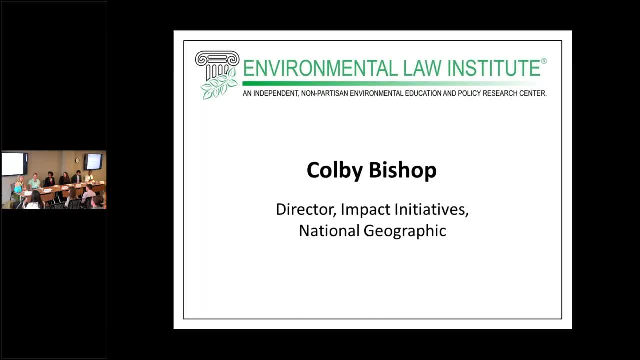 there were quite a few changes at National Geographic And we so, for example, we are now. it was one big organization when I started And now we're two separate organizations. we have a nonprofit side- And that's where I sit, And it's like impact oriented side, And then we 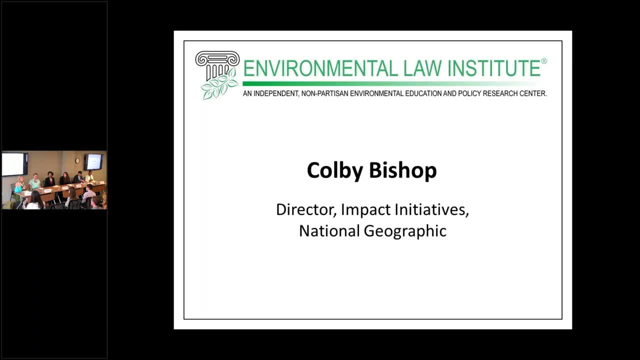 have a full profit side And that's like where the magazine is, the channel, probably a lot of what you guys are familiar with, the Instagram account. all of that's on the full profit side. We're all under one roof, but it's kind of an interesting setup. But it allows us as a nonprofit. 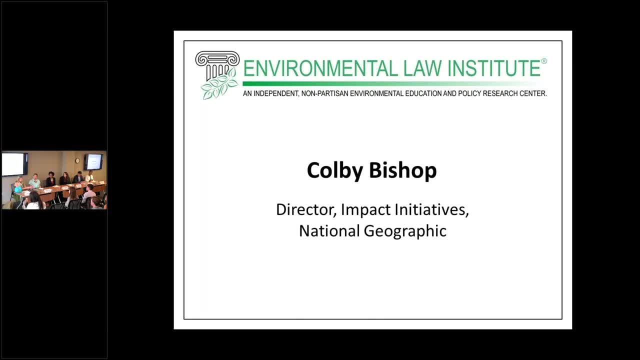 to really focus on on the mission and on the impact side, instead of magazine sales. So all of a sudden, the work that I was doing on this program side became what was most important to our executive and our CEO, which timed pretty well as I finished my MBA. So I all of a sudden became in charge of 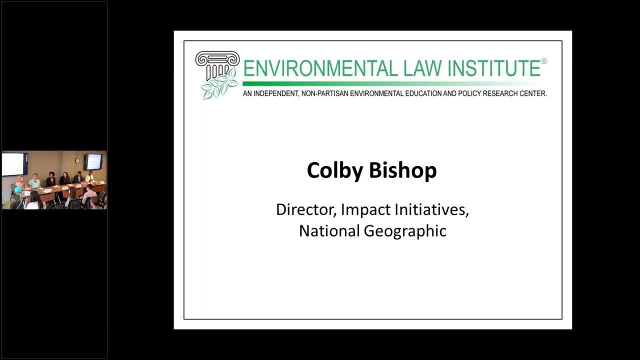 all of the wildlife programs. As in this role I mentioned, managing budgets is a big thing. I don't know if any of you have heard of logic models, But basically it's like a project strategy document, as you're creating a program so that you make sure all the activities that you're working on lead to what you're trying. 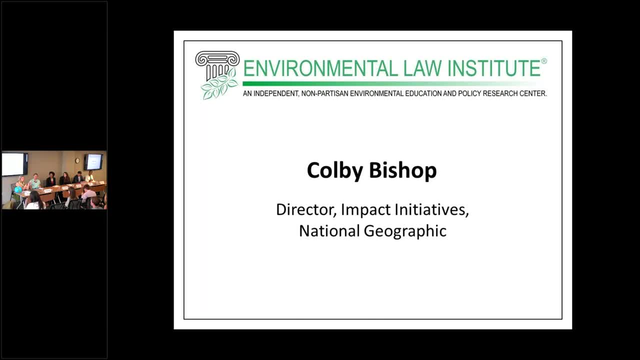 to achieve, because it's really easy to get distracted and say, Oh, like I want a globe because they're cool, But actually, is this globe can help me save big caps? maybe, But you have to make sure that you have a clear pathway. 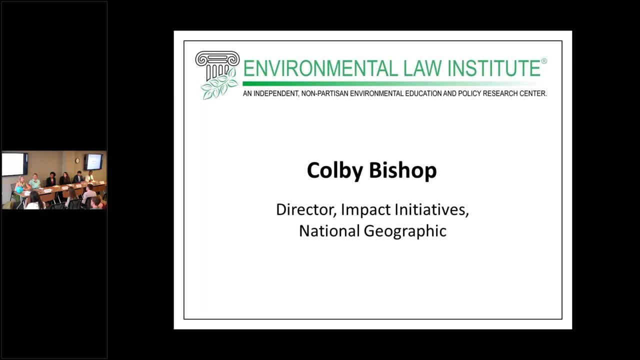 So that's kind of how that's going to happen. I have a full, I have a team of people. we're a matrixed organization, So I there's some people that do report into me, but others that have like dotted lines, because the marketing team, for example, has responsibilities on some of these product. 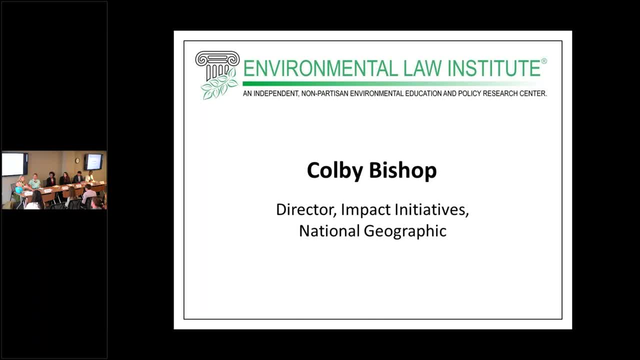 projects. So they have a budget line in my budget and they're responsible for spending it, But in the end I'm the one who's responsible for the full project. So it can be a little bit challenging managing those relationships, But it's just kind of the beast of National Geographic and how we're 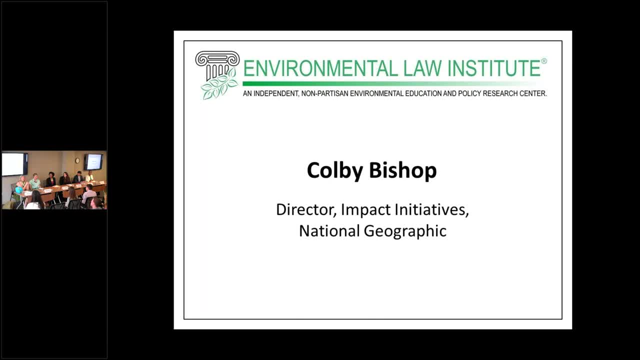 able to keep up some of the projects that I manage, So I have. you may have seen there's some posters outside. This project is called the National Geographic photo arc. Joel Sartori is a photographer with National Geographic. He's been a photographer for the magazine for like 30 to 40 years along one. 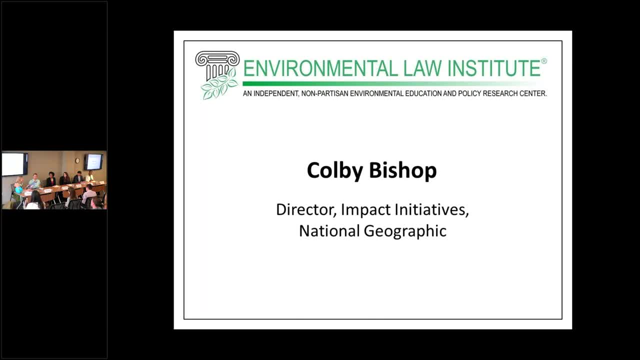 of our. he's been around for a while. He started taking pictures of all species in captivity And he puts them against a wall, And then he puts them against a wall, And then he puts them against a wall, And he puts them against a wall, And then he puts them against a wall, And then he puts them against a wall, And. 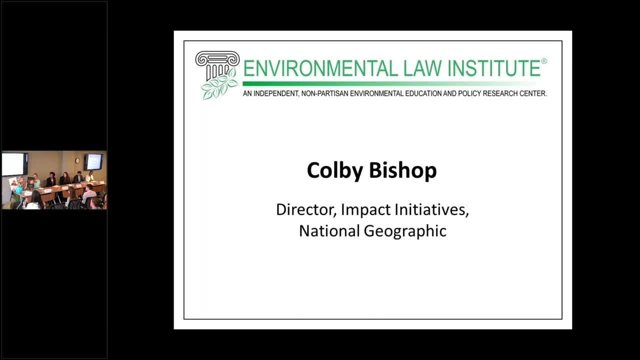 he puts them against a wall, And then he puts them against a wall, And he puts them against a wall And white or black background, just like this, tries to capture the eyes of the animal, And the idea is that a lot of people haven't seen these animals in real life. And, yes, you could go to a zoo and see. 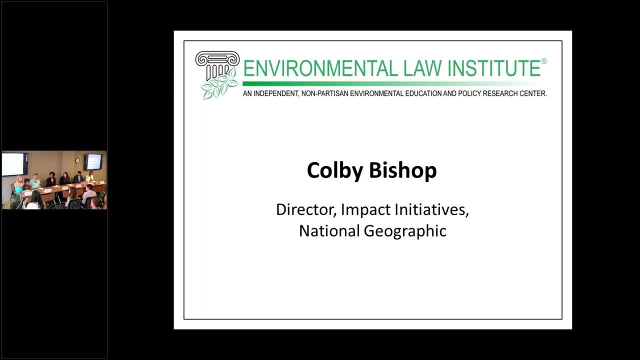 them. But some people don't even have that opportunity. So we're trying to market biodiversity, market wildlife for people so they understand them, get to know them. He captures the eyes so that you might care. Sometimes they have expressions that like a human might make. So the idea is that. 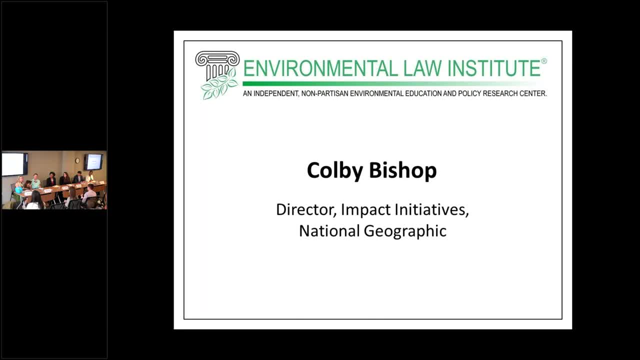 you captivate people in this way, get them to care and then change their behavior to actually save. lot of these big wildlife programs that we have have the science and research component but then also a marketing kind of public engagement side. so this is the public engagement side, the photos to captivate people. he had a TV show. 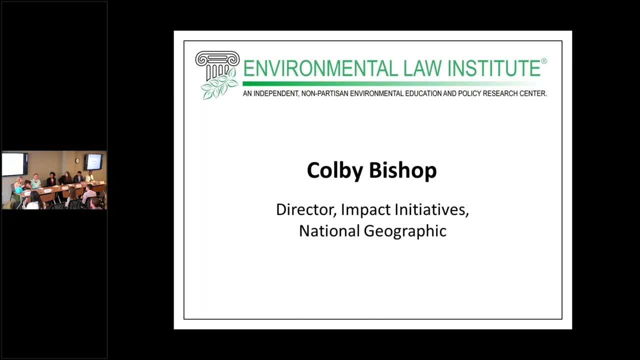 actually last year on PBS, we had a big billboard campaign across the US and actually that's what these posters are from. there's still some bus shelter stops around DC that have this, so keep your eye out. but it was. it was a campaign from last summer, so a lot of them have changed over, but then we also 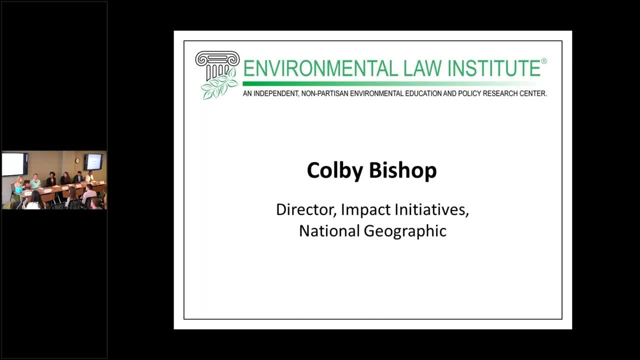 give grants to species. it's a conservationist working on species in the photo arc that are at risk of extinction, that might be lesser known, so maybe you've never heard of them before, but like the pangolin, for example, it's like this scaly armadillo like animal that is highly trafficked illegally. so 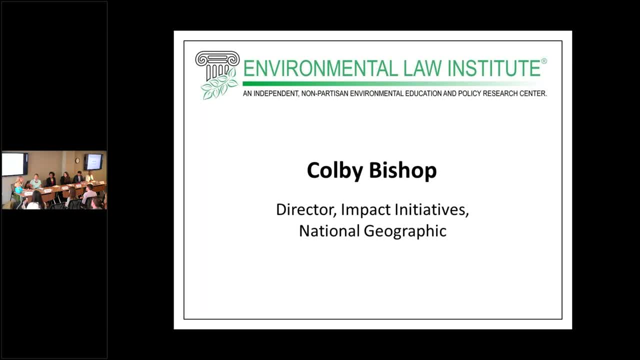 by investing and giving conservation grants to the pangolin. we have the photo, we can bring it to the forefront, you get people to care. so it's the combination of the science and the public engagement that brings a lot of these programs together. in terms of challenges, I think probably the biggest challenge with National Geographic right. 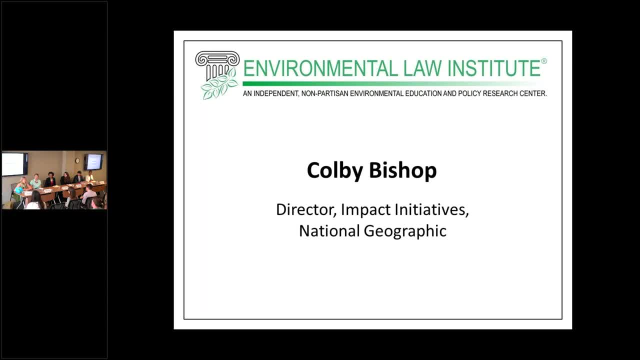 now is change, and I've. I think. for me it keeps things interesting and I think that's a key. a key thing is be open to change, because things will change. don't get too comfortable in your role, because you never know what could happen. right now we are looking for a new CEO and so hopefully, once we get our new CEO, 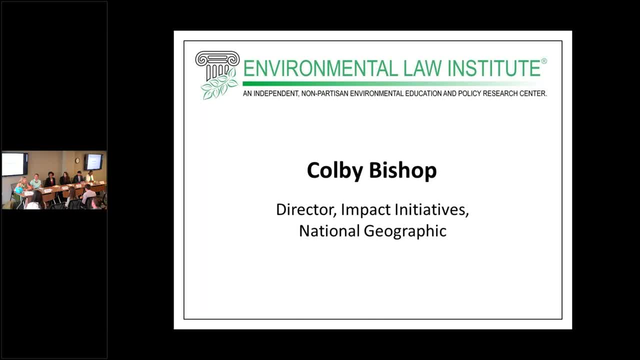 on board we'll have. we'll feel like things are a little more stable. but ever since we've kind of separated into two organizations, things have just we're trying figure out who we are and what we want to do. it isn't exciting place to work because I think probably the biggest perk of working there is the 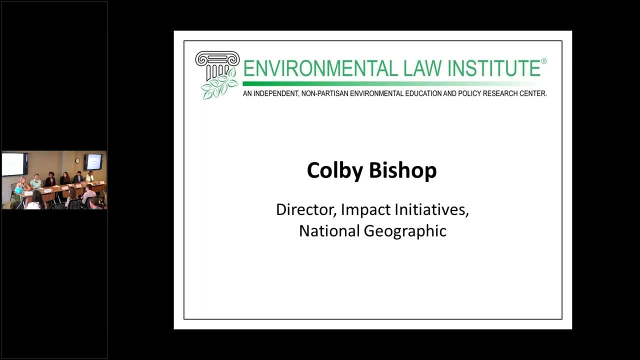 people. everyone has different backgrounds, different interests. they've traveled all over the place. I actually I'm going to Indonesia for a few weeks in a few weeks and there's three people on staff that have spent like years there and so I'm grabbing coffee with all of them to say, okay, I have like four. 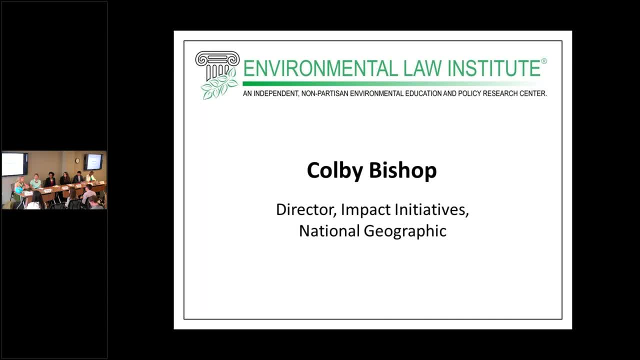 extra days. what should I do, you know? and they all have really they'll contacts there and they can just set you up. so everyone is it's just like a great place to work. everyone is there for the mission, so the people are great. in terms of environmental policy and law, I would say because we are. we are a neutral. 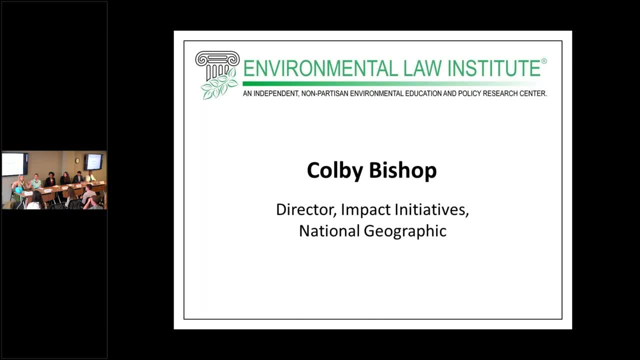 brand National Geographic. a lot of people want to work with us and we can get people to all come and play in the sandbox that maybe we're working on the same thing before and maybe even conflicting with each other's efforts, but we can, being neutral, we can get people to come together. so the biggest 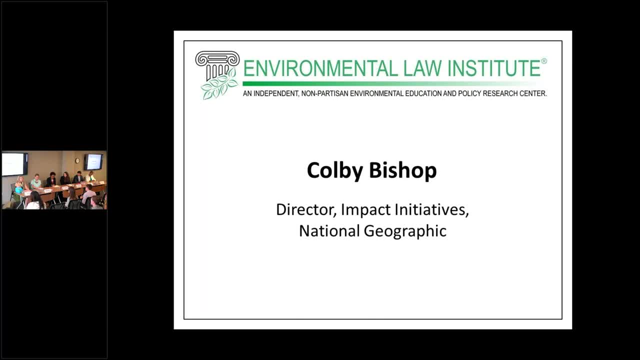 thing is, partnerships work constantly. I'm constantly working with our legal team to draft up legal documents to get these people together. a lot of these projects are international conservation projects, so we're working with governments and talking about their environmental policy- one project, for example, that I'm working. 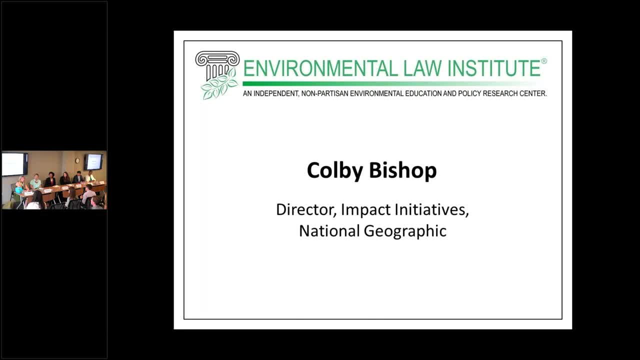 on now has to do with the Sumatran Rhino. there's about less than a hundred left and left in Indonesia right now, but the government of Indonesia technically owns all of their wildlife. so in order to do anything we have to work really closely with the government and make sure I'm following all of their environmental 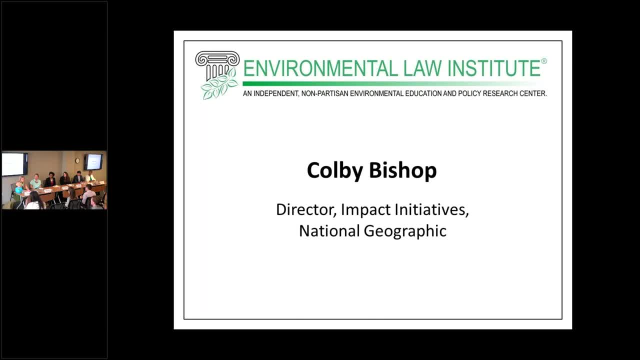 laws, know their conservation laws. so that's that's definitely where I'm working on our legal team. I'm working very closely with them to get these agreements signed with the government, making sure that we're following all of their policies specifically. so that's a quick overview of what I what I do and 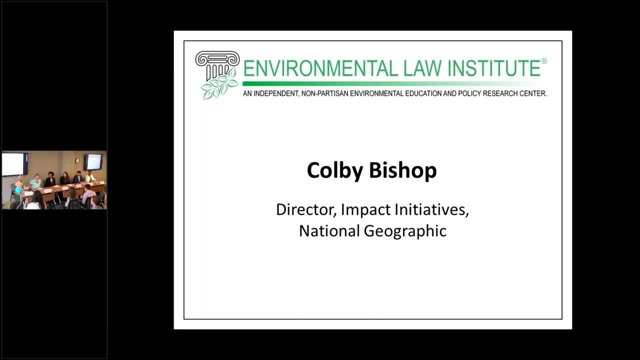 will take questions later. thanks, you're really cool. I'm Margo Pano duvert. I'm the external relations manager at Meng trade America. have you guys heard of their trade? yes, a little bit噴. So we're a global certification for mostly food, but also some textiles and mining. 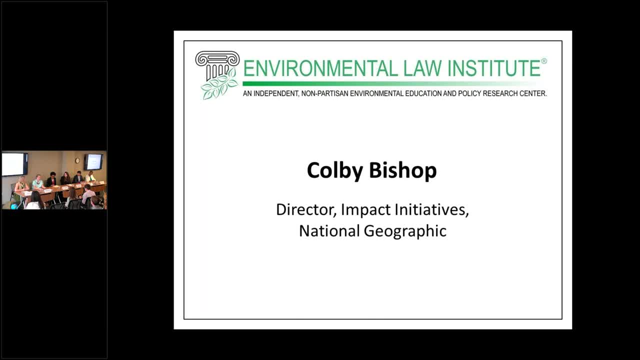 And we work with brands to help certify their supply chains to make sure that, from the farm or the mine or the factory where anything you're purchasing comes from, everything that's happening is as it should be. So I have a really fun job as the external relations manager of our US office, one of 32 offices around the world, and working with about 1.7 million farmers and workers globally to help them get their needs met in their jobs and also make sure that the practices of the corporations and businesses we're working with are respecting the environment as well as the people that work in their supply chains. 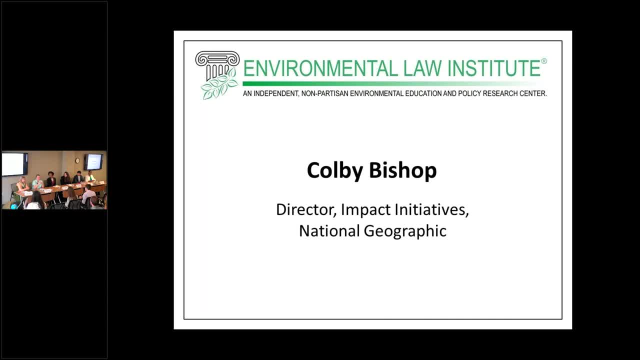 So that sounds all very business-speaky, but I promise I'm a down-to-earth, normal person. My education path was a bit winding and we were talking earlier about this, about how sometimes when you're thinking in these career panels, it seems like everybody's life is like do-do-do and then it's a very straightforward path. but it's not true at all. 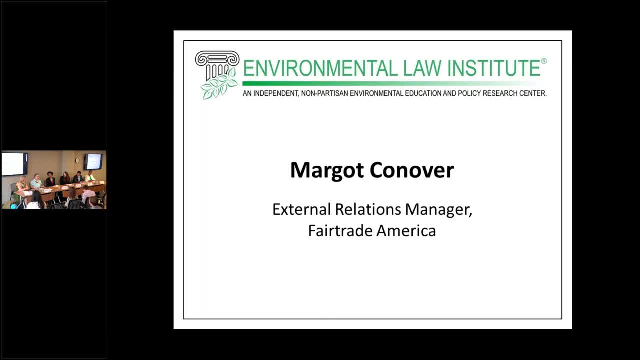 So how I came to be in this role and following this career path was somewhat by accident. so I kind of realized a little bit too late in my undergraduate education at Christopher Newport University in Virginia, which is also a small liberal arts school, that I was interested in agriculture after having pursued political science and Spanish. and it wasn't until my senior year, as I was writing for the US office, that I realized that I was interested in agriculture. 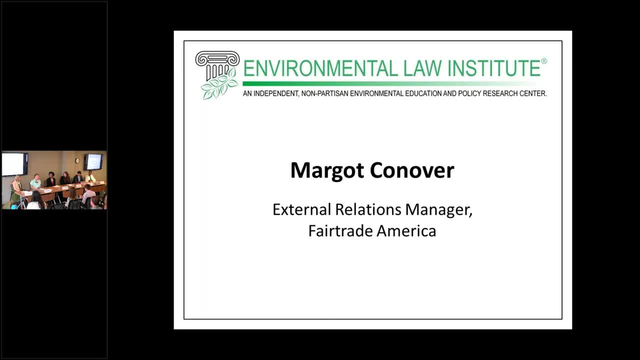 And it was during my BA thesis that I realized that a lot of the things that I was really interested in, like development policy and how US foreign policy is engaging in Latin America in particular, has a lot of agriculture implications, especially for sustainability. 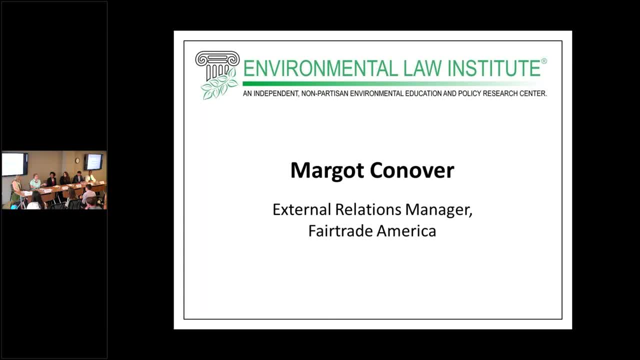 So by that time also, I had the exciting fortune to graduate right in the middle of the recession. so I thought, wow, I'm probably not going to get it. I should go to grad school and give myself a little space to think and wait until things even back out. 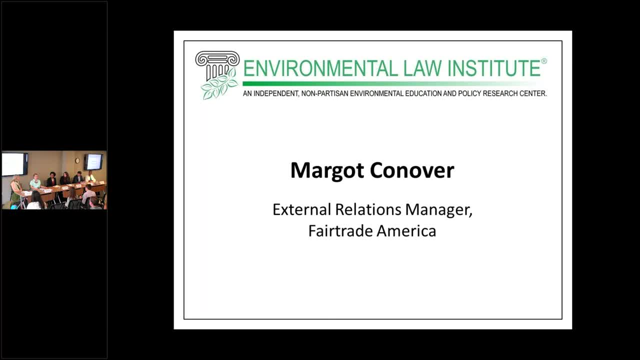 So I went to the University of Chicago to study international relations and talking about meandering paths, I honestly don't know why they admitted me to this program. not for a lack of merit on my part, but because everyone else in my program was like NATO war, great power politics, and I was like I like farms. 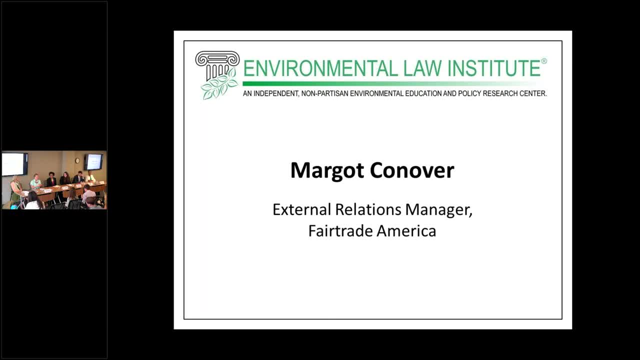 It was a really interesting experience to work with a lot of people that were just on a totally different wavelength from me, but to find a space within that where I was also getting my needs met. And at that time, because US Chicago is very well known for economics, I also found the only non-Miltonian libertarian corner of the economics department in the form of my thesis advisor. 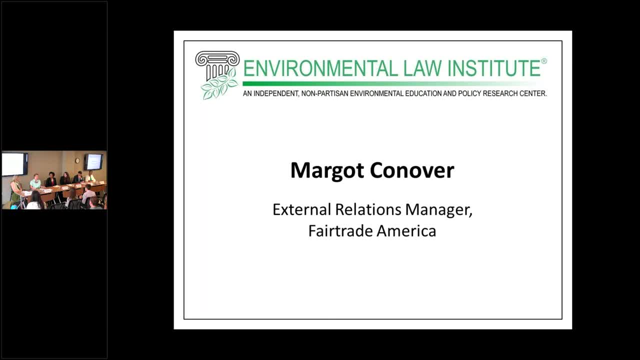 And with him I worked on a sustainability and agriculture and economics thesis that looked at acai. It's a palm fruit that comes from the Amazon estuary that had just recently been introduced in the US market for juice, So you guys may have seen it and, like Stambazon was the first brand that brought it to the US and I was like, wow, this is so cool. 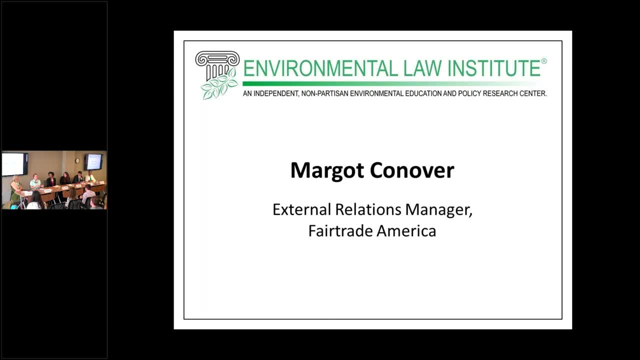 It's like business, It's environmental, It's sustainable development. working directly with these communities got a conservation component, So I found myself getting real excited about that. By the time I graduated from there, the recession was still going strong, and I also began to have nightmares about having to work in an office. 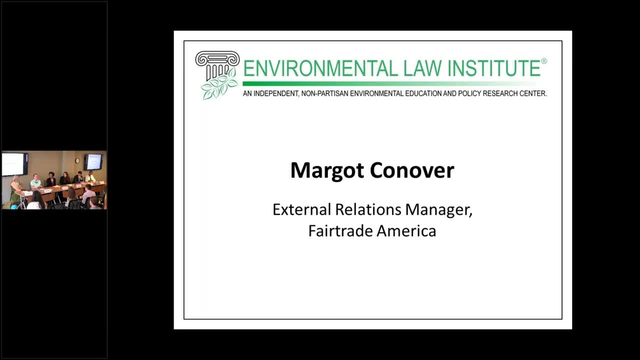 So I was like: why don't I just go somewhere and work in these environments that I'm so excited about? And a good friend of mine, Who's Ecuadorian, was like: oh, I know this guy through the Ministry of Agriculture down there that I used to work with. Do you want to come work for? my friend Carlos And I was like, yeah, great. So I ended up moving down there, sight unseen, to be broke somewhere else instead of in the States, and worked for two years with sugar cane, cacao, citrus and coffee co-ops. 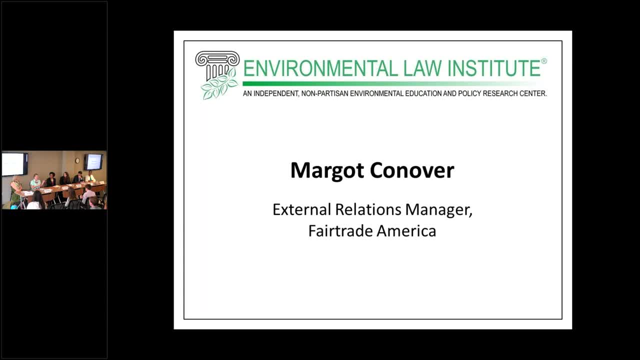 And that's, And that was just like a total detour. My parents lived out. They were like you're going to get murdered by drug lords And I was like it's not the 80s like you're up here. 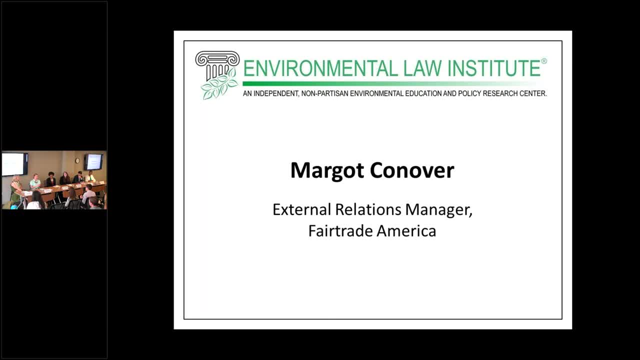 So I moved down there and ended up working in particular with the sugar cane co-op that was on the pathway to organic and fair trade certification and got to have a lot of really exciting opportunities to help the local community translate Some of these policies and regulations that businesses wanted to see implemented on the farms. 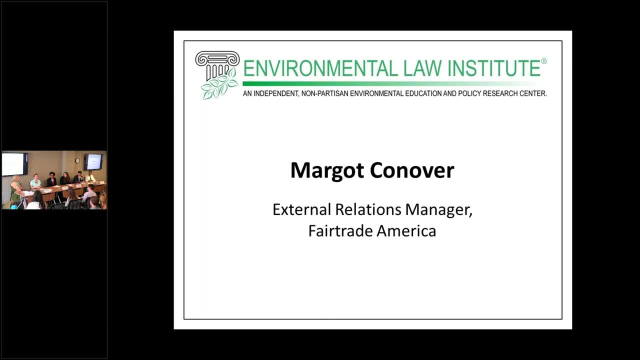 into a language and pathway that made sense for the local community. that wasn't just a bunch of white people in Switzerland writing a 200 page document that was like you're bad because you use child labor and burn your trash and like, instead of understanding the context in which this is taking place. and again it 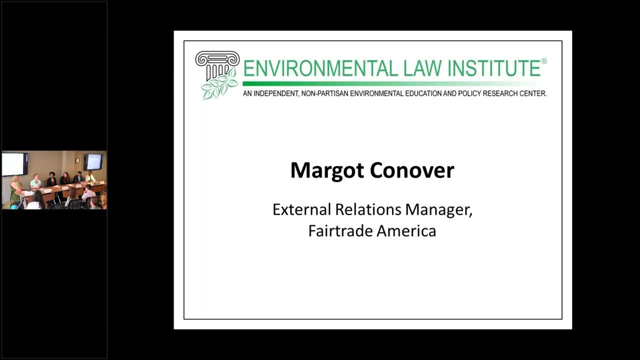 was just like taking advantage of an opportunity and saying yes and like being cool with being broke and dirty in South America instead of broke and clean at home. and there I found I really was extremely excited about and loved working in the field and on the agriculture side, but also got 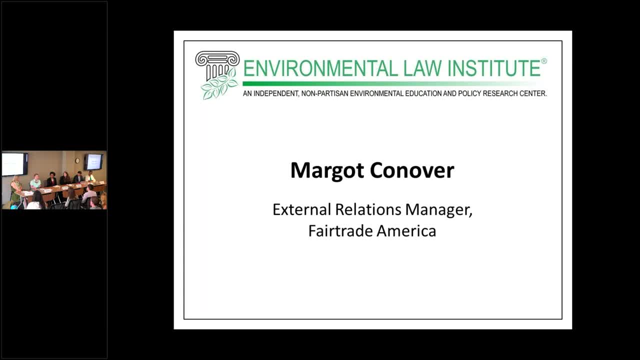 increasingly interested in the business side. I got to work with some pretty cool brands like Dr Bronner's and soap company, the body shop, a few coffee companies that are sourcing from down there, and really like loved being in this environment. but after two years of that I 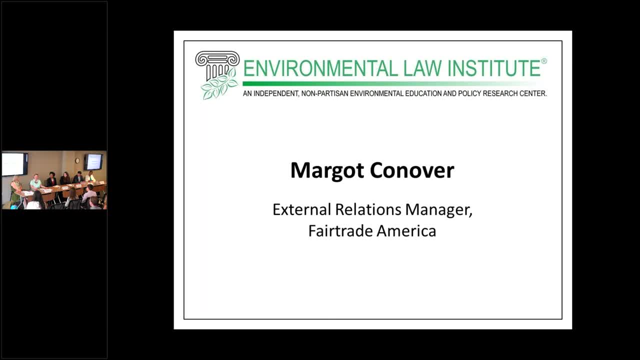 was like you know what sounds great: working in an office. it's so clean and relaxing. so I decided to move back to the States and ended up having a brief detour into public health, where I- because I, after having seen some of the health issues and the farmers that I was working with and how, 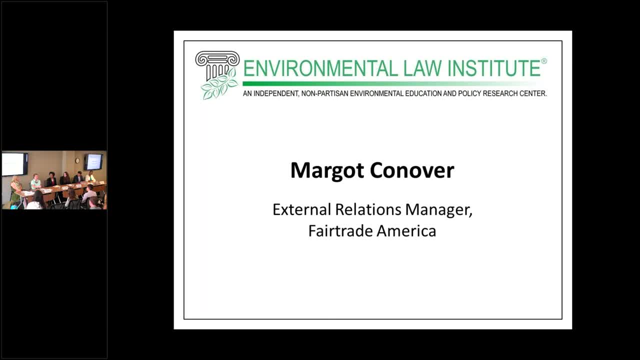 people don't really divide our lives into these little boxes and the way that a lot of development sometimes does, and I was like, yeah, I can, like I can offer a perspective there. but after a few years of that and writing grants and not loving working in an office as much as I fantasized about, I found I really want. 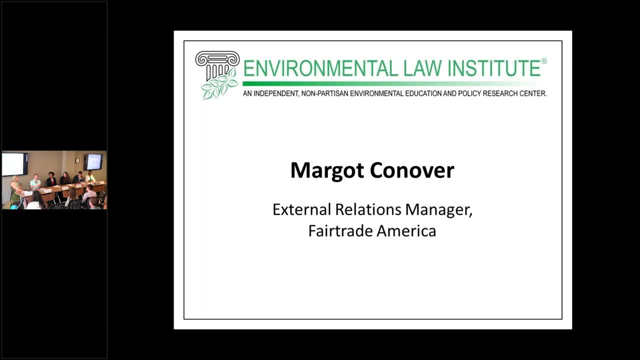 us to get back into that fair trade world, so I transitioned to Fairtrade America. I just finished my three-year mark a couple weeks ago, so that was exciting and I have really loved it since then. it's a great blend of caring about all of these different issues and it really 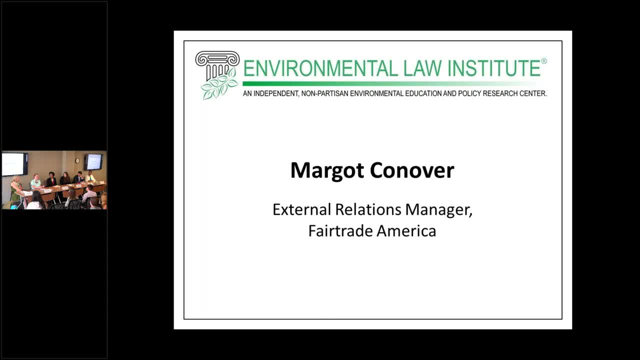 touches practically everything you can care about if the environment is your thing, but we have really strong work with our farmers about climate change adaptation. in Michigan I did a big project and a little bit of work in my litigation making sure that all the practices on the farm are really respectful of watersheds. 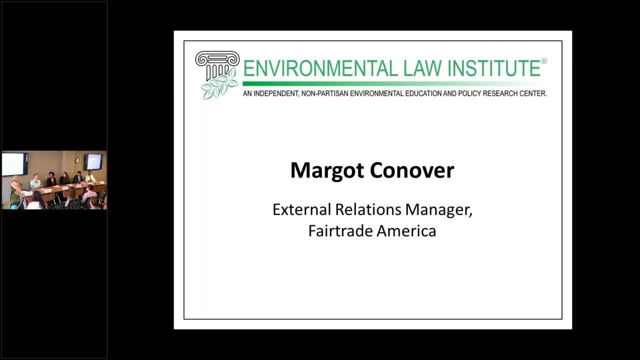 that we don't use GMOs, not because of an anti-science stance, but because of predatory behavior on the part of some of these ag companies towards small farmers. Or if you care about child labor, if you care about human rights, if you care about labor. 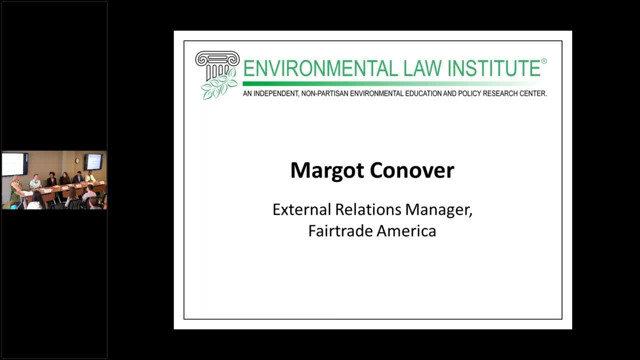 rights. there's something in it for everyone. So in my current role, I would say that is both what's really exciting and what's challenging, because it requires a lot of. you need to really be able to focus and bring clarity to these disparate issues. 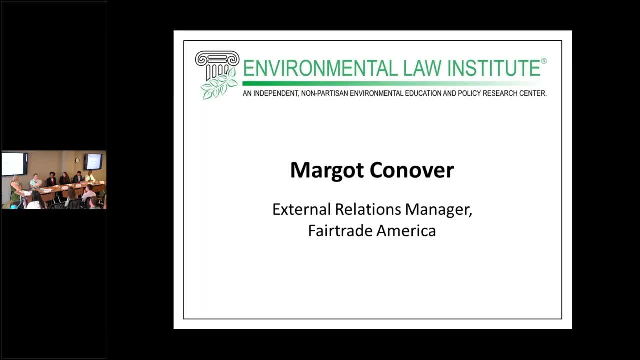 But I've really been able to do so much cool stuff. Like the way that I got connected with ELI was last fall because we were doing an outreach to promote some of our climate change work. So I was doing an event, A learning breakfast series, called Toast a Climate Advocate, where we brought fair trade. 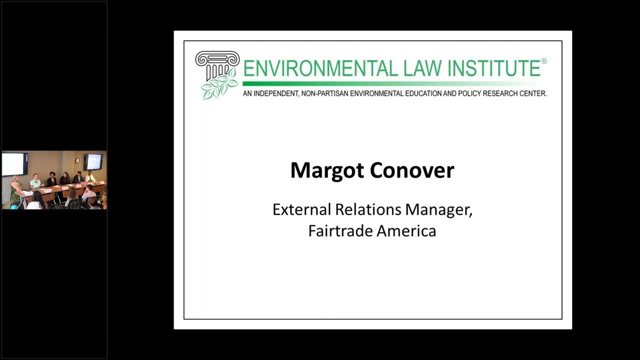 avocado, toast and coffee to all of these organizations that work on climate or environmental policy to be like high five guys and share some of our work about power engaging with the issue as well. I love being able to have that kind of creativity and autonomy about how to engage and share. 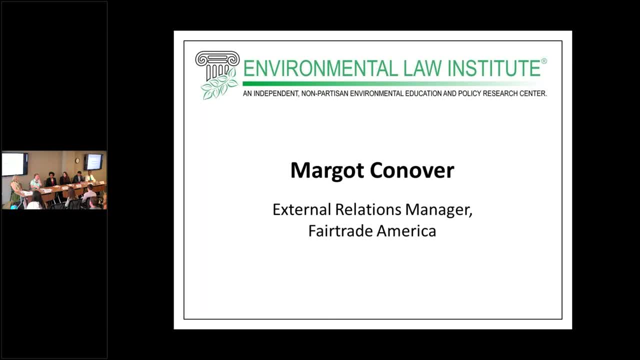 these issues, But it is really hard. It's really hard to choose because there's so many cool things to share and so many issues that are relevant And the importance I would say to environmental law and policy relates to my work is kind. 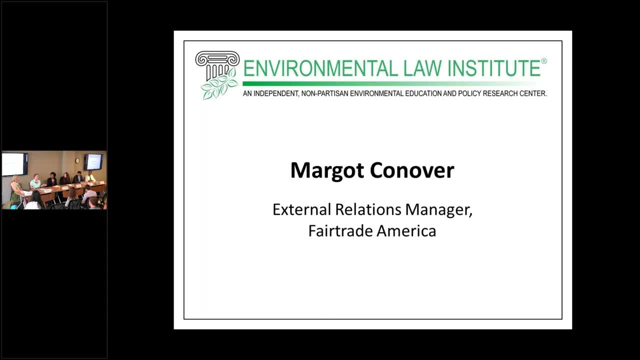 of encapsulated by this Wendell Berry quote that I really love. If you guys have never read it, I'm sure it's awesome That eating is an agricultural act, and it's one that we do three times a day at least. So if you're. 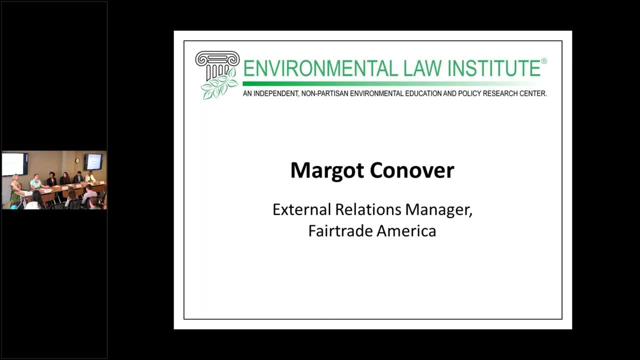 If you care about food and you want to eat in the future, then you really need to care about environmental policy In particular. it's a really interesting space for me to be in, because we do work a little bit with some government policy, but we're primarily focused on changing corporate policy. 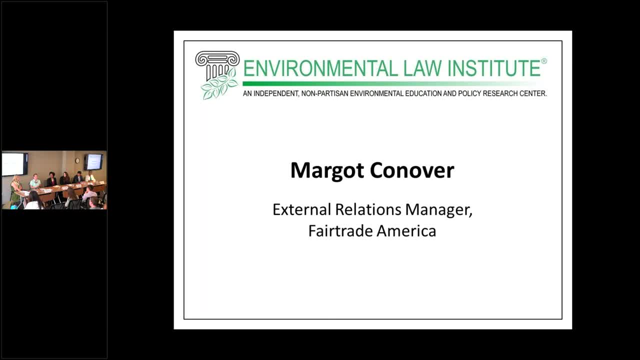 either directly through engaging with businesses or through the trade associations that they belong to. That can be super impactful, In the same way that changing a law is, because if Target changes some of their sourcing policies, it has such a huge impact and touches so many people all over the world that it also not. 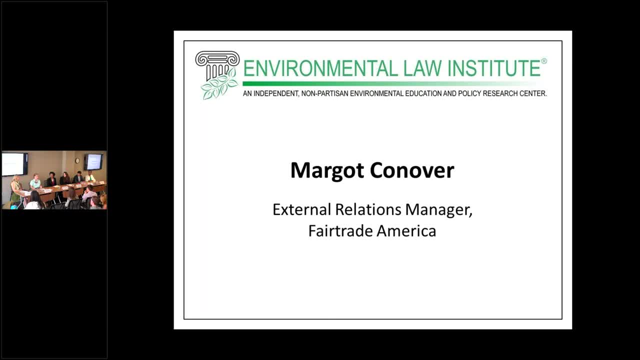 just changes Target's supply chain, but it makes it a lot easier for smaller businesses to jump on that bandwagon with them. So our goal is to empower businesses to not have to choose between making money and being good. We want them to be rewarded for being good and they should not be rewarded for being. 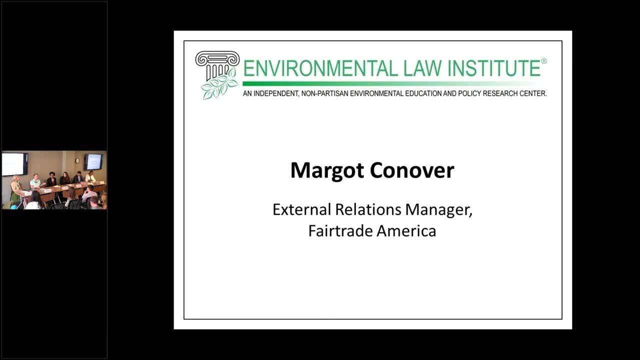 bad. So we help them to have the information and resources that they need to do that, as well as helping consumers like you guys to have the information and resources to hold the businesses accountable. And that's really exciting, not just because of In-N-Out itself, but it's also exciting. 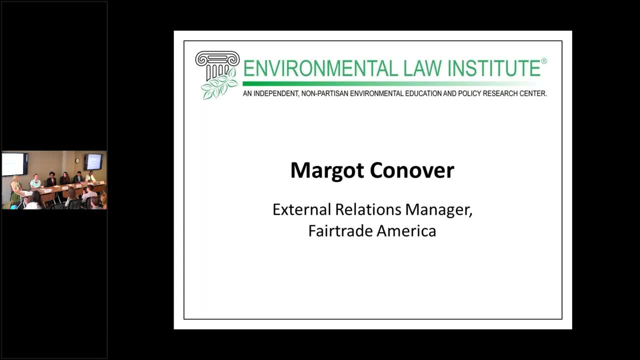 because it touches everyone. We all eat and we all have to wear clothes, and that's so exciting. So we're really excited about that. We're really excited about that. Thank you, Thank you, Thank you, guys. We would love to hear from you. 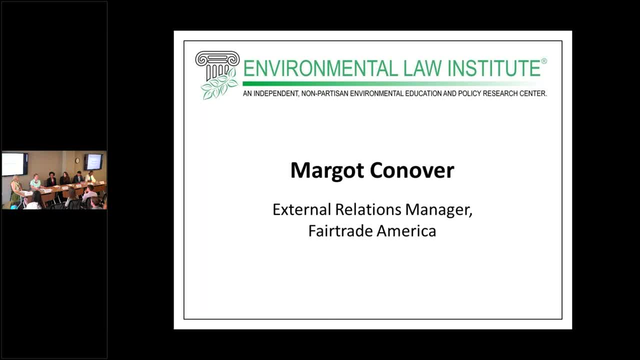 So fair trade has space in it for just about everyone, and sustainability is an issue. It's one of the few bipartisan issues, truly. Some of our strongest supporters are very right-wing libertarians and some are very lefty, so there's something to care about for everyone, and it's not kind of like with. 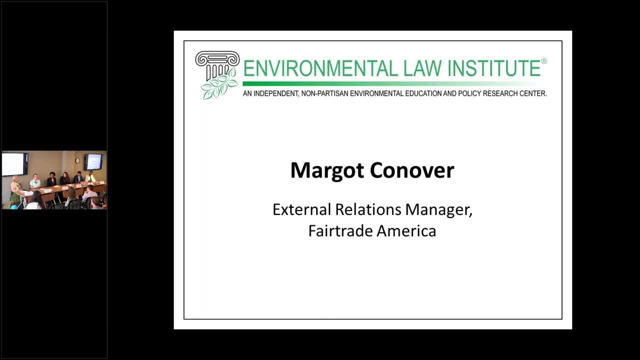 National Geographic. It's not closed off any of your other political views, because everybody loves food. so I would say, if you don't remember anything else, remember that that we all eat and so we all need to care about the environment because of that. so thank you, guys, I'm 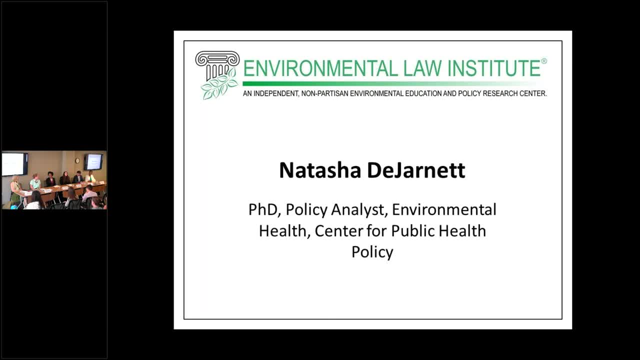 looking for your questions later. thank you, no pressure to follow. I'm Natasha D Jarnett and I'm from the American Public Health Association. we are the largest Association of Public Health Professionals worldwide. we have 50,000 member- regular members- and then we also have 50,000 affiliate members. that are, we have affiliates in each state and 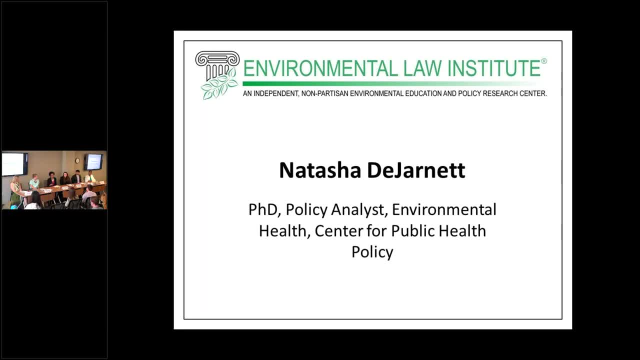 to New York, to in California, to um, and one in Puerto Rico as well, and I'll get more to APHA a little later and give some background on myself and then bridge those two stories together. so I went to Western Kentucky University for undergrad and everybody all my life said: 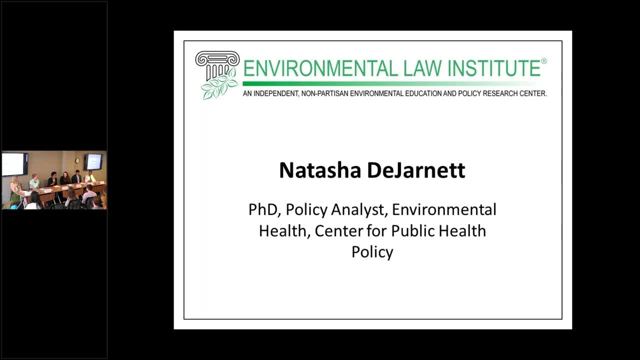 you're smart, you should be a doctor. well, not everybody. people said you care about people, you should be a doctor. and I said I do. I want to understand. where did I get my degree from? from wherever I graduated and everywhere I attended from, and I was told: you're smart or мы bad, If you want. 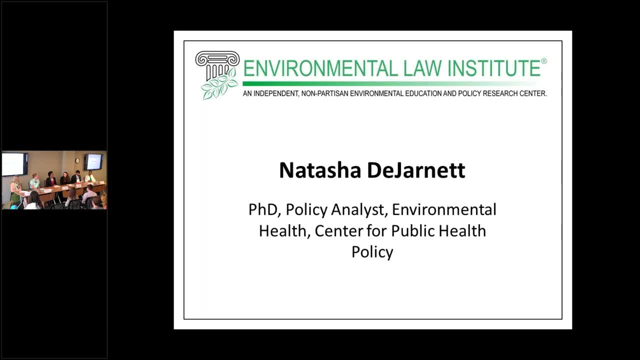 to protect people's health. I want to be a doctor, so I was pre-med and undergrad and I majored in biology and chemistry, because that's what you do when you're pre-med- at least that's what I was told at the time, and and I can't believe you- 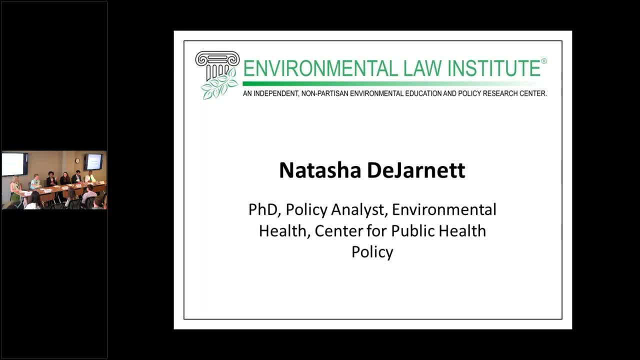 told at the time and- and I stop with that throughout- but about halfway through my undergraduate experience I began to feel a disconnect with medicine cat. I graduated and I said I don't think medicine is it for me. I don't know what to do with this, and spoke to my very wise mother. if you see her, tell her that. 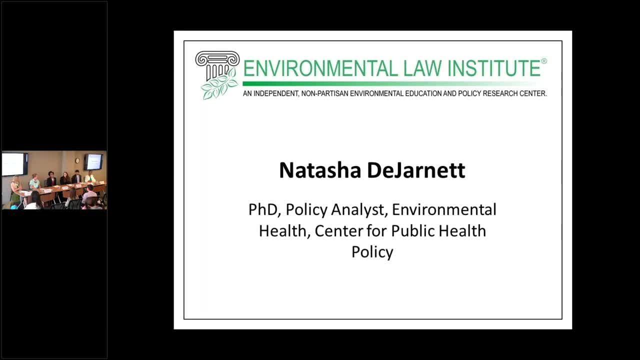 he said she was right. she said I said I don't know what to do, and she said: what about public health? and I said: oh, that sounds good. what's that? and she said I don't know, but she was right. instead of listening to her, however, I went and I 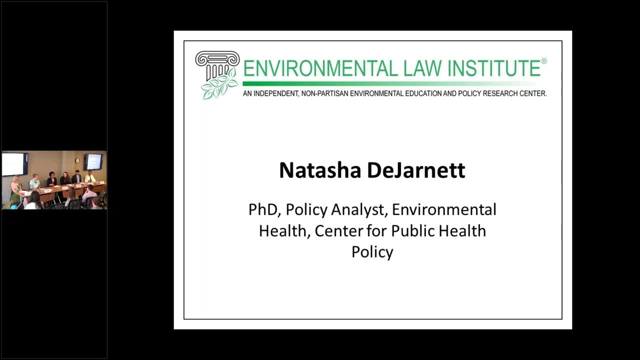 worked in industry for a few years and I did research and development. so I used those chemistry and biology degrees but I was committed to health. if my interview, don't know why they hired me, but I'm glad they did. but if I interview, they said: so what do you want to do with this? they manufactured printers and I 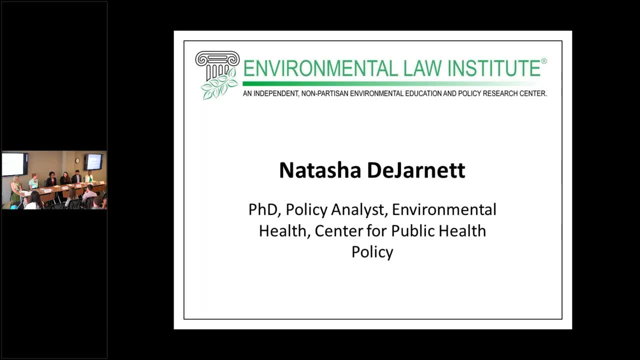 said I want to use printers to improve quality of life- and the interviewers pretty much. I think this may have been my first day, my first week there, when I got there- and this is not unusual for anyone that works in research- but my office was in a 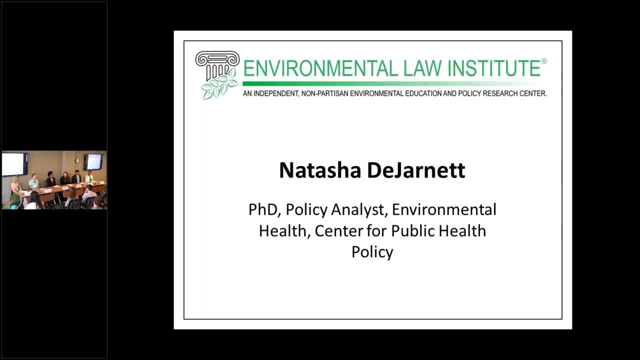 lab. now, this is my first job out of undergrad and I was like I I don't understand why my office isn't this laboratory. okay, we'll deal with it. then I became kind of hypersensitive to what was happening. it wasn't a lab that I use. 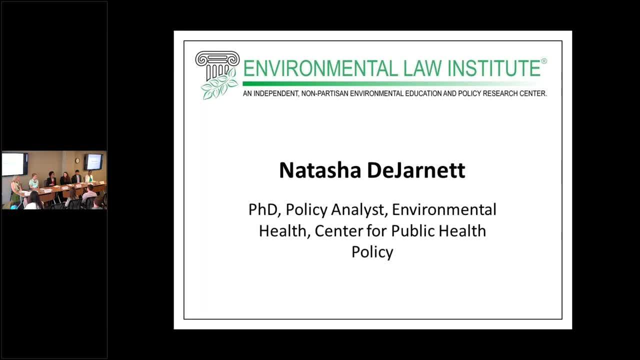 just happens to be where my office was. I use different laboratories and I would see people come in the lab and they may operate with a chemical, but not using the, the fume hood, and i'm like: what am i breathing, what am i exposed to? hypersensitive disclaimer. this company is environmentally great, um, but as a 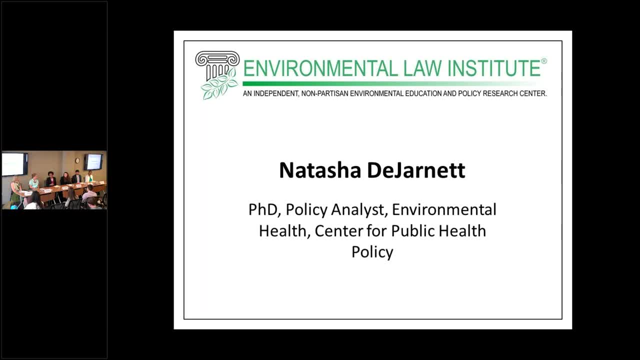 you know, new graduate um you're. you don't know what's going on, you get nervous. so i um started looking up these chemicals and some are teratogens, um reproductive um hazards, and then some are carcinogens. i just i said i i don't know how i feel about working in this lab and i'm doing. 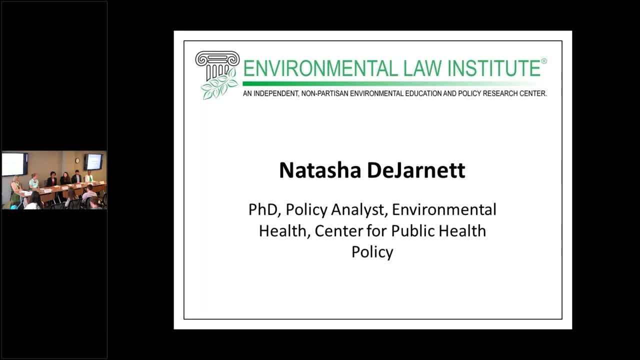 spreadsheets and people are using, uh, these things. so talked to my boss and he said: okay, i'm gonna move you to a regular office, which is what i wanted. i'm gonna move you to a regular office, but first i want you to do an air sampling experiment and i want you to report back out. 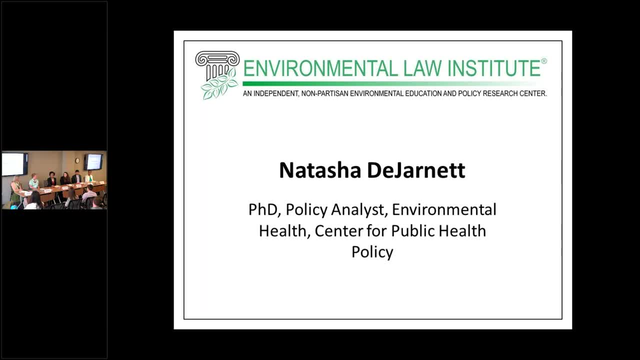 on your findings and you know if there is a big concern then we need to do something about it, and that was my introduction to environmental health. it didn't have a face and a name to me at the time, but through that i found that i was very concerned with the health of the workers and i was 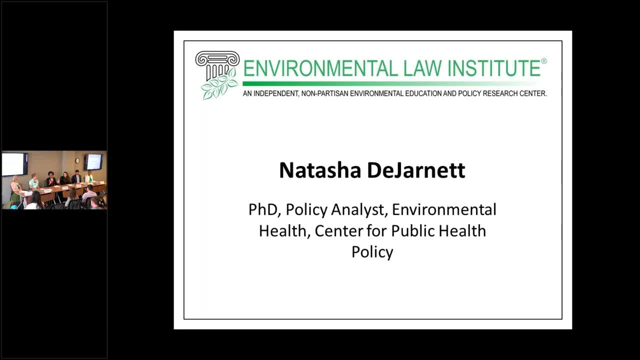 also very concerned with the health of the people on the fence lines of the industry. so, um, long story short, did the air sampling experiment? we were not in danger. the the levels were in like the parts per trillion range, stellar company, um. but i learned a lot in that um i i think what made it was a teachable experience for me and i'm i'm glad i got something. 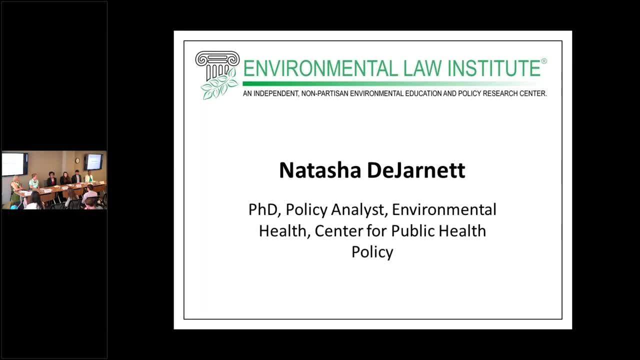 out of that, put that out the back of my mind, went on to work there for several years and, um, that itch for health just kept coming back to me. so i started volunteering so i could do, you know, fill that need and i, in my volunteering experience i met a woman with a phd in public health and then 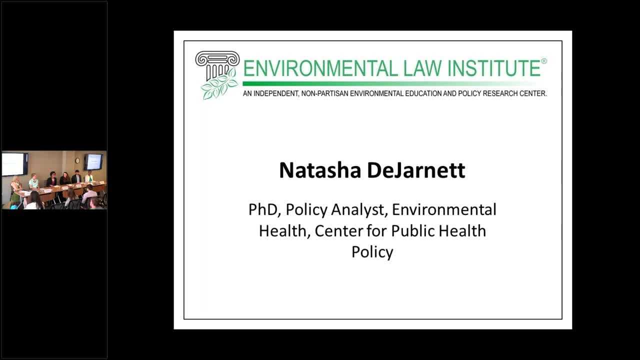 i remembered what my mom said. so i think it's a great experience for me to be able to do that, and so i did a google search and next thing i know, i was off to grad school at university of louisville, first public health class. i knew that was a fit for me. i said, oh, i wish i had found this sooner. 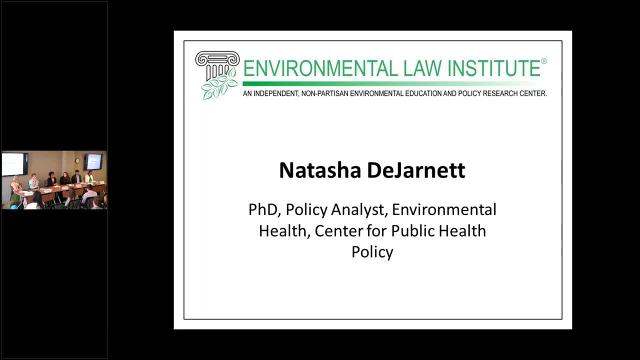 but i probably needed that time to appreciate it more and also have those experiences and research and touch on environmental health to really inform what i wanted to do. i didn't have my first environmental health class until my second semester but i was sold. i'm pretty jealous and i missed that last semester to make sense of what is going on. 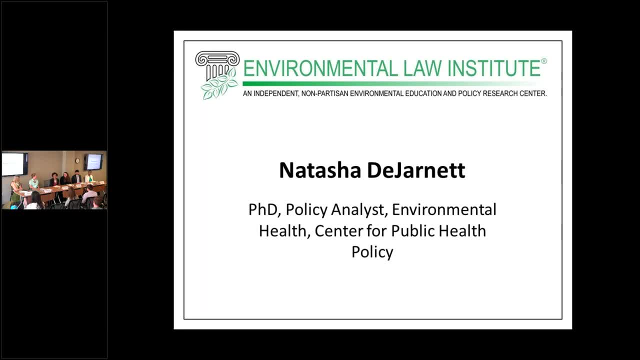 and you know, environmental it's not everybody's niche, and so some of my classmates would go in the class, fall asleep. and that's the one class i was like: tell me more, i've got questions for you. i didn't even need my little tricks to stay awake. candy didn't need that to get through those classes. 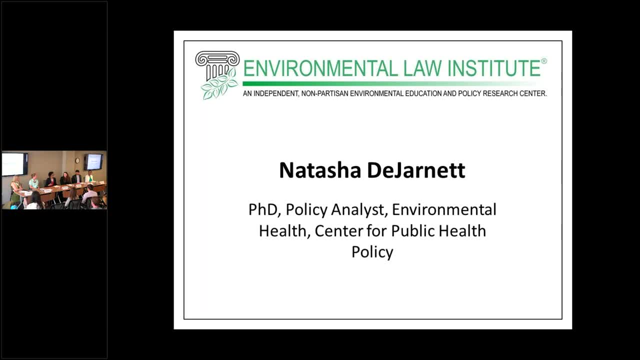 so, um, i loved it, but i was hesitant about it. um, i never grew up seeing myself as an environmentalist. i never saw myself as a tree hugger, that we breathe and the water that we drink. I was fearful that I would be going into a life. 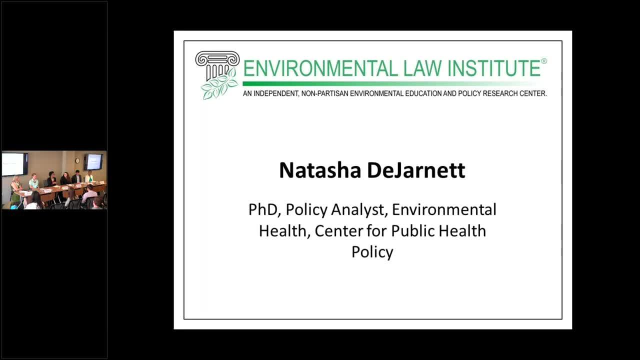 of bug collecting, which I'm terribly afraid of. It's important. We need that. I'm horrified of it. however, Once I realized that it was bigger than that, I said I think environmental health is a fit for me. So I come close to graduation and one of my professors- I won't give you the. 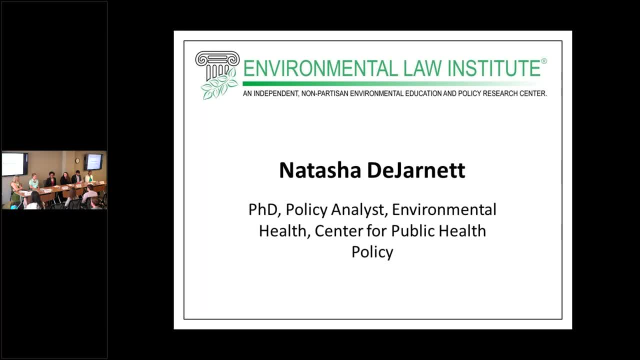 long story behind it, but they were very encouraging and somewhat of a strong arm said: you should really consider getting a PhD. I'd never been told that in my life, but I'd never thought of it And I'm glad that I listened and allowed my arm to be twisted. 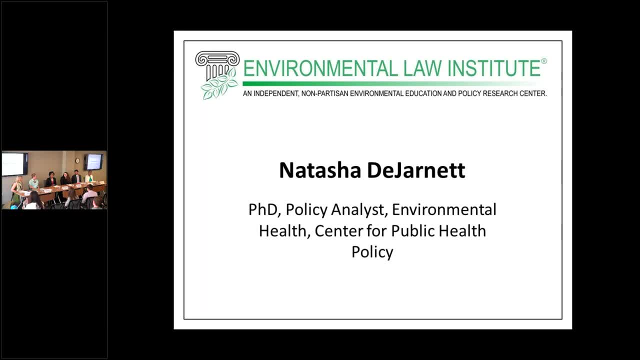 because it was a great fit. I stayed there and I went on to do my dissertation research around air pollution and heart disease, which was once again a perfect fit. I enjoyed that because the connections aren't obvious and overt. We can see air pollution and 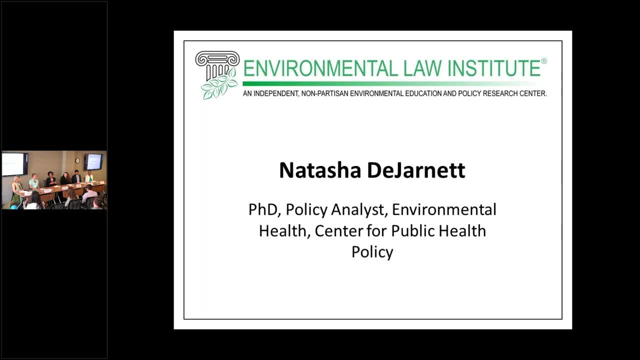 asthma and air pollution and COPD, things like that, But connecting it to heart disease. I love when I talk to people about it and you kind of see the light bulb go on over their heads. And so I did that. I stayed there for my PhD and then I also stayed there for my postdoctoral. 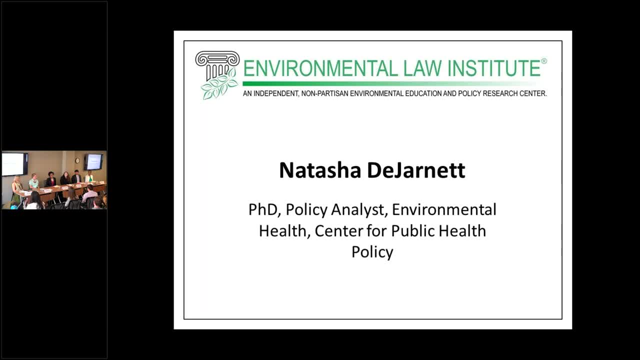 fellowship to get some of our research papers out the door, get some more experience. my project was mostly around environmental epidemiology. During the program, one of my professors picked up on my interest in policy. He's like: all right, are you really interested? 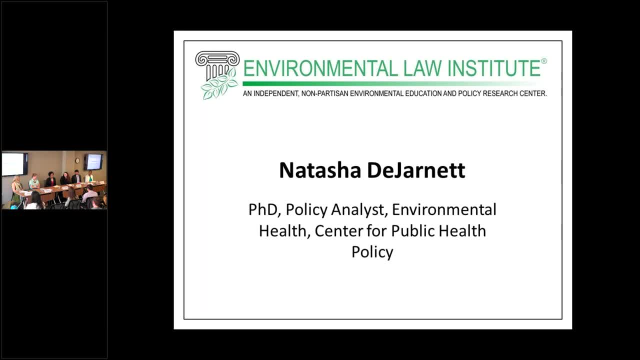 in doing lab bench research for the rest of your life, Or are you interested in something more like policy? And I was like policy, yes. And he said, well, maybe we can create a policy option for you, a policy route, because all the classes are for the PhD program, very biochemistry. 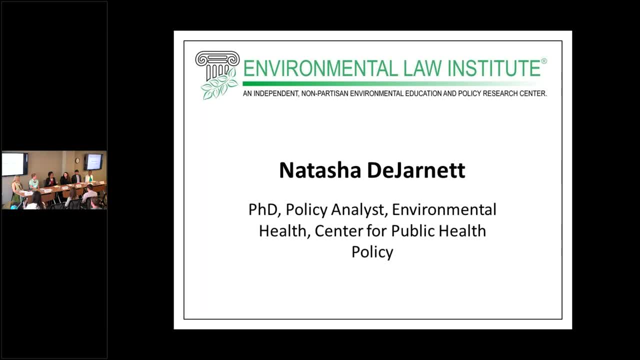 biobiology focused, And so I thought that was so exciting. There are classes at our law school that had environmental law, so I thought it was going to be great. It did not pass, did not go through. Our chair was insistent that if I want it to be an environmental policy, I would be best. 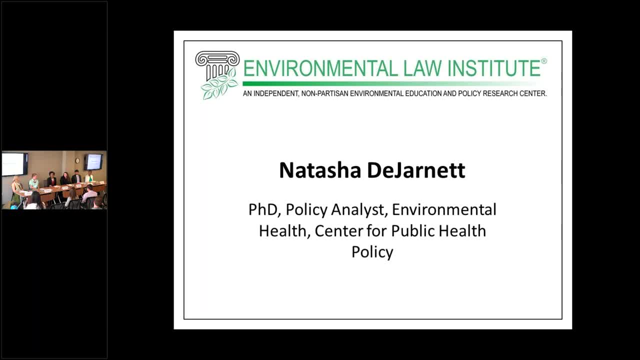 served if I understood the science that supported policy. That was tough. I already had the degrees of biology and chemistry so I didn't come in interested in furthering myself. I didn't come in interested in furthering myself in that direction But I think it has served me very well. I think 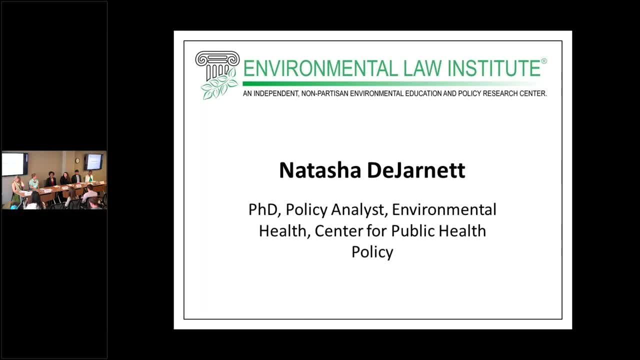 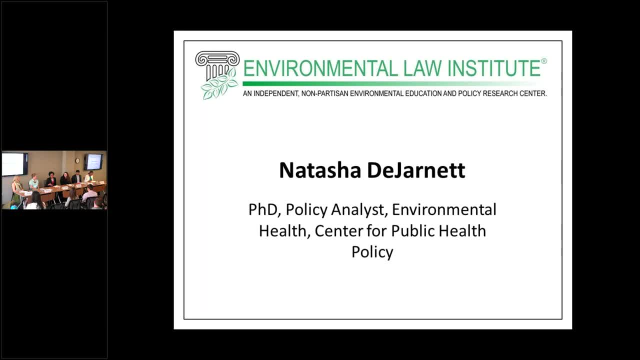 before I became staff, And it was a very, very long time before I became staff, And it was through my membership that I found out about the position. I was a part of the environment section and then I started to have leadership positions within the environment section And through one of those, 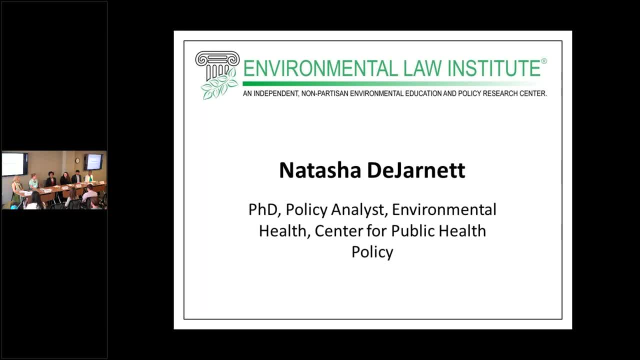 leadership calls. my boss now called in and said: hey, we're hiring a policy analyst in environmental health And I said this might be my chance to get in policy And luckily it was. So what we do and The community about policy is absolutely, truly true. We support America going against the 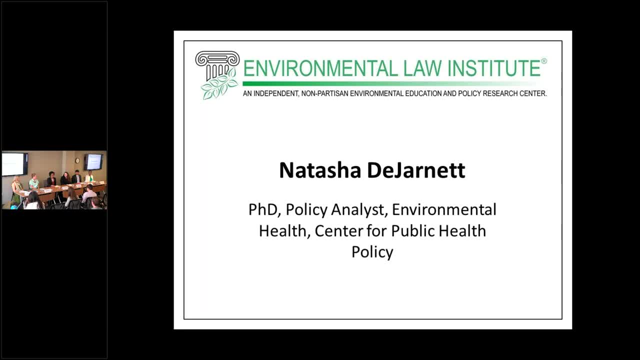 fact sheets, webinars. We have educational opportunities to inform those that are decision makers, to inform the general public, to build a ground swell of public opinion, or to inform those that direction has its own government relations department, so that work doesn't fall. 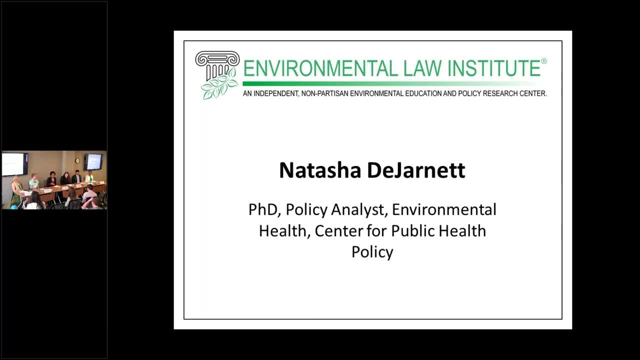 under the policy center. but what we do in the policy centers? we serve as subject matter experts for the staff throughout APHA, including government relations. so I am on the environmental health team and I lead our natural environment portfolio, which includes air, water and climate change. I've been at a 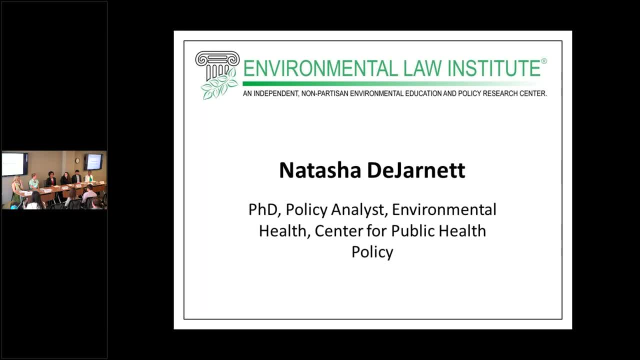 PHA for three years now. for the last two years, my work has been almost exclusively around climate change and health and it's been exciting- it's not a huge jump from my background and air quality and health, because that certainly informs climate change and health, but it has been a challenge much. 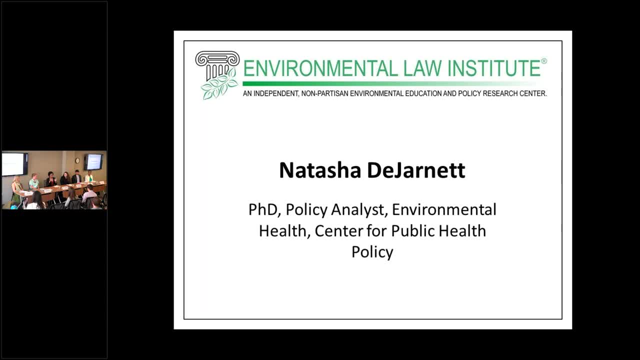 of my understanding on climate change and health has been from on-the-jobs learning, so be adaptable, always be ready to continue research because things continually evolved. last year was a huge year for APHA around climate change and health and hopefully that'll serve as no tip momentum to continue forward. but last year we 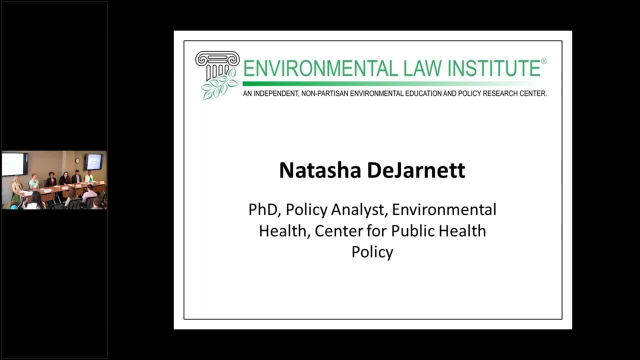 launched the campaign- the 2017 year of climate change and health. the timing was interesting. when we decided the timing, but certainly thought about when we decided the timing, but certainly thought about when we lost our misery. we were getting lots of persecutes. we had tough times at the. 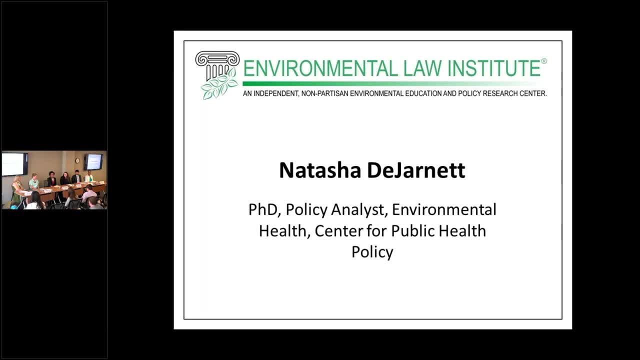 lack of emotional resources. we didn't know what was going to happen in the administration change and we didn't necessarily predict which administration it would be, to put that very politically correct. and so once you know elections happen, they said: you know, we're gonna stick with this, we're gonna 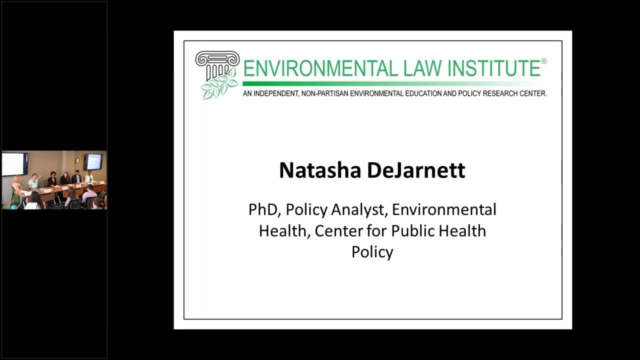 go forward with this. we had zero funding to start with for climate change and health and the year one off without a hitch. we did receive some funds to partnered with us and offered their services, their expertise and kind to move the year forward. So each month had a different theme around climate change and health, climate justice. 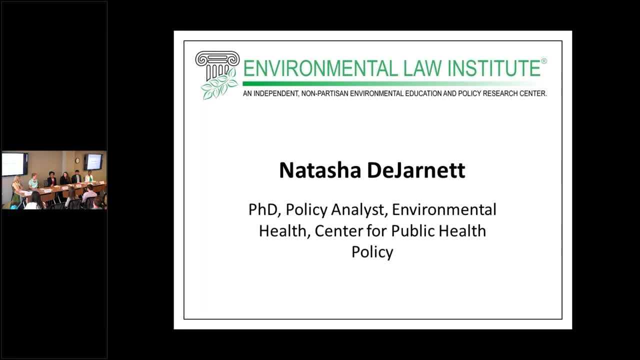 vulnerable populations, agriculture, water quality, air quality, et cetera, et cetera, et cetera. It's all on our website at APHAorg slash climate, But each month we had webinars, we had activities or workshops and we had many blog posts that. 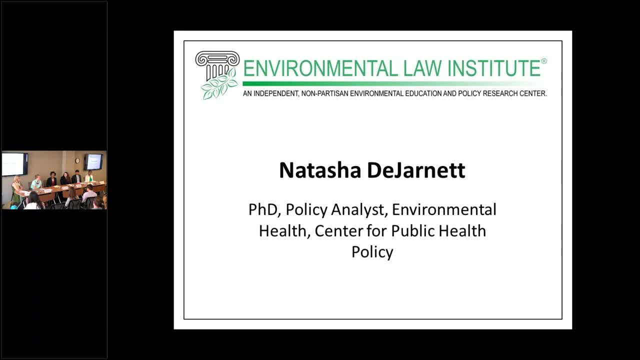 were contributed by experts to bring together these different topics, So we have really increased the amount of information that we have on this topic, And so when we do meet with policymakers or decision makers, we have a large amount of things that we can share with them on whatever interest would connect them with this topic. 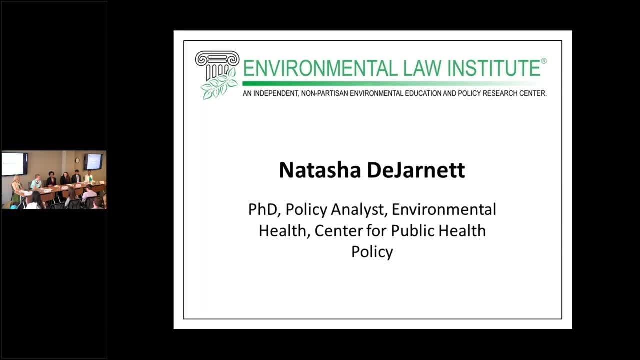 We've also done work on responding to the Flint water crisis and numerous other environmental health issues at the same time, But my work is primarily digital, So we've been around climate change and health. So the challenge therein, as I said or as I've alluded- funding. 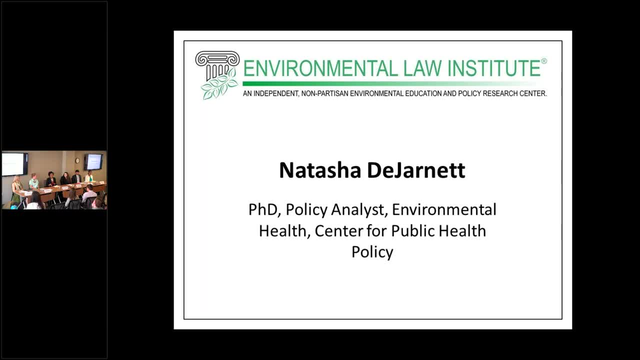 We are great on funding on climate change and health right now, but the work has to continue to move forward, And one thing that wasn't appealing to me to continue in a university is that every five years your life kind of hangs in the balance as you go and apply for funding again. 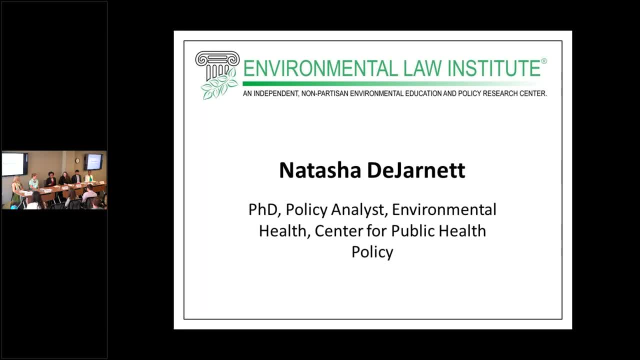 And I thought that was not a great. not great for my stress levels, I didn't. I didn't handle that very well. Who knew I was coming into the same scenario? Two of our big grants are ending this year, And so we're in the process for reapplying for some of our climate funding and some of 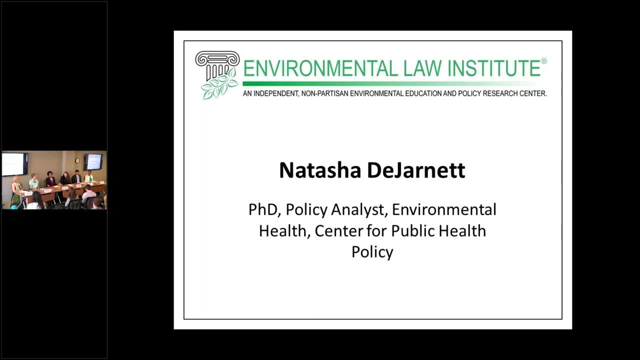 our environmental health funding. So everywhere you go, funding may be a concern. I don't think we can run from this, So that's something. And then it's a tough climate to be looking for climate funding, for lack of a better word. 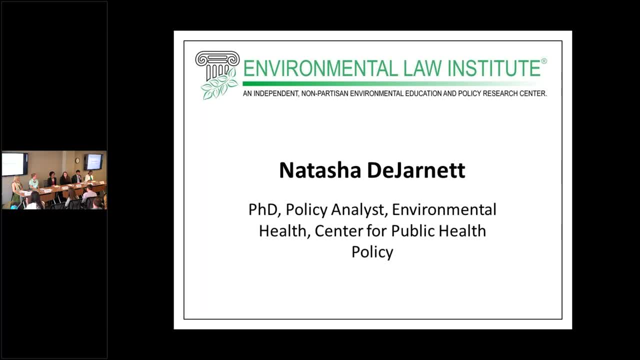 But it's there. There are people that are interested in supporting the work moving forward, especially on the level of philanthropies And then for valuing environmental policy and law. we definitely look for many opportunities to connect with professionals and environmental policy and law. 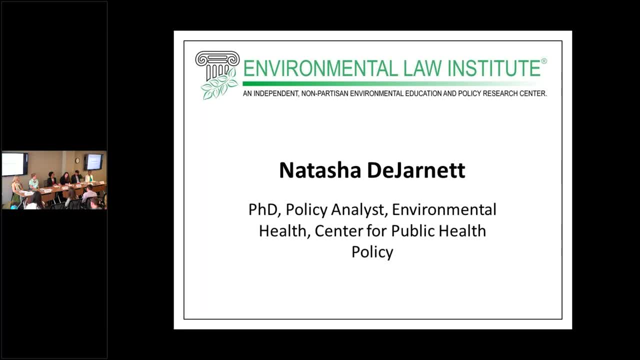 So that we can bring the public health voice into the conversation and make sure that health is considered in environmental policies. In addition, we all within environmental health, facilitate several partnerships. I was one of the facilitators for your climate change and health partners And we had about 60 part organizational partners. 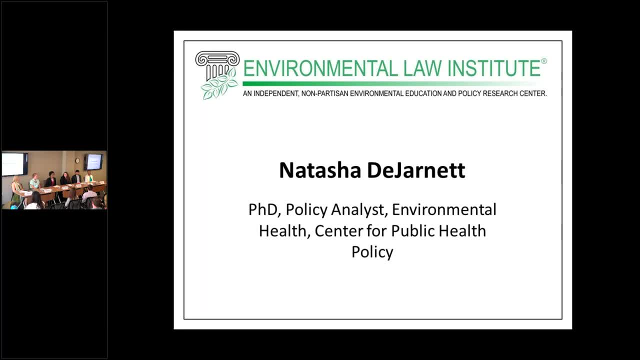 I'm also staff liaison to the National Environmental Health Partnership Council, which brings together senior and executive level leaders. We have Self- embarrassing- and senatorial leaders on the research department, which will meet with city council members and other finance ز Mon 거 They create. 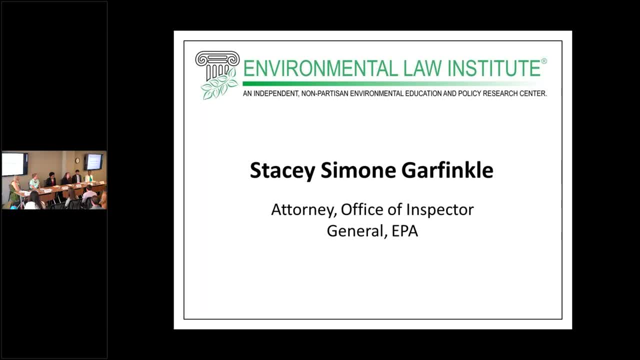 priorities and they create documents to add Pants of environmental health among those including climate and other environmental health concerns. And with that, I'll be glad to take questions at the end of the panel. thanks for your time, Hi everyone. My name is Stacey Garfinkel and I'm Associate Counsel with EPA's Office of Inspector General. 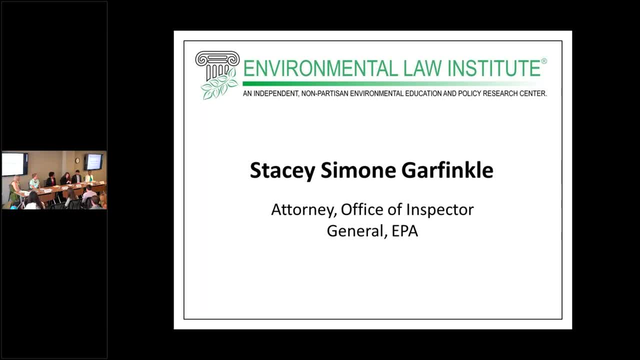 And I've worked with the Office of Inspector General for six years each, for the five years that we've been here in Utah. But a quick disclaimer: I'm here in my personal capacity, So anything I say or views I express are my personal views. 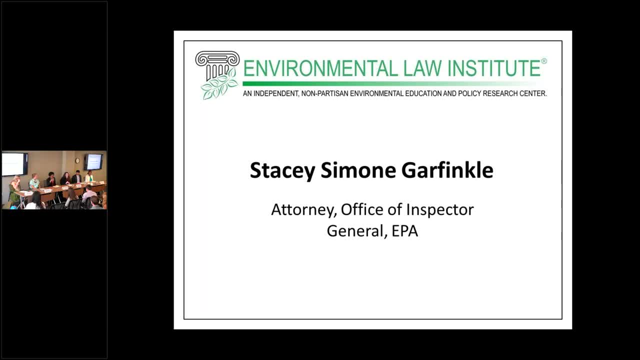 Nothing should be construed as reflecting the positions or views of US, EPA, EPA, OIG or the federal government. So a little bit about my background and then I'll get back to my work at OIG. So I've been interested in environmental issues since I was really young. 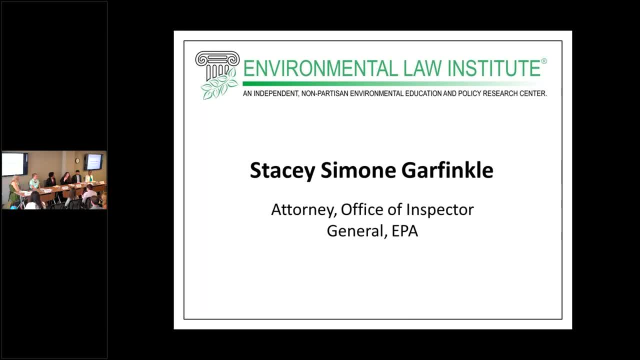 I lived in Brooklyn, New York, when I was a kid. My parents moved us to the suburbs when I was about nine And I think I don't know what it was about that move, but something about it sparked something in me. 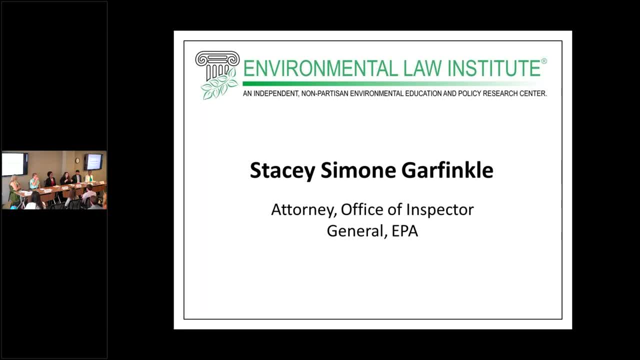 Maybe it was being surrounded by trees, maybe it was having deer in our backyard which I thought were awesome, and everybody else who moved away from the city couldn't understand why there were deer, And I'm like this is their habitat. You moved into it. 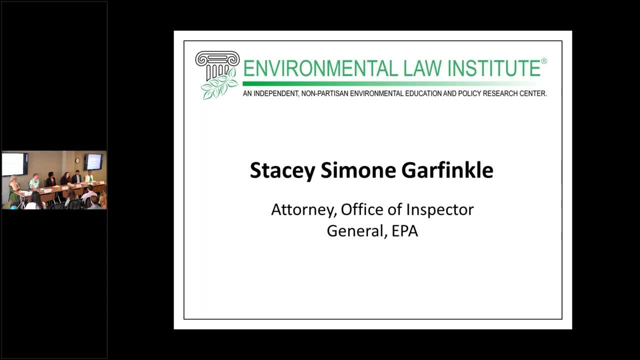 And so from that point forward, I just loved animals, I loved wildlife and I wanted to preserve spaces for them to live in. And then, as I learned more about the environment, obviously I became more interested in just air and water in general and toxics and pesticides and all those things. 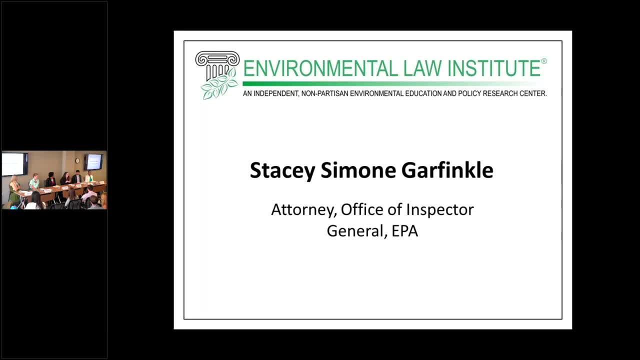 Another thing that happened and I will still never understand why she did this, but I had a teacher in fifth grade in a science class who one day showed us a movie and it was out of the blue like I don't know why. 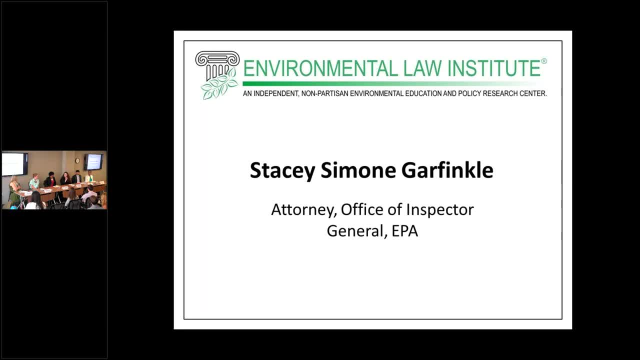 And it was this film that had been done for HBO and it was called Dead Ahead- the Exxon Valdez Disaster. And it was this film about the Valdez oil spill and, like, Christopher Lloyd was in it, but it used all this archival footage from the real spill. 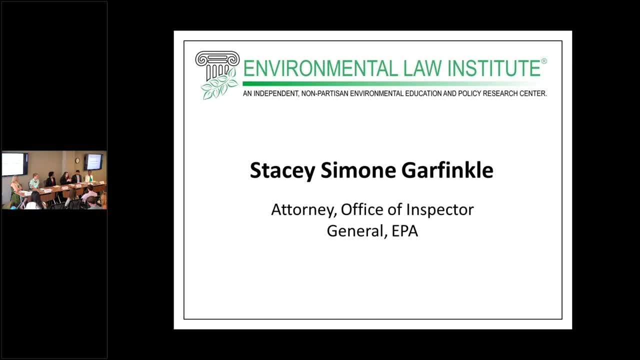 And something about that, and I was nine and seeing this footage and you see sort of just the breath And the depth of the effects that this had had like a really profound impact on me too, And so from that point forward I knew I wanted my life to have something to do with environment. 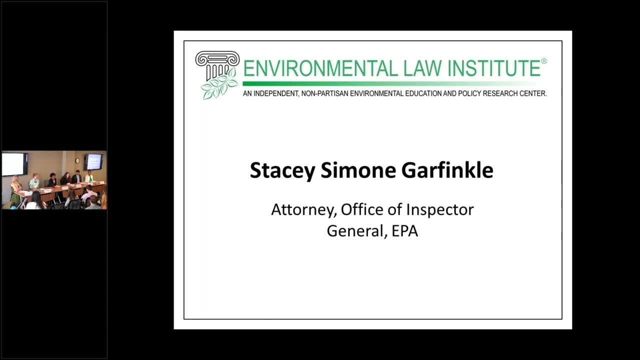 I didn't know what at that point, And then as I got older I was really interested actually more in politics and stuff like that And so we moved to Jersey. I did an internship when I was 15 with New Jersey Public Interest Research Group and they were working on like an environmental campaign and I found it really interesting and cool and engaging. And then the next summer I interned for my then senator, John Corzine, which was really amazing. I was like 16 years old and I was interning in his constituent services office in New. 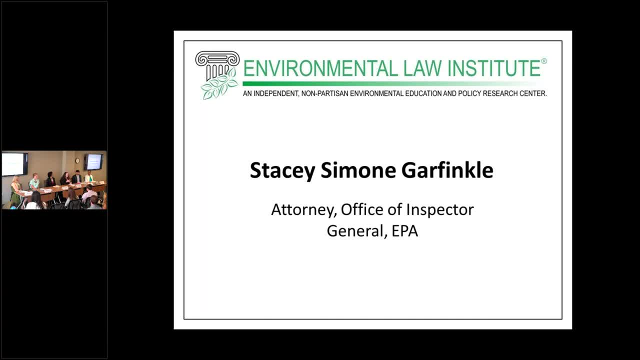 York, New Jersey, And it was a really cool experience and I kind of thought I wanted to spend my career in politics. So fast forward and I went to, but I was also interested in environmental and that was kind of what pushed me in the political direction. was this sort of underlying sense? 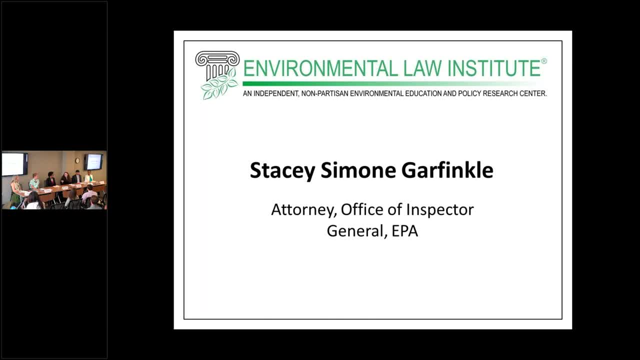 of I care about these environmental issues. at that point It wasn't really on the forefront. It was on the forefront of people's minds and I wanted to do something in that realm. So I ended up going to GW down the street for undergrad and I went thinking I would 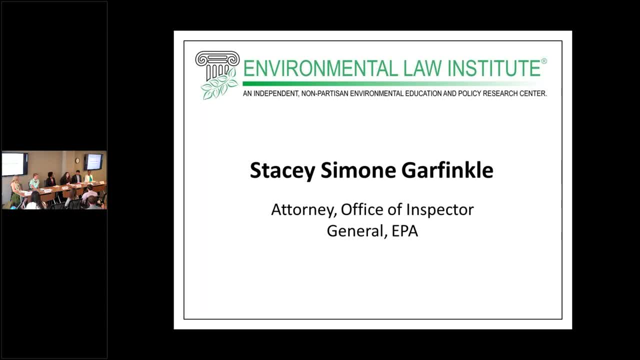 study political science and environmental studies And I happened to, my first semester, take a criminal justice class which was housed in like our sociology department at GW, and I fell in love with that class And all of a sudden I switched my majors to political science with a focus in policy. 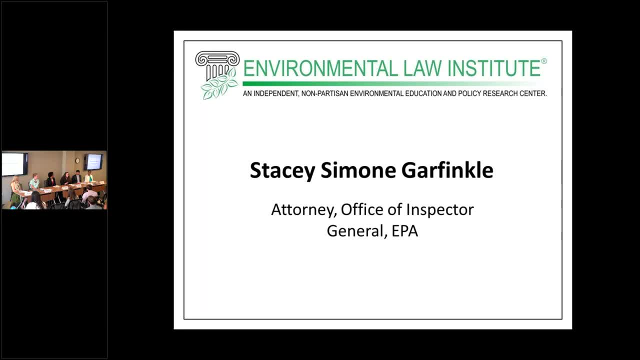 and criminal justice And those criminal justice classes really sparked my interest, I think for me, an interest in law which was always in the back of my mind, but I didn't really know if it was something I wanted to do, And so while I was in college, I was very politically active. 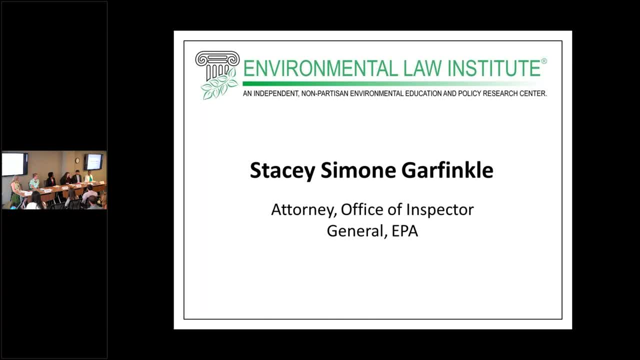 I ended up being president of College Dems thought I really wanted to kind of go the political route. I did some internships, including for League of Conservation Voters, and I wasn't working on environmental policy. One was a campaign they were working on for the 2004 presidential election aimed at some battleground states. The next summer I went back and worked on development and fundraising- Really policy-related- But then what happened was I was doing this policy focus and GW had these like five-year programs where I could stay an extra year and get my master's in public policy. 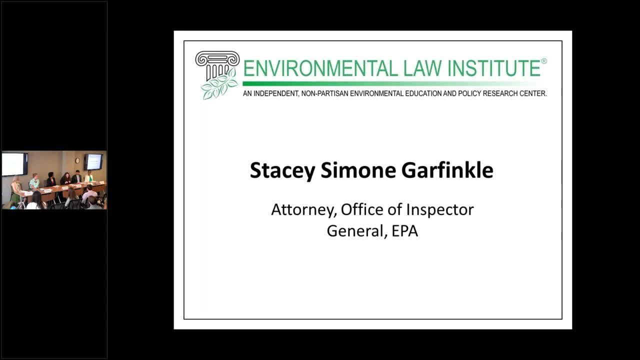 And I did that And originally I kind of went into it like I crafted this special concentration where I would be taking classes in the School of Political Management, like all with this thinking that I wanted to do more political stuff or campaign work, and ended up really loving 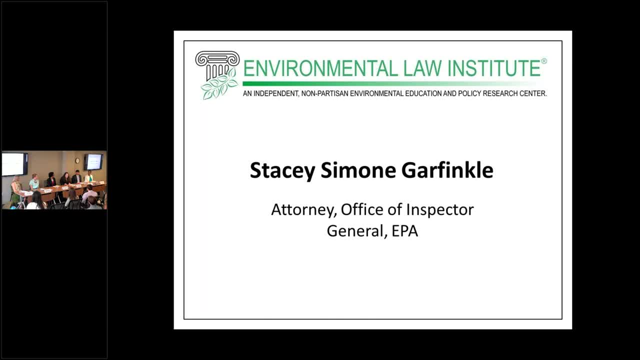 the policy side of it, And so I worked part-time doing government research And then I ended up really loving the policy side of it. I did a lot of government relations work for part of grad school and I really enjoyed it. But at some point I started to also look at the people in the positions I wanted to 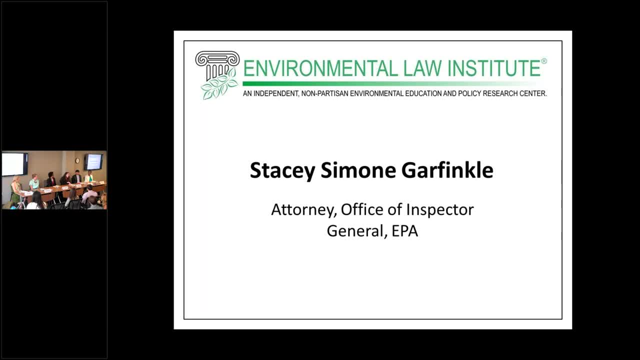 be in, and I realized a lot of them had law degrees. So whether they were practicing or whether they were lobbying, whatever it was, a lot of them had that background. So I ended up taking a couple years off trying to figure out if it was what I really wanted. 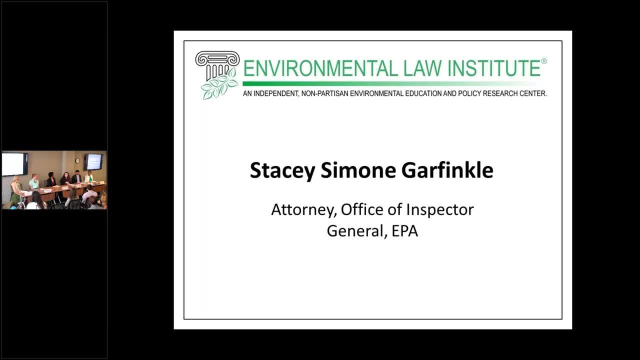 and then went back to law school and went to American- also not that far away- And so that was when I really shifted my focus more toward law. And in law school, you know you have to have a lot of people. You have to have a lot of people. 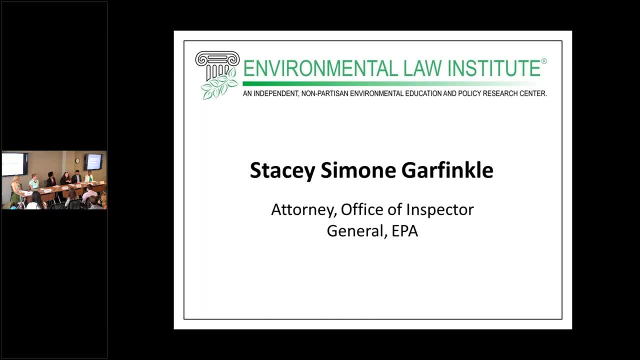 You know you have like core courses and then you can have all these electives And I was very fortunate in that American had like tons of environmental classes and energy and natural resources classes And so I pretty much like outside of the courses that I was required to take, I took. 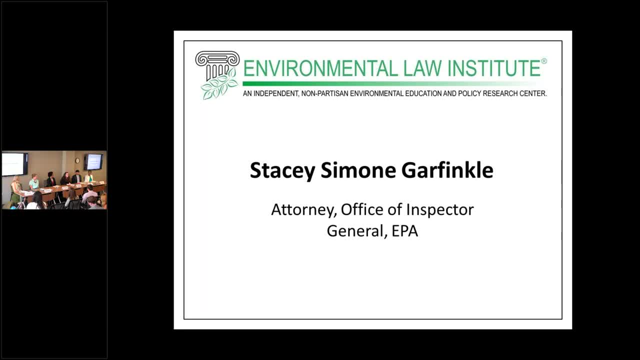 probably 90% of my classes in those areas, which also helped me to realize kind of the breadth and depth of environmental areas. Like I went in thinking, kind of smug thinking, I know what I want to do, You know like I want to practice environmental law. 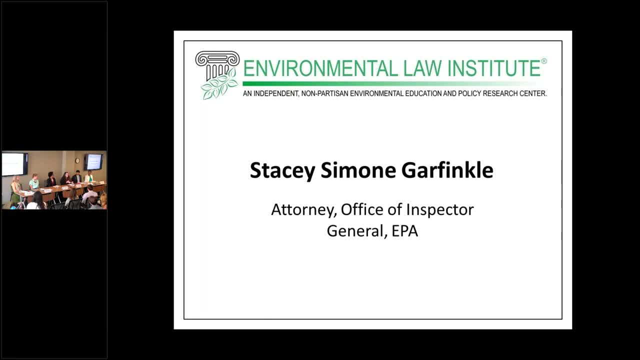 And then all of a sudden I was like, wait a minute- environmental law, or energy law, or natural resources law, Or animal law, which in some ways is related to wildlife law, And you realize how broad it is, And so to kind of try to figure out what I wanted to do, I also did a bunch of internships. 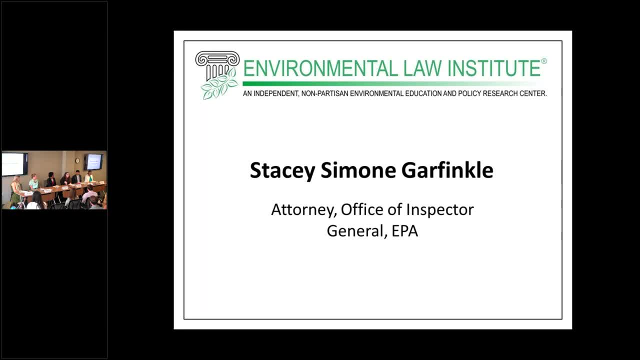 And so, starting with my second semester, my first year of law school, I started interning And I pretty much spent every semester and summer, beginning then, somewhere in the federal government. So I spent a lot of time at EPA and the Office of Compliance and the Office of Civil Enforcement. 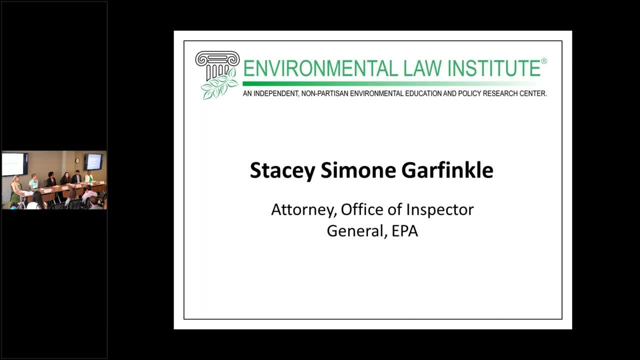 working on like Clean Air Act enforcement And the Office of Administrative Law Judges And they handle the administrative adjudications for EPA and also for NOAA, National Oceanic and Atmospheric Administration. So a lot of like fisheries cases and species and like marine mammal stuff. 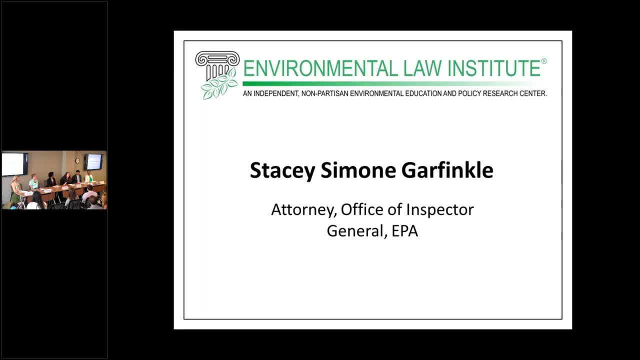 I spent a semester at the Solicitor's Office at Interior, a semester at DOJ and the Environment and Natural Resources Division And I kind of thought I wanted to go into government and was very public service-minded, even going into law school. And through those internships I also realized that, you know, even if I – and I wasn't 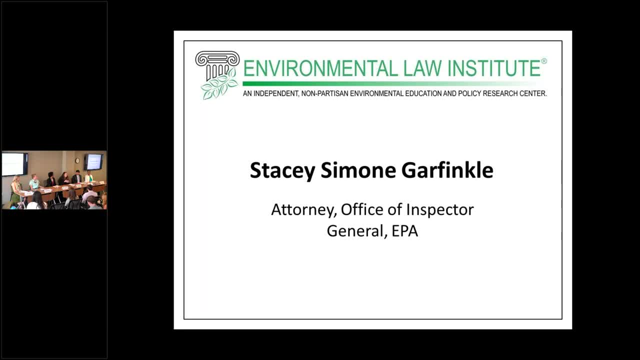 sure at that point if I saw myself in government in 10 or 20 years but knew that it seemed like a very valuable experience to get, And so when I graduated, I ended up going back to EPA as, like a fellow. 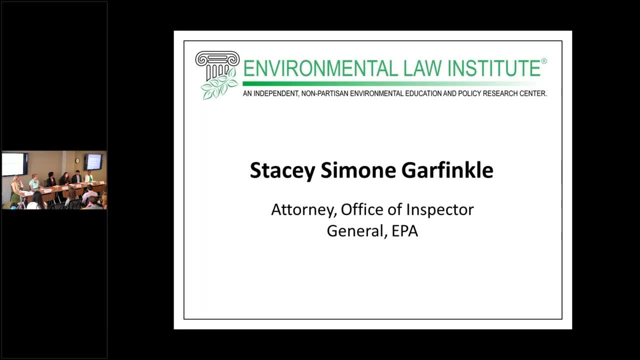 And then I worked briefly for the ASPCA doing some like animal welfare regulatory work and then ended up getting my current job in the IG's office. So the IG's office is a little bit unique because we're an independent office within EPA. 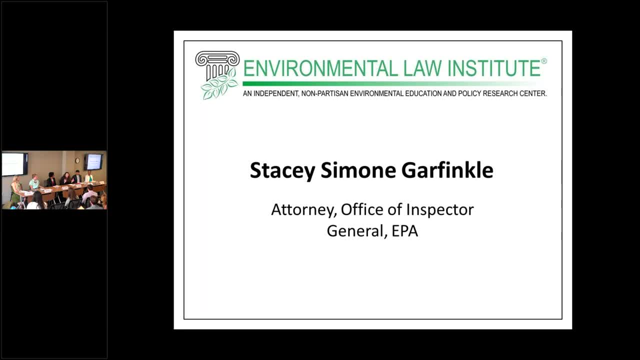 And we're charged We – again, I'm here in my personal capacity, But it's an exciting place to work because we garner a lot of interest from Congress and the press and the public and the agency ends up taking like pretty concrete and 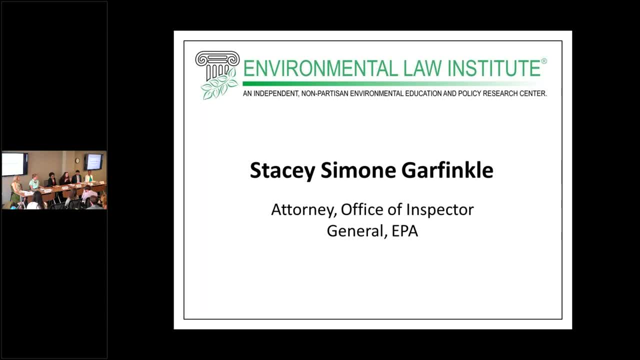 sometimes very significant actions off of recommendations we make. So what do we do, though? We serve like an oversight function, So our mission, sort of broadly, is to detect and prevent, and detect like fraud, waste and abuse in agency programs to help increase the efficiency and effectiveness of the agency. 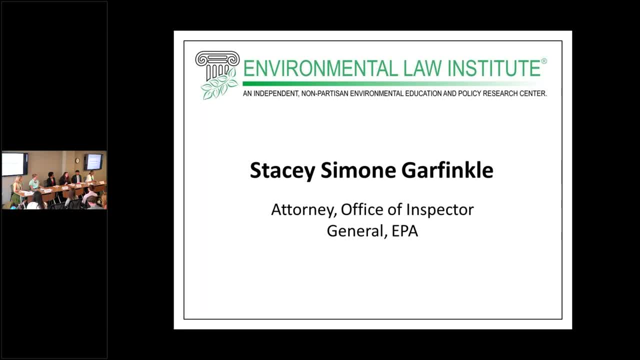 the agency as a whole. And then also we have like investigators who are investigating things like contract fraud and grant fraud and stuff like that. And the way that we do that is that we have like auditors and program evaluators as well. 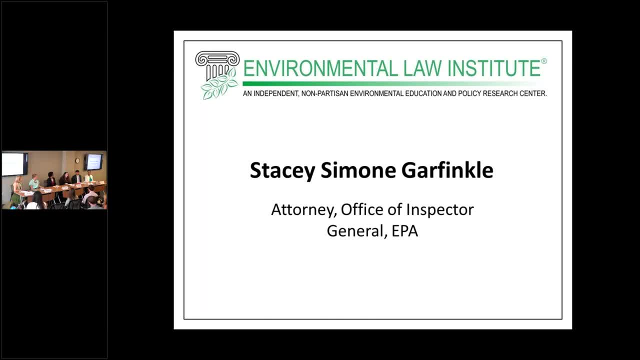 as investigators I mentioned, And our program evaluators. it's kind of cool. They sort of track the EPA program offices, So like there's an Office of Water, an Office of Air and Radiation in EPA, And so we have evaluators who just work on air and who just work on water. 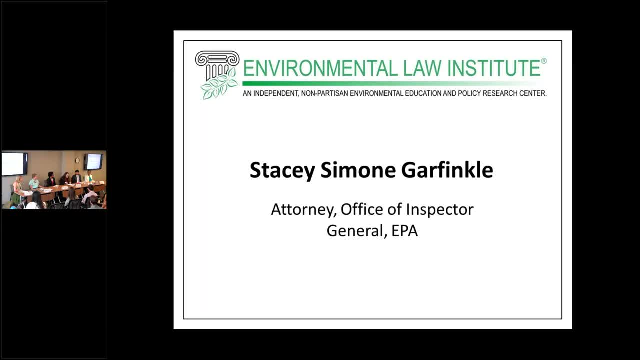 And it's kind of cool. So there are like a lot of environmental aspects too. All right, Thank you, Thank you. And then we receive like requests to look into various matters from, like the public, from other employees, members of Congress. 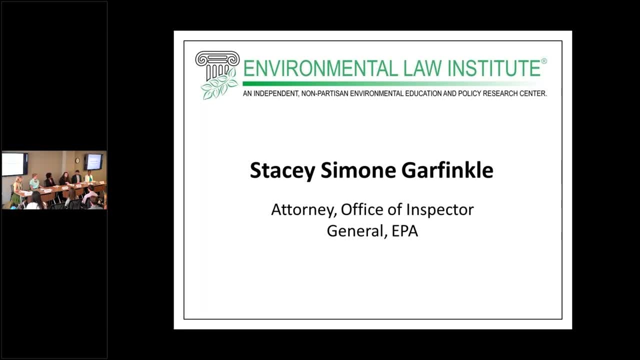 Our office has been in the news a lot lately because we've been asked to look into a lot of things that the administrator has been up to and that the agency in general has been up to, And the work that we do tends to like culminate in reports. 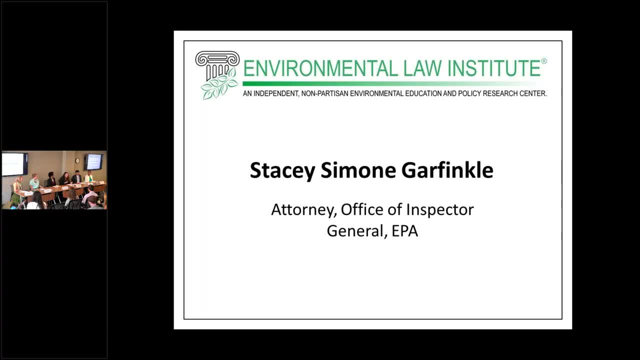 So it's audit reports, It's investigative reports, It's program evaluations And, like I said, they tend to get a lot of scrutiny from like external stakeholders Right And from the public, And the recommendations, as I said, can often have like very significant impacts on the 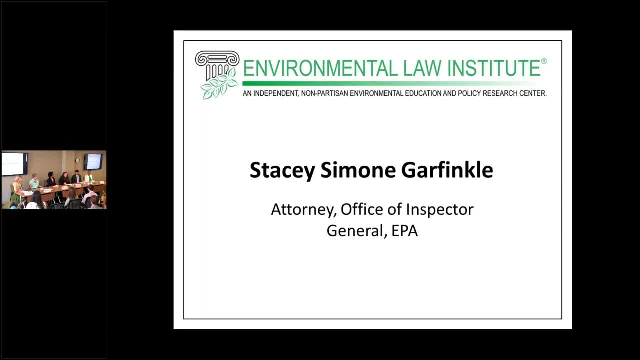 agency And often we ask them to do things that are going to be, you know, an expenditure of resources or funds, And the agency is constantly doing more with less. So we have to really make sure that everything we're doing is sort of supportable and defensible. 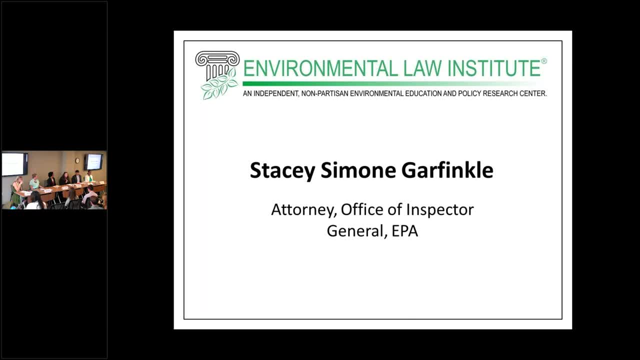 in terms of the recommendations we're making And that's sort of where my role comes in in the Office of Counsel. So every single like audit evaluation, investigative report that goes out, like before we go into the public, before it is sent anywhere or made public, we review them. 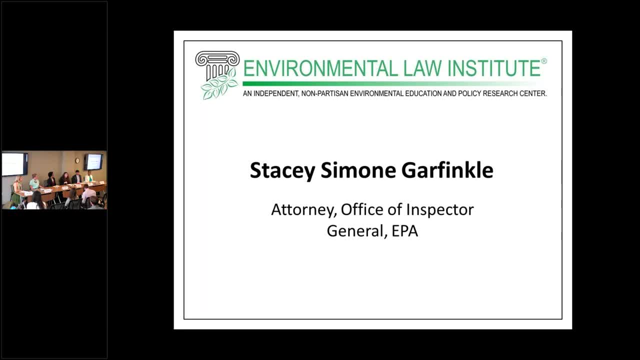 And we review them for legal sufficiency. So we want to make sure that, like any law, reg, policy guidance document that's being cited or relied upon in any way is being cited correctly and properly applied so that the conclusions and recommendations that flow from them are legally supported as well. 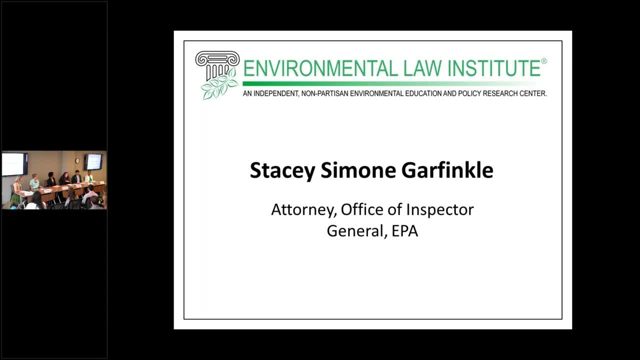 So it's an interesting job because we deal a lot with EPA-administered statutes- So Clean Water Act, Clean Air Act, RCRA, CERCLA, all that stuff- But then at the same time, like we also do, a lot of client counseling. for the rest, 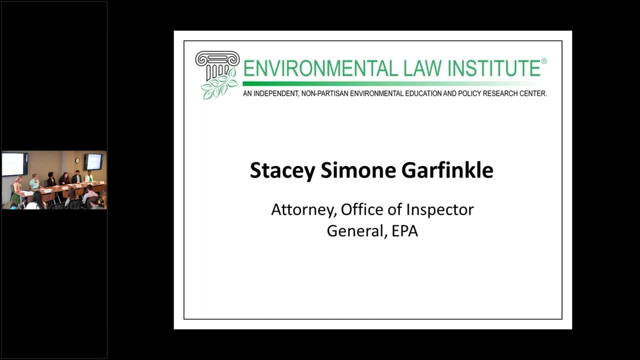 of OIG, because they're basically their general counsel's office And so it's a lot of general law issues too, And so it's interesting because I get to work on environmental stuff, but I also work on appropriations issues and HR-related matters and employment law. 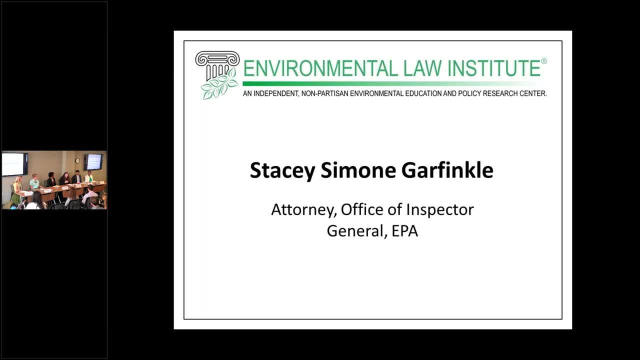 So it's pretty cool. Our office also handles FOIA and FOIA litigation for our office. We also do some employment administrative litigation for like OIG employees. So it's pretty cool and it's been an enjoyable experience. I think the one thing I would say is: it's a type of position where- because it is a lot- 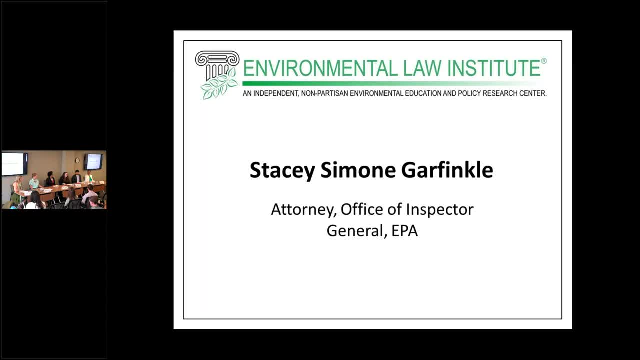 of general law. it's sort of something where, to me, the benefit is that we're really helping to support EPA and helping the agency run more effectively and efficiently and kind of contributing overall to EPA's mission, as opposed to necessarily doing like substantive. 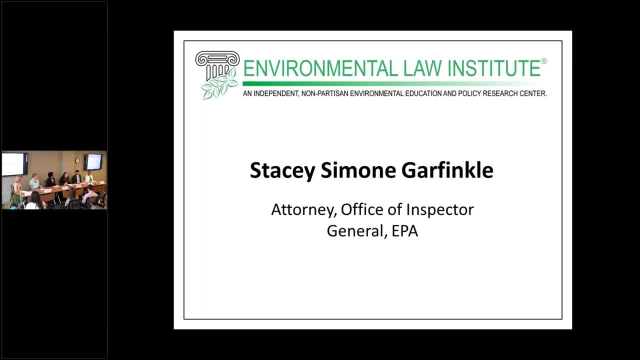 environmental work on a day-to-day basis, And I think for me that was something that I had to really consider was like: what do I want to be doing? Do I want to be doing like substantive environmental work? Do I want to be doing environmental work every single day? 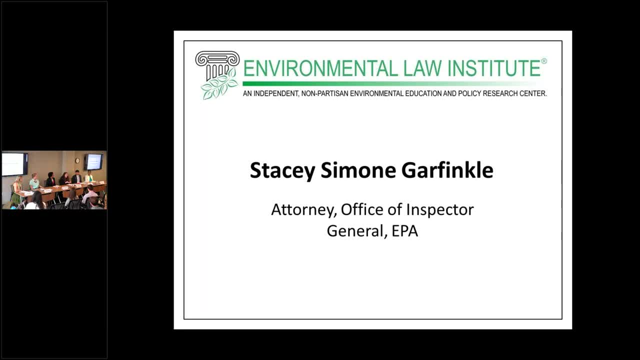 Or do I want to be in a position where I feel like, at the end of the day, I'm really contributing to, you know, the mission of an agency that I really care about, And that's sort of how I view my work. 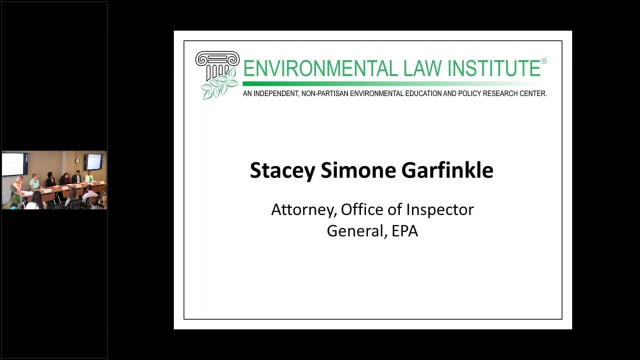 And for anyone who's interested in oversight work, pretty much every agency and department has an OIG. It's sort of a plug. So there's EPA OIG, Interior and USDA have OIGs, and Commerce, which houses NOAA as well. 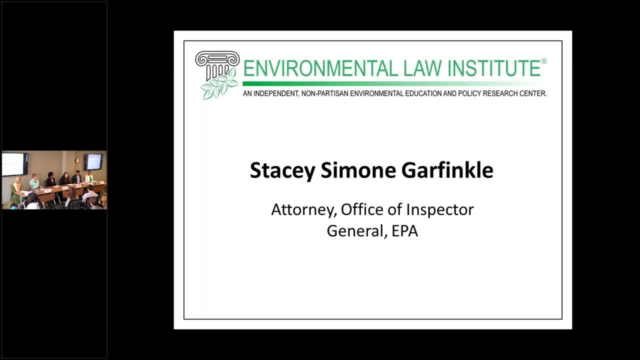 So it's exciting. I think to me sort of the reward and the benefit is seeing recommendations that we make going into place in the agency. And it's interesting sometimes- I'll be, you know- reading evaluation reports and it really sheds a tremendous amount of light on agency programs that people aren't really 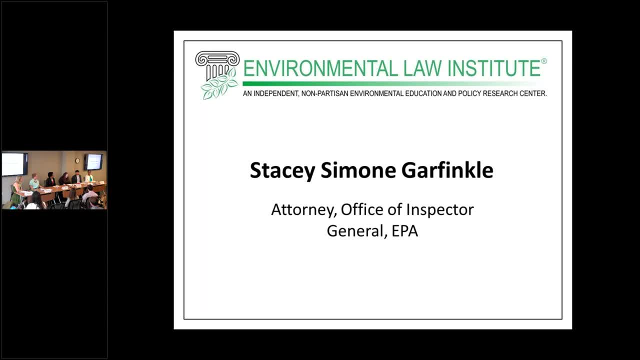 scrutinizing. for the most part, You know EPA's been doing things a certain way for a long time and then all of a sudden you have evaluators going in and looking at it and really realizing that there are a lot of improvements that can be made. 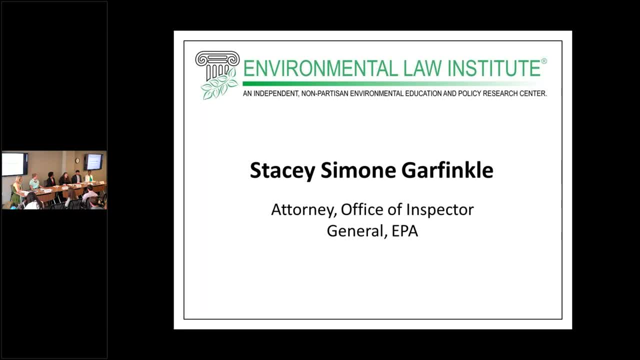 And so it's really kind of cool to see those sort of real-world impacts And, you know, every time a recommendation is sort of accepted and they're taking corrective action. it's pretty cool. You feel like you're really contributing to that. 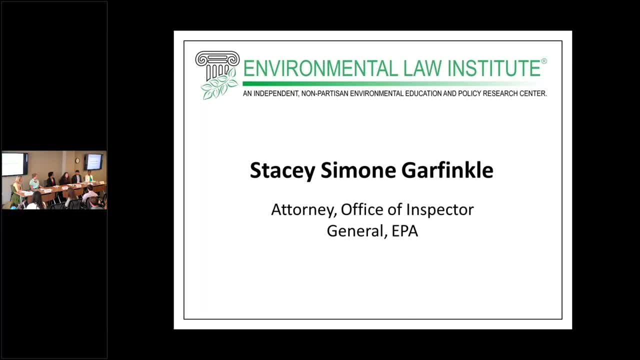 It'll be awesome. Your office is contributing. As far as challenges- I think government-wide, for anyone who's interested in government. you're constantly being asked to do more with less, And I think that's a challenge not just for my office but anywhere. so you know having 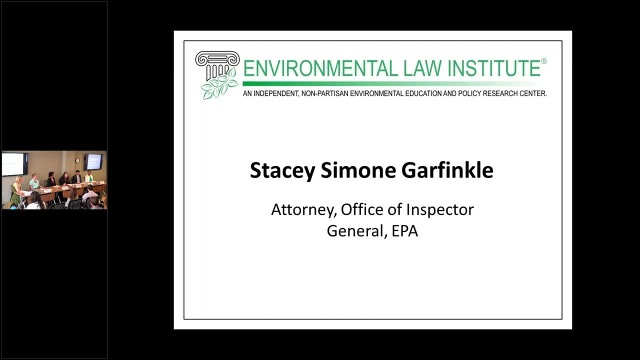 the same amount of work, or more work, but with fewer resources to do it. And then the other thing, because we're independent, is making sure that we really are truly independent. And that's tough, especially, you know, right now, in this climate where it's very politically. 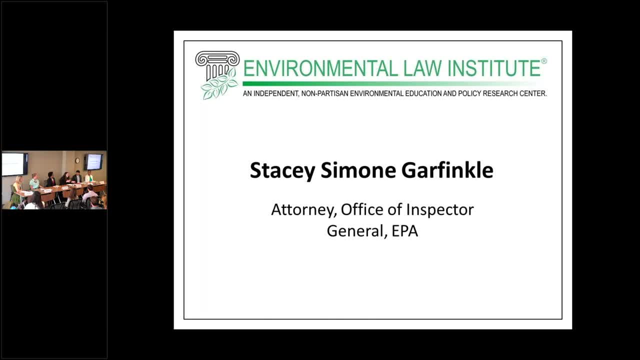 charged and we want to make sure we're not, you know, seen as favoring the administrator and is, you know, going after anyone in particular, And so I think that's definitely a challenge and sort of a unique thing about like an OIG. 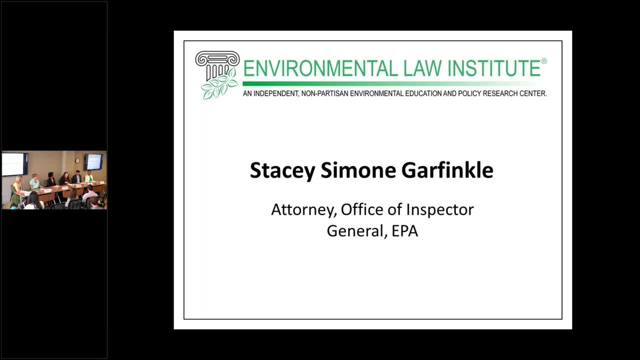 or an oversight role. But yeah, that's it And I look forward to taking questions. Well, my name is Dimitri Karakytos. I'm a partner at Holland & Knight. I guess I'll start off by saying I never grew up with any sort of interest in the environmental. 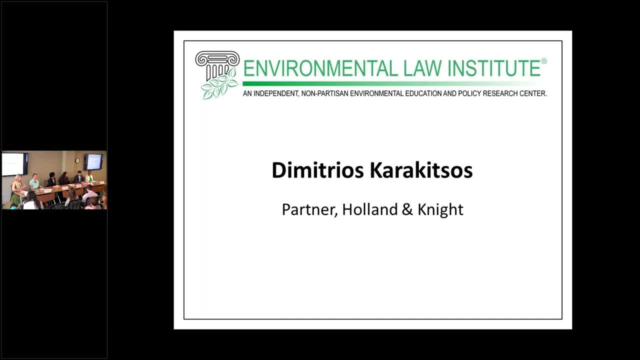 space. And if somebody had told me in law school or even early on in my career that you know in my career that I would have done things that I had done or worked on, I would have thought they were absolutely insane. So I grew up in the Lansing area of Michigan, which is the capital city of Michigan. 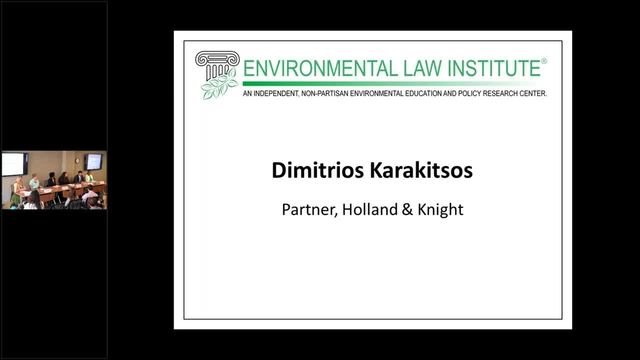 In undergraduate I was really drawn to public policy and politics. When I was in undergraduate I interned for my local congressman. I also after that interned for a local state and local lobbyist that I had grown up knowing, And both jobs I absolutely loved. 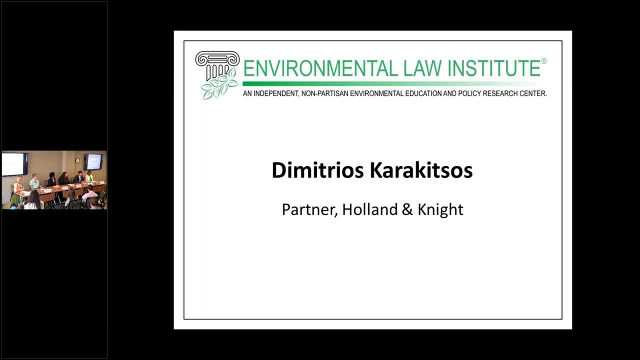 And I think a lot like Stacey in both offices and when I went and talked about to people about kind of getting into politics and the policy space, I heard very frequently law school was a great education. It's a great way to get your foot in the door. 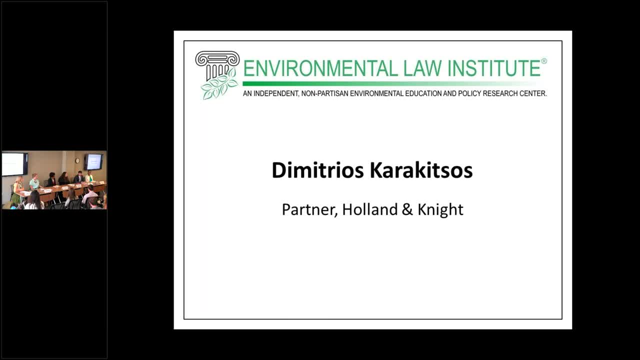 It's a great kind of Yeah, It will just be helpful for you in that career. so you should really think about it when you graduate undergraduate. So I did that. I ended up going to law school down in Florida And instead of, you know, kind of the focus on the traditional legal side of things. I 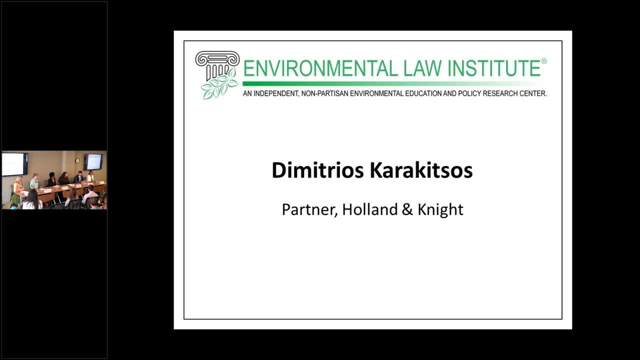 always kind of knew it was an end to get or a means to get to into the public policy space. I focused a lot on constitutional law. I took a lot of state and local law. I took a lot of state and local law classes, international classes, just to get as much experience as I could. instead of you know, in between semesters in the summer, instead of working at a law firm, I pursued some work with somebody down there who was heavily involved in state and local politics and had previously been involved in national politics as well. 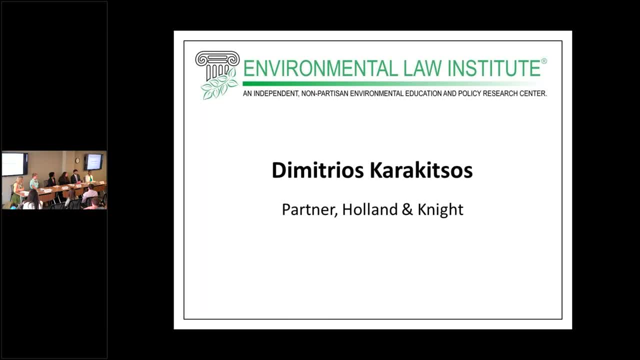 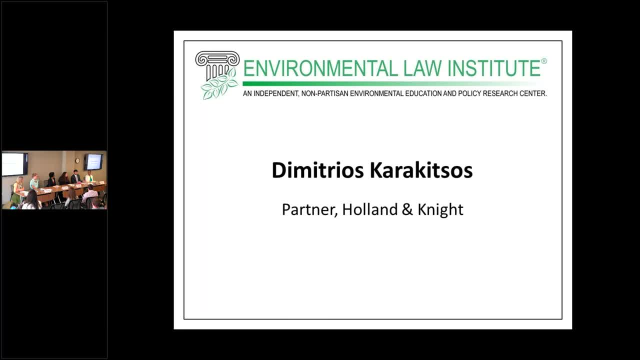 I went to law school, I decided to come to DC. I had no kind of ends here. I had no thought of what I was going to be doing. I actually came at the start of 2009.. I am a Republican And at that time it was not a good time to be a Republican in Washington DC, with the White House flipping over pretty much a super majority in the Senate and a huge majority in the House of Representatives. 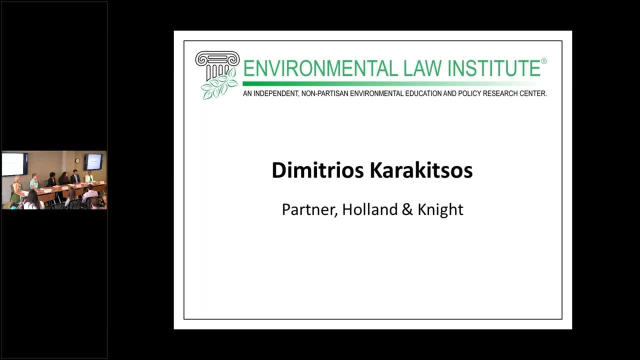 The first opportunity I got just kind of dumb walk. I heard of a legal internship at the Senate environment public. I had no idea what that was, who was on the committee, what they did anything about it, but I jumped at the opportunity. I did a lot of googling just to figure out. 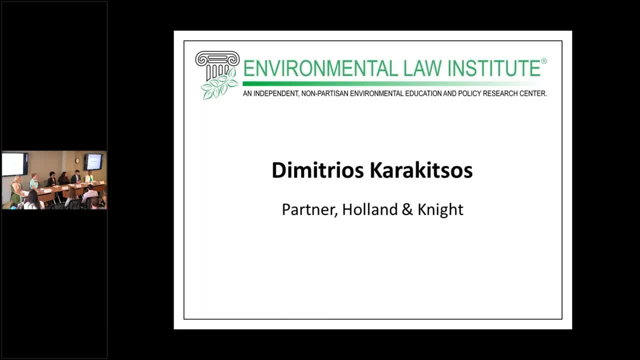 what was going on there and what kind of work they worked on. I applied and I got basically what was a temporary four-month legal internship there. I think I'll say, just for those who haven't worked on the hill, I think it, you know, incredible experience. I'm so glad, did it. it's it's certainly less. 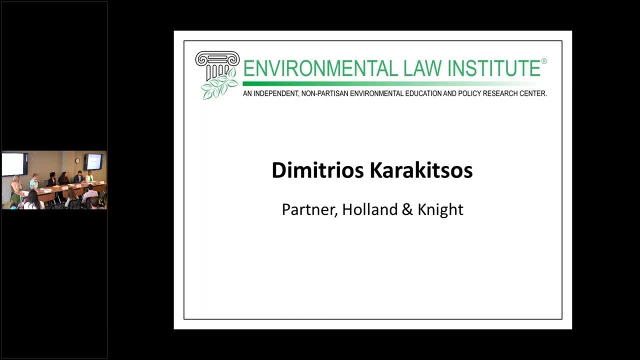 than glamorous. at times it was difficult watching friends in law school get associate positions at law firms and start making good money and I'm an intern on the hill answering phones and, you know, responding to letters. but that's just kind of the way that the hill works and I think it applies to. 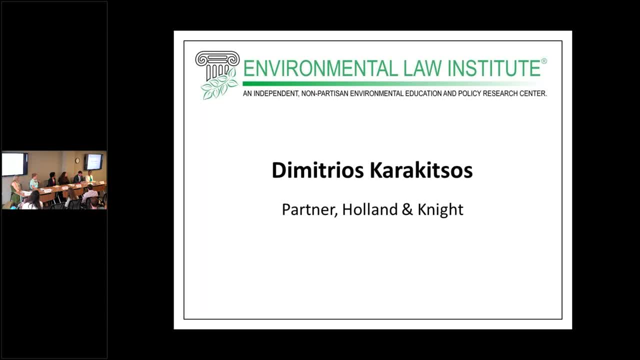 outside foot, you know, outside the hill as well, but certainly on the hill where you really have to start at the bottom, work your way up. just another one of those right time, right place moments where my internship was coming to an end and they had a full-time staffer leaving and, because I had been there, got to know. 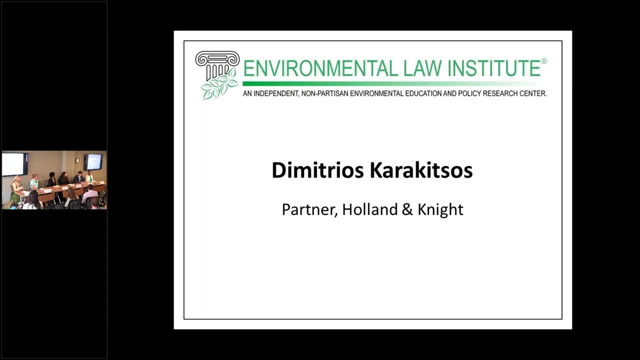 folks. they offered me the full-time position and again it was still doing more of the same- answering phones, responding constituents and things like that- and I could say back to them: that hold until 2 am. you're like I'm off, then get 50 seats. what time of the day is it that evening? so then it goes everyday. 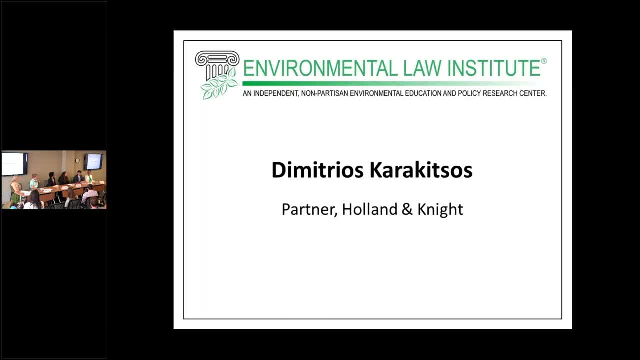 but I can't find a full-time job. I can only meet one person because I had a. maybe not. it could be a little bit cold, it could be intense, it could be some kind of stumbling block. it's all self-degradation up for me, you know. 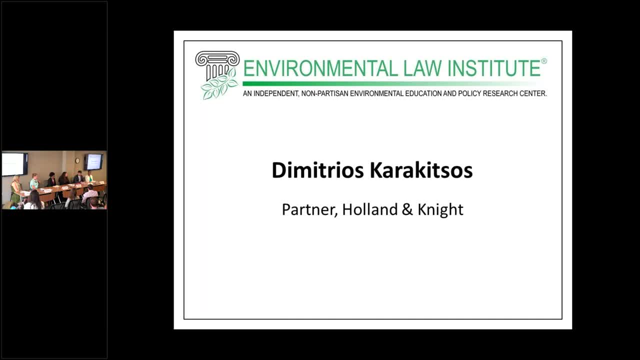 when did you get the palavra student residency? how fast are you able to get рез說 the strictly you know what time of the day, whatever tone you are want to do? something that was see whether that's all oikea were gonna fail to get to不是. 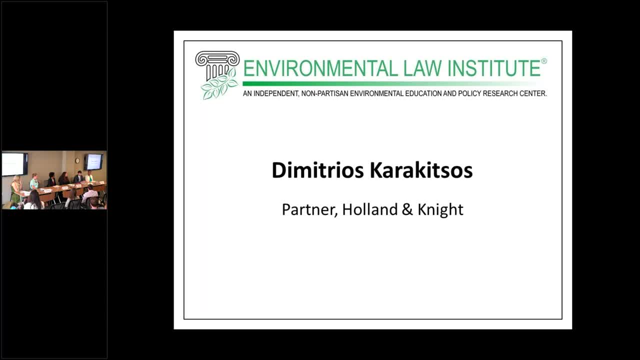 when a senior kind of career staffer came in or senior staffer on the committee came in and said kind of looked at me and said you're not who I was expecting to see sitting here And I could see on his face he needed help with something. 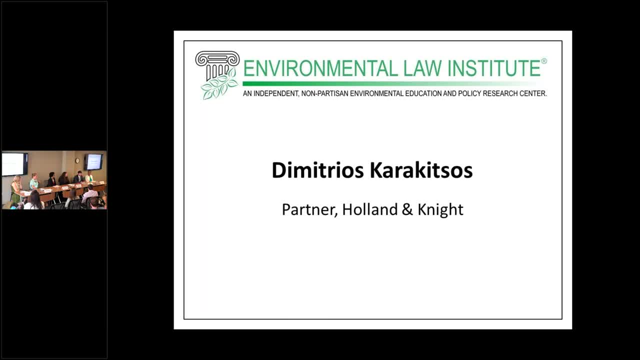 but didn't want to ask me and didn't know if he could trust me to ask me, right? And I said: can I help? What can I do? What can I do? And I was eager enough that he said: all right. 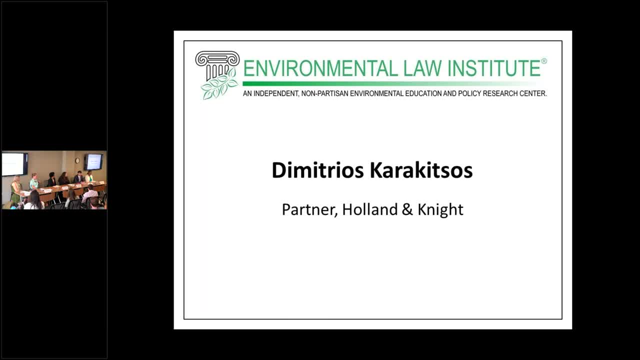 let's see how this goes. And he gave me a task to do, And you know I did well enough on it that he then started coming back to me instead of the other person. So you know, you just start kind of getting. 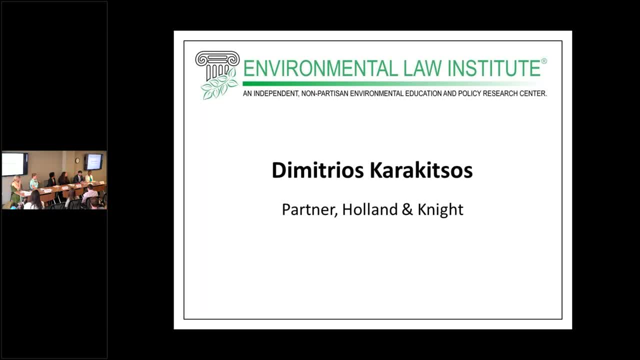 into those situations and, you know, learning as much as you can. I got very, very lucky in my role there in that I got to back up, for part of my time as a junior staffer, the deputy staff director of the committee. He had a broad portfolio, kind of touching everything. 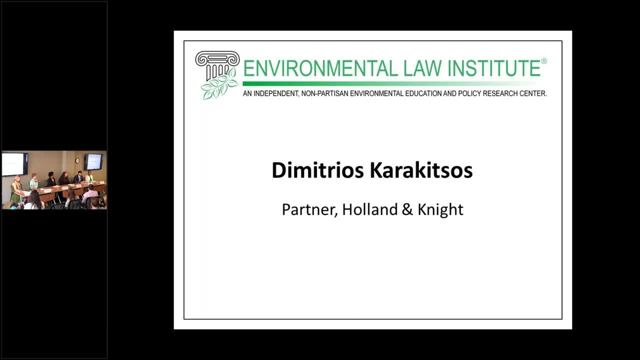 energy environment on the committee and, you know, served as kind of a mentor for me And I would say I got beyond lucky because of how smart and well-respected- I think on both sides of the aisle- this person was. He went on to be run energy environment policy. 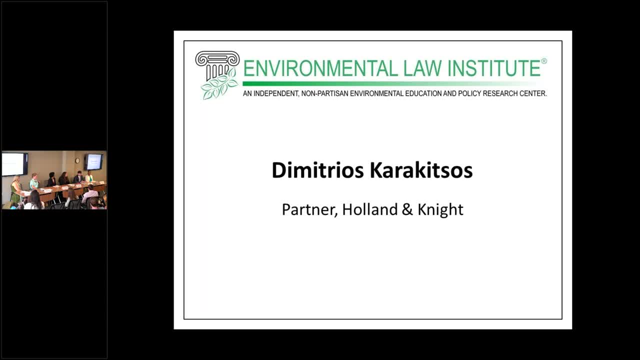 for Speaker Boehner and then, until very recently, for President Trump, So very well accomplished, great person to learn from on the job. The first issue that I got to take over on my own was the chemical portfolio on the committee. I won't kind of directly quote it, but I think it's, you know. 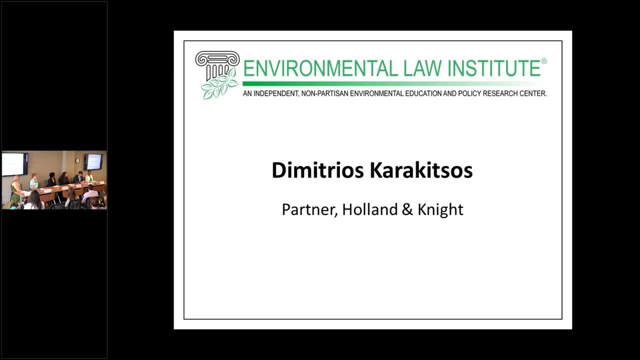 a quote what I was told when I got it. but just to paraphrase a little bit: I was told: this is never going to take up much of your time, This won't be a big deal. You know, there's a partisan bill out there. 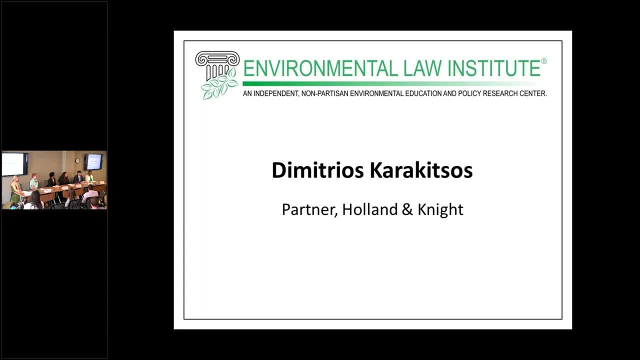 It was Senator Lautenberg from New Jersey's bill. The business community, the right- didn't take it seriously. Every year the committee basically had a hearing on the bill very divided. The left talked about the need for it, the right talked about how bad it would be. 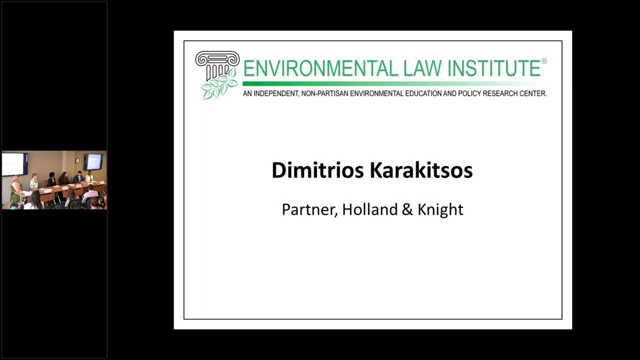 And it was kind of a stalemate. So that's the expectations that I got going in to that first issue And I'll kind of go back to how wrong that was in a minute. But you know, as I continued at EPW, 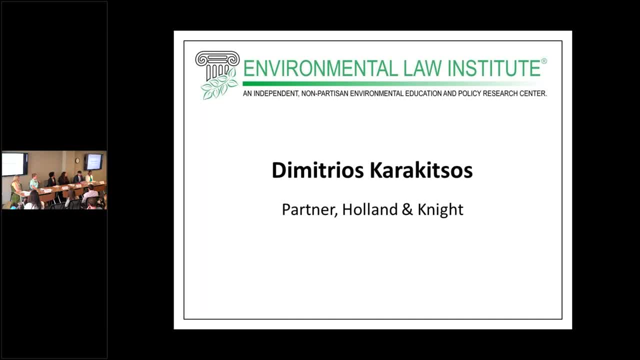 my role expanded in many ways. I got to help negotiate environmental streamlining provisions, for example on a major infrastructure bill that passed- And as contentious as that can be, I mean that then passed with broad bipartisan support, Signed into law. 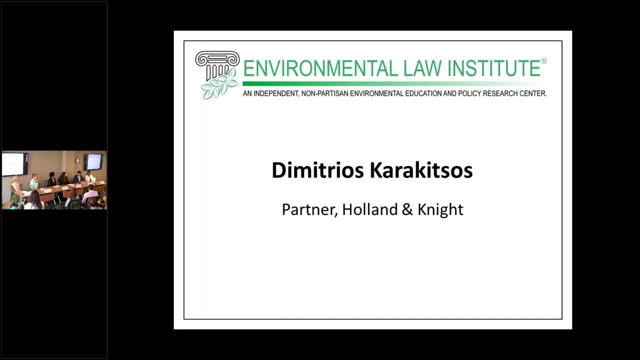 And that's. you know, that's a fun issue, that's kind of ongoing. every infrastructure bill You talk about the balance- and I think I'll probably use that word a couple of times- but the balance between trying to get these roads and bridges built, or water infrastructure, whatever it is. 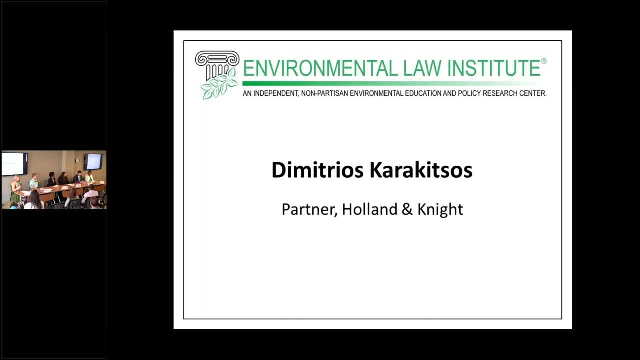 and how to appropriately protect the environment, human health, things like that, Because you know at that time we had bridges collapsing right. You don't want to unduly delay these projects because there are real world impacts if that happens, But at the same time you don't want kind of a lasting 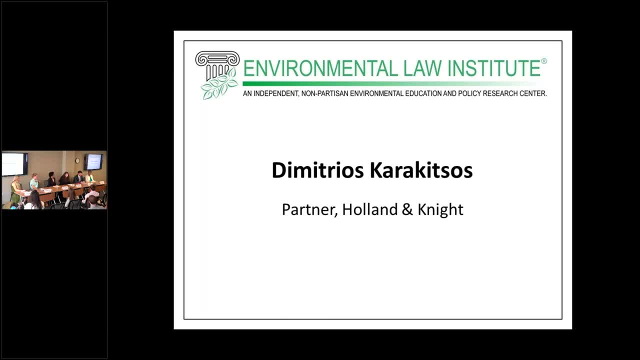 environmental or public health kind of risk from that. My primary focus for a lot of time was energy policy. I did that for both- a member from Oklahoma and from Louisiana- obviously two very energy rich states with major oil and gas production there- but also cared about renewable energy. 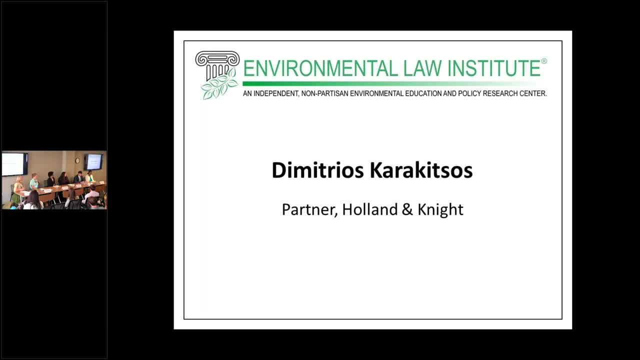 In particular in those states- wind and geothermal. I had the opportunity to work on some very high profile issues like the BP oil spill, hydraulic fracturing- kind of at the height of all the discussion about that And, being from Michigan, something that hit close to home. 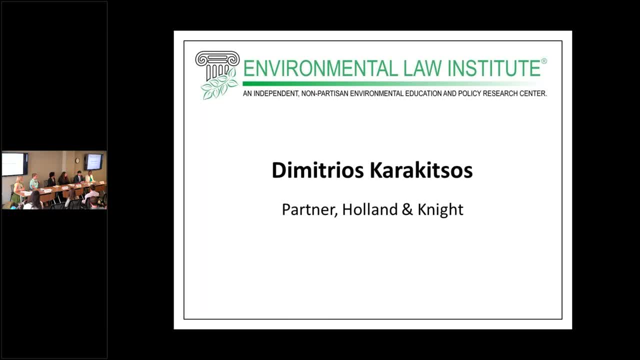 I got to go down to Flint with primarily the Michigan Senate delegation and have a lot of meetings there, And our committee was actually the one, through the water infrastructure bill, that passed the bipartisan solution to try to help the city and the crisis that it was in. 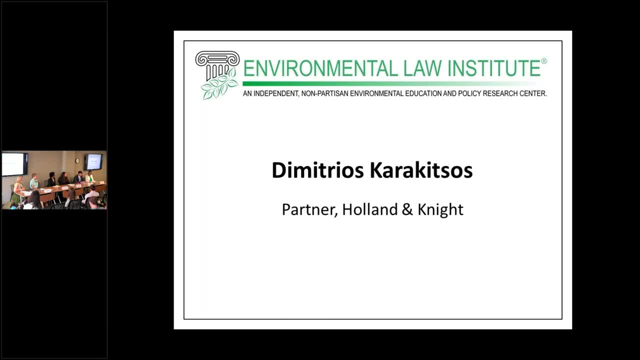 So got to work on kind of a lot of diverse really cool issues. But going back to, what took up most of my time was really the chemical portfolio and TSCA reform. For those of you who don't know TSCA or the Toxic Substances Control Act. 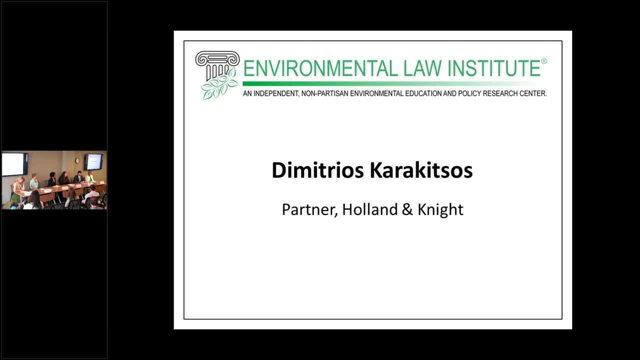 is a law from 1976 that was designed to regulate chemicals and commerce in the United States And that covers everything. I mean just about everything in this room is in some way, shape or form, touched by chemistry. They had kind of very high hopes. 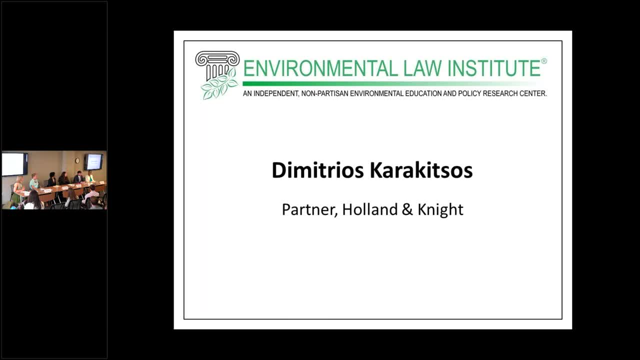 when that law was first enacted By 1990, it's kind of the greatest example used by folks of its failure, and it failed for a number of reasons. But by 1990, EPA's ban of asbestos was struck down in court and EPA largely didn't use the law. 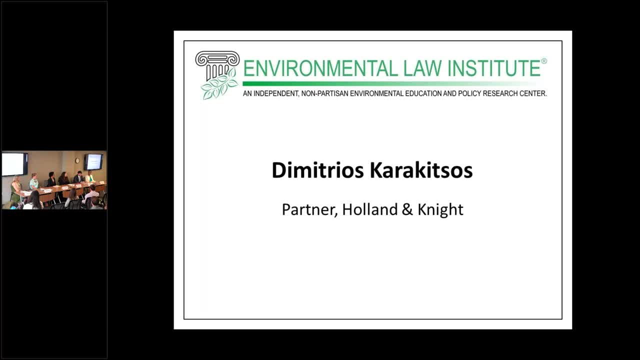 to regulate chemicals from 1990 on. So it was, you know. it got to the point where it was a. it was a big failure. It was the only major environmental law that had not been rewritten or significantly updated since its inception. 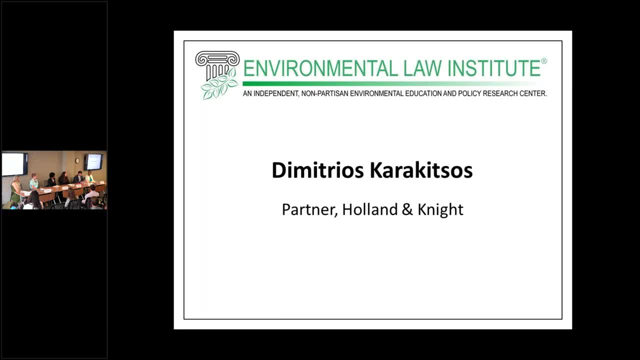 You know I mentioned before, obviously the environmental space and politics can be very polarizing, but this was a really, really rare opportunity to work on an environmental law that was viewed on both sides of the aisle and by a really diverse coalition of people is broken. 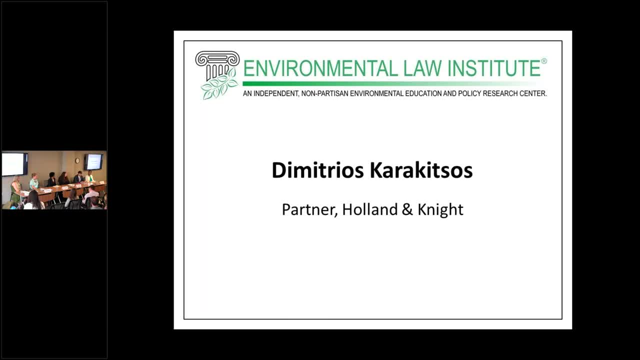 I think it's safe to say Democrats, environmentalists, public health advocates felt it wasn't doing its job. It wasn't protecting human health and the environment from potentially hazardous or dangerous chemical exposures. I think certainly there wasn't disagreement on the right that it wasn't doing what it was intended to do originally. 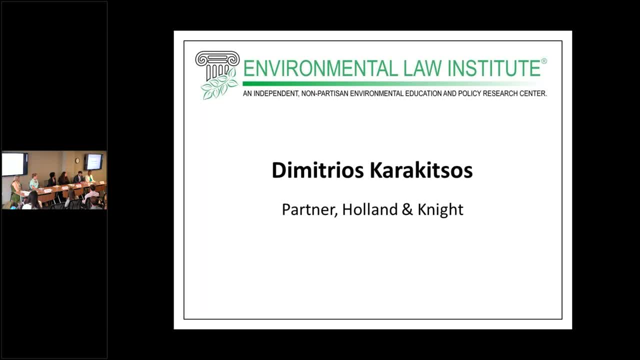 but there was also kind of a business perspective that the failure of a federal system was resulting in kind of a patchwork of state regulations. So you had states like where my boss is from, Oklahoma didn't have the money, didn't have the resources. 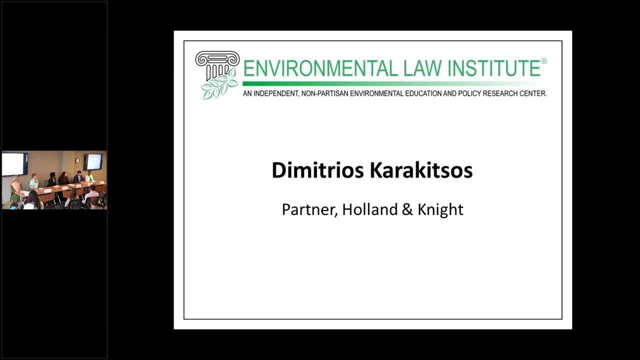 didn't have the ability internally to regulate chemicals, So their citizens didn't have any protections. You had states like California and New York, the more progressive, larger states who had money resources. but we heard from a lot of those states, in private conversations too, that we don't want to be in the 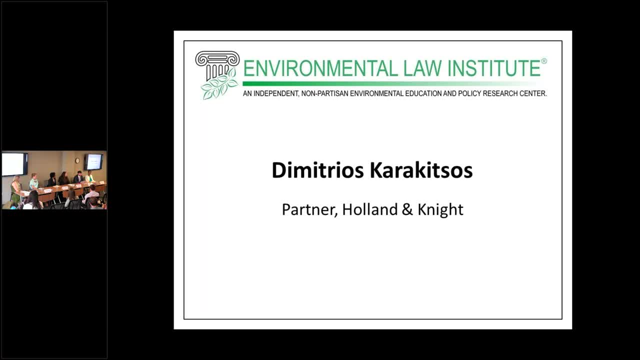 public and private space to be doing this. it's better for a national standard to protect citizens everywhere, certainly from a business perspective. you can't make cleaning products, can't make, you know, furniture, you can't. you can't make the plastic that's in the National Geographic globe 50 different ways. 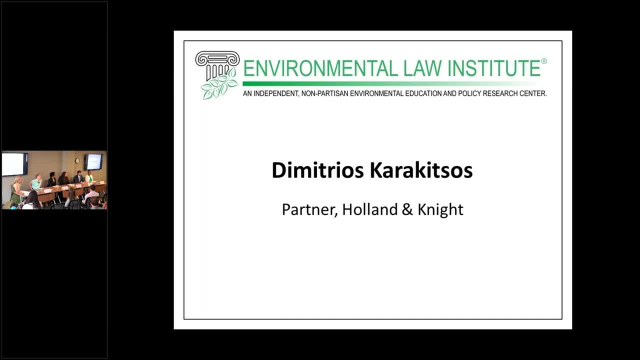 for 50 different states, right, you have to have kind of uniformity there, and so because of this kind of bipartisan desire to fix this law and to have kind of a strong national standard, you know things started moving a lot more than folks originally thought they were going to. so, Senator, 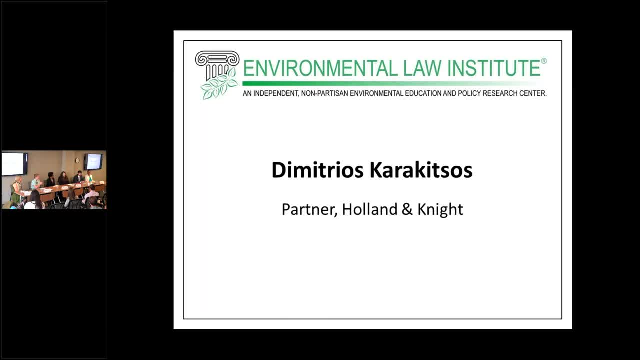 Lautenberg came to Center in off and originally asked for stakeholder meetings at a staff level. we got those together and notice that there was a little bit more common ground once you got folks into a room and and not on their talking points, but actually talking about. 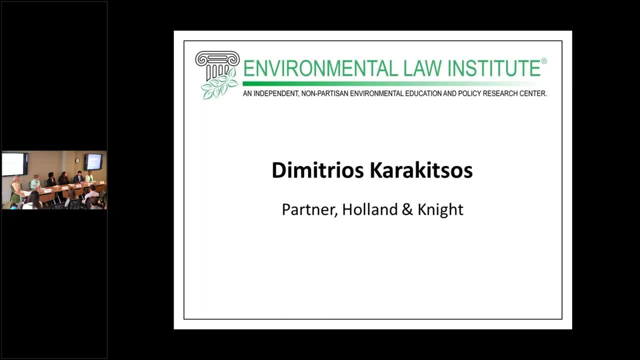 the issues and possible solutions, then we had thought at that point we had. you know, senator, bitter from Louisiana really got involved, primarily because of Louisiana is such a major chemical producing state. it was a very, very long soap opera of chaos for best, the best way I can describe it from there. there was a whole lot of ups and downs, but 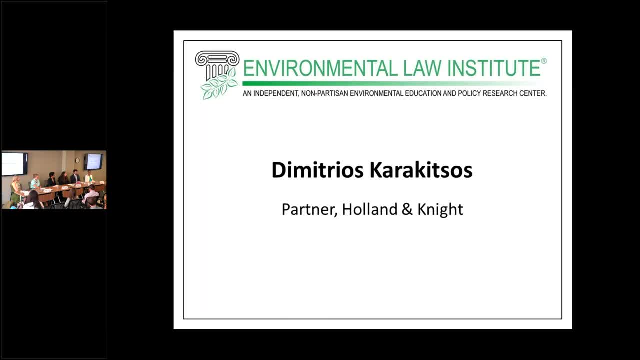 to sum it up very succinctly: Senator Lautenberg unfortunately passed away soon after the bill was introduced. from there, we had co-sponsors turning on the bill. we had you know NGO groups who would call me and say how great this was and how much they supported the bill and publicly trash. 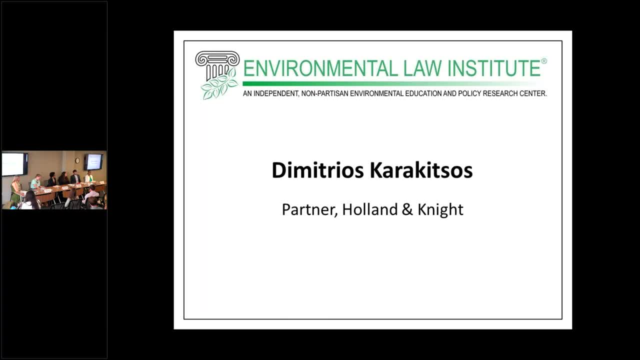 the bill we had. you know, luckily for us, Senator Udall, from New Mexico, who is is a staunch environmentalist from a very staunch environmentalist family going back generations, really stepped up to take the reins of the bill on the Democratic side. um, in part because New Mexico is a state like Oklahoma that doesn't have the money, the 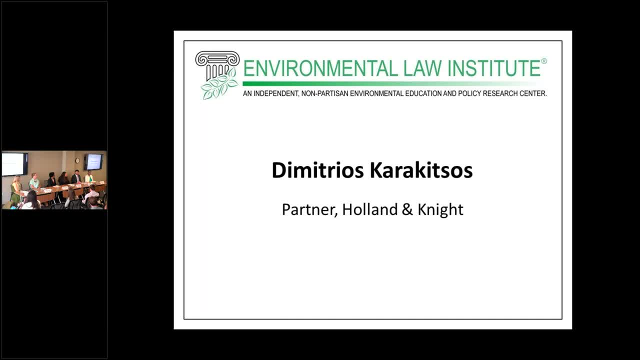 resources, was never going to get the protections that California could provide its citizens, or um that New York could, and saw the need for a strong National standard. um, in addition to Senator Udall stepping up the, the passing Senator Lombard also brought forth, uh, the stepping up of Senator boxer, who was then the chairwoman of the committee. 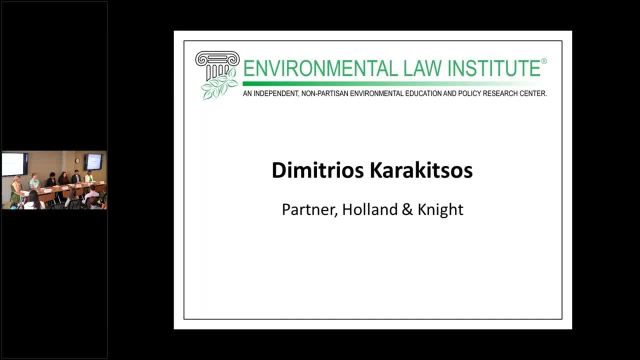 um from California, as the staunchest opponent of the bill. and that's not the chairman of the committee, is not you want, opposing the bill that you're working on. so that's a very kind of formidable person to be against. uh, you know, fast forward after years and years of work. 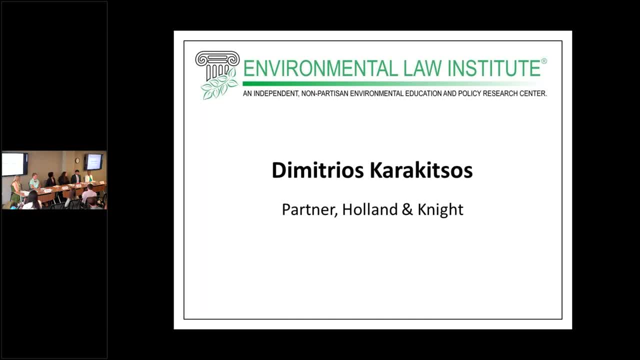 we got a bill that had strong bipartisan support. the house passed at 403 to 12.. pretty historic for a major environmental law. the Senate passed it by voice vote, which means nobody objected enough to even have their vote recorded as a no and you had a Republican House and a Republican Senate. 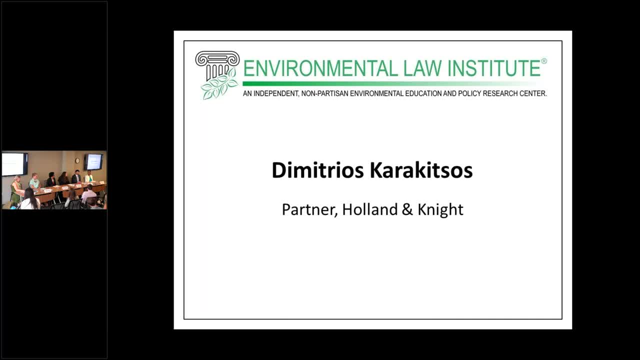 sending an environmental bill that in June of 2016, President Obama signed, had a signing ceremony for and was very proud of. so you know that was kind of the the biggest project I worked on in my career. that was absolutely exhilarating, was an incredible experience. it was also exhausting and 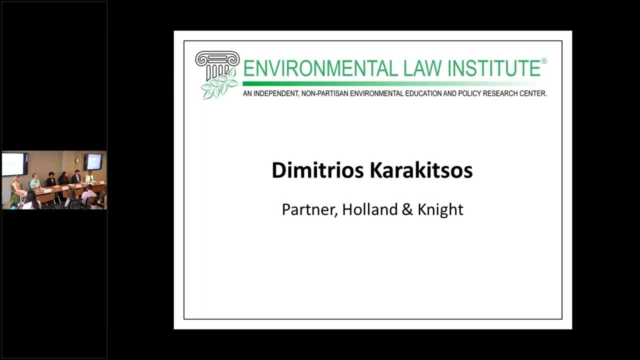 having worked on a big project like that, to go back to some of the politics and other things you have to deal with when you're on a hill didn't seem all that appealing to me. so that's when I decided to leave and join Holland. tonight I've 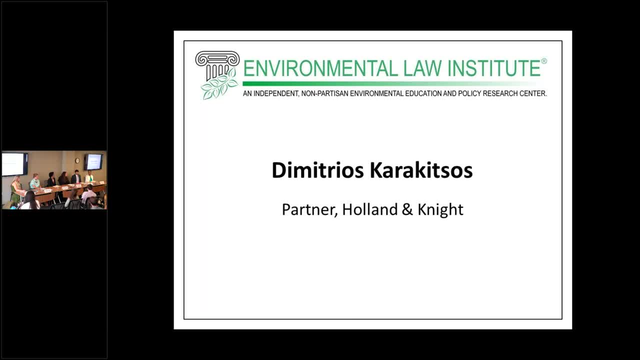 been there for about a year and a half now. today I work in the public policy and regulatory group, which is about a bipartisan group of about 90 professionals spread across the country. it's a very, very diverse group of folks from. we've got folks who were in 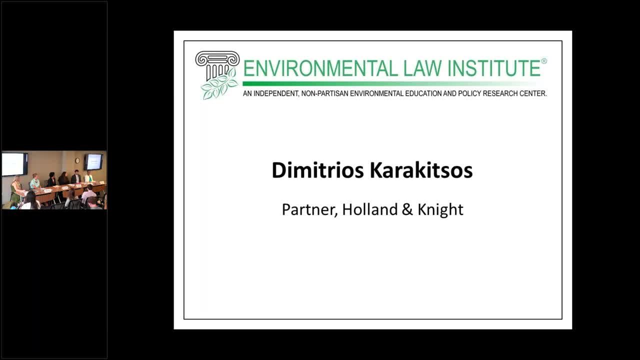 President Clinton's EPA, we have, you know, somebody who was President Clinton and Gore's primary climate change advisor, and then we have Trump campaign. so it's just completely across the spectrum. I would say what I do now is not too dissimilar from what I did when I was in the Senate. you're always kind of working. 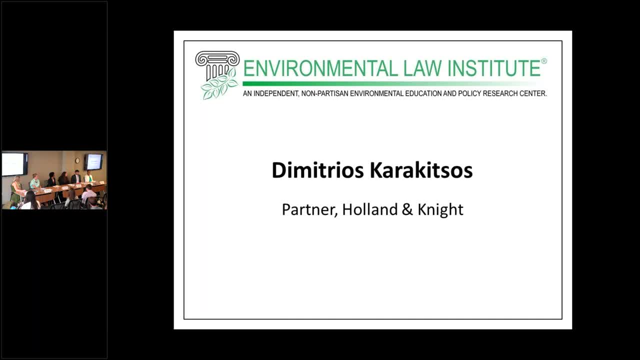 with people to try to solve problems. you're always kind of working with people to try to solve problems. strategize how to best achieve goals, identify issues, kind of key players. who's for and against your position? you know that doesn't always mean. one thing is setting realistic expectations as well. that doesn't, you know, identifying a. 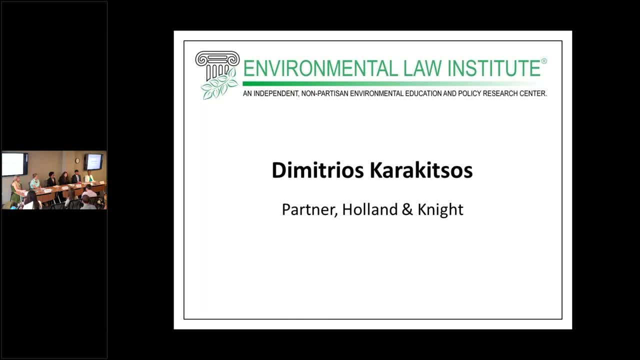 goal doesn't mean identifying a way to advance the ball. sometimes it's not seeing too much ground. I mean depending on the politics and where things are. you know, one thing I loved about my job in the Senate- I continue to love line about my job today- is that there's never really a dull moment and I work on so. 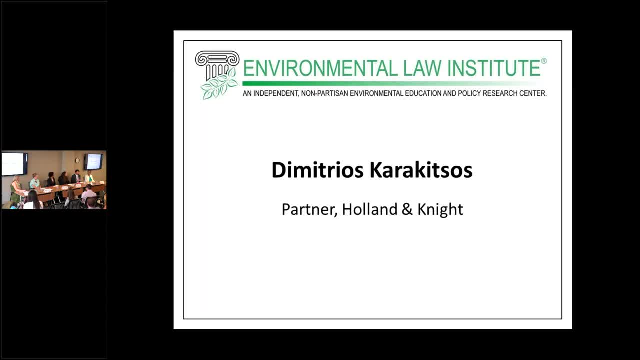 many diverse issues. I don't go in and do one thing every day. you know, one minute I could be working on task implementation. the next minute could be, you know, super fun sites, fuel economy, standards, I mean you name it. there's just a huge diversity in those issues. 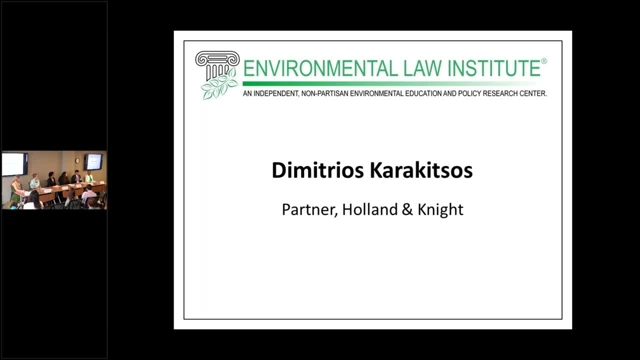 and also in who you work with. in government I get to work with the house, with members of the house, with members of Senate, with the administration, particularly the White House and EPA- quite a bit. I think it's not easy working in an environment where staff and members are turning over, so 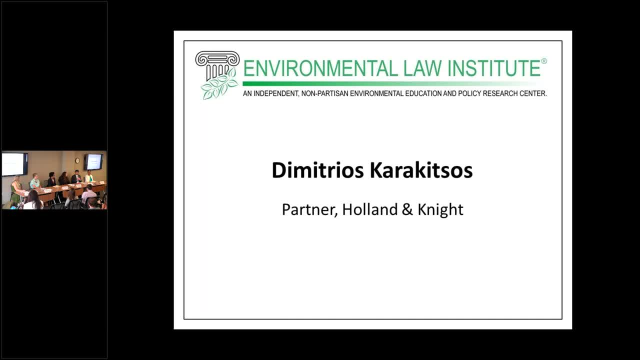 frequently you have staff who gain kind of knowledge and experience on issues and then leave to go work on the outside, leave to go to the administration and other offices. so you're constantly dealing with changes there. you also have politics interjected at every layer of all of. 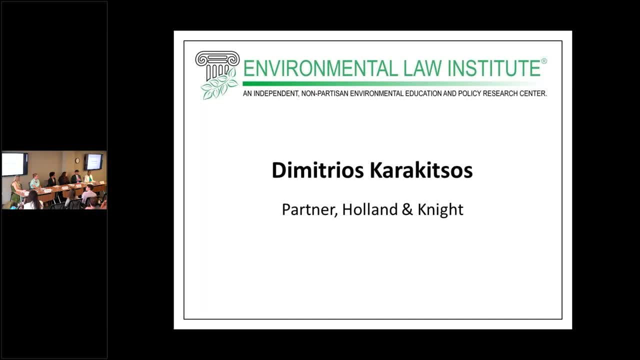 this right. so even if you have consistency, you have folks in the house. we're running for reelection every two years in the Senate, every six the White House. as we know from this election and previous elections, I mean it makes a big difference in this town kind of who is in charge of the executive branch, not 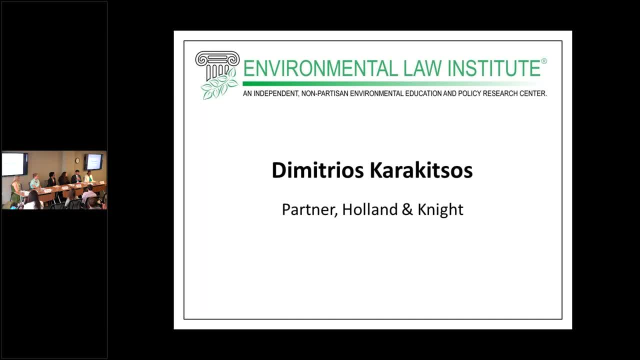 only kind of shaping debate of issues but implementing policies through the federal agencies. Frequent challenge you see in this space is not just how to get results but how to get lasting results. You can have executive orders and you can have things that kind of patch over problems. 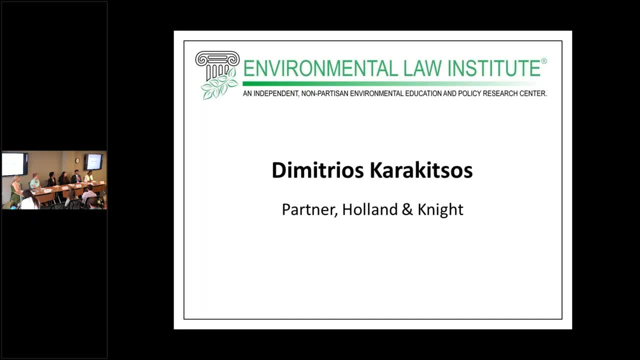 or can solve things temporarily but can be undone very easily. So what you want, if you can, is really to get a regulatory or statutory fix that's more lasting. You know, I think, overall, what I learned and what made me kind of passionate about the 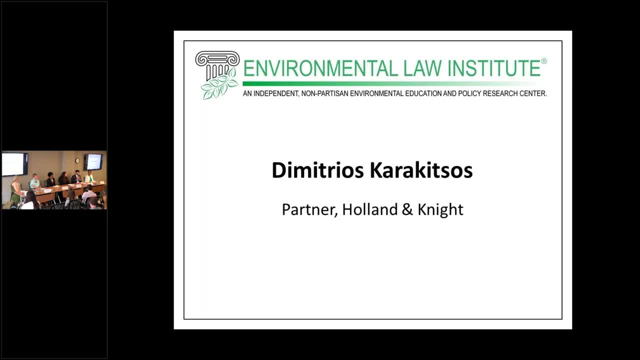 environmental law space is. it's important not only to the environment and public health, but to basically our standard of living and our economy. Everything, I think, requires a very appropriate balance. We obviously need clean air and clean water, but we need jobs too. 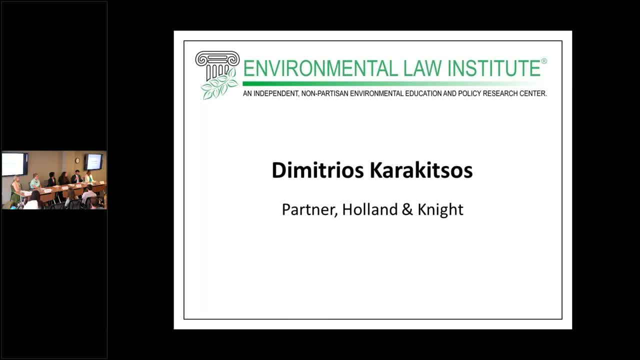 We need cars, we need factories to make all the things that we rely on day to day, But again, it's got to be done in a very responsible way. So you have to find that appropriate balance and cut through a lot of the politics that 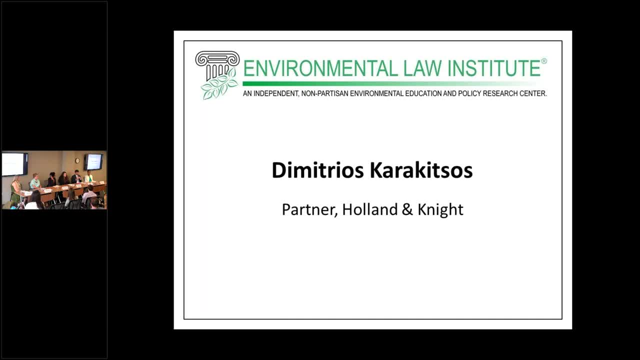 we deal with. You know you hear a lot of rhetoric. You often deal with arguments that don't make a lot of sense or are not based in facts or common sense in DC. but it's kind of trying to cut through that and get to. you know. 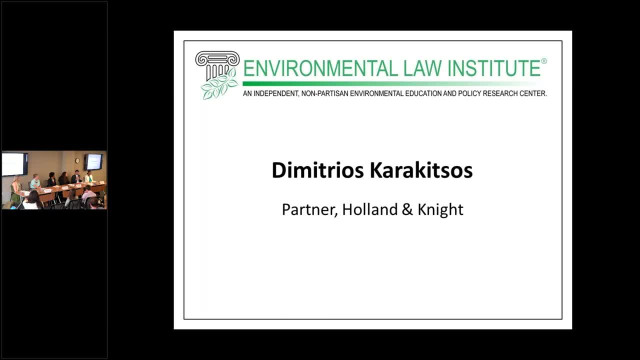 real, achievable results that I've tried to focus on both in the Senate and now in private practice. You know it is difficult trying to work in an increasingly polarized environment on very polarizing issues but, you know, trying to find consensus, I think, is why a lot of us 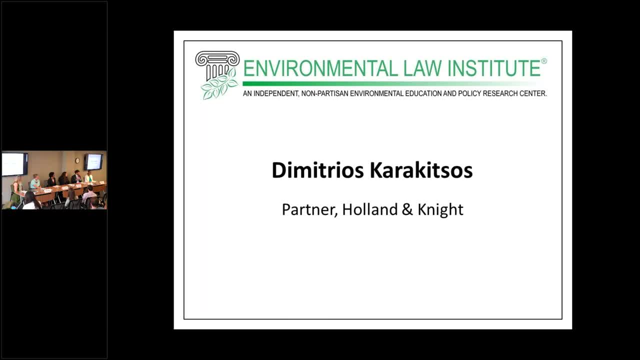 are here and have passion about the space, So I look forward to taking questions when we get there. I don't know about you all, but I'm sitting here feeling really inspired and I've learned so much today. I just want to thank you. 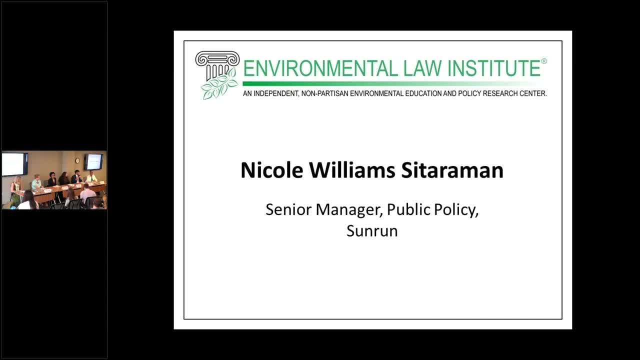 Thank you. I want to thank ELI and Caitlin for inviting me to participate in today's kickoff session for your Summer Educational Series. My name is Nicole Cedar-Rahman and I am a senior manager of public policy for a company called Sunrun. 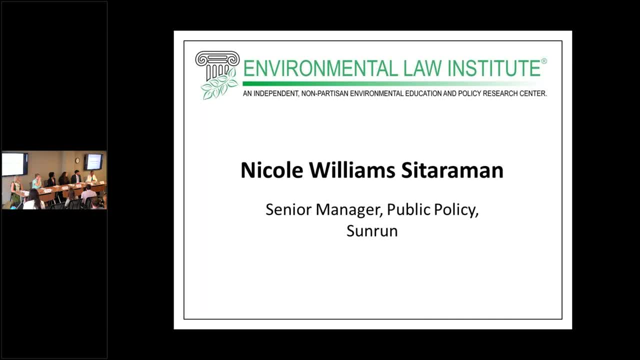 Sunrun is the largest residential solar plus storage company in the country and I'm focused on representation. I'm representing the company's interests in the mid-Atlantic region, both our legislative initiatives as well as our regulatory initiatives. So mid-Atlantic meaning DC, Pennsylvania, Maryland, New Jersey and Delaware. 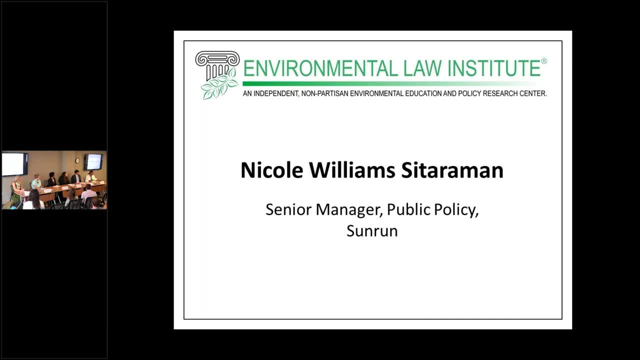 So just to take multiple steps back to share a little bit about my path to working in, you know, the solar industry, solar plus storage industry. my path is quite winding But there are kind of common threads that I'm excited to share with you. 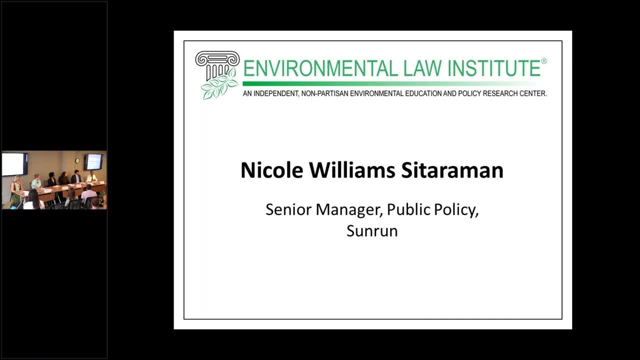 So I am originally from Philadelphia, grew up in the 80s low-income background, grew up in the Germantown section of Philadelphia And had a single-parent household. I was born and raised in Philadelphia. I was born and raised in Philadelphia. 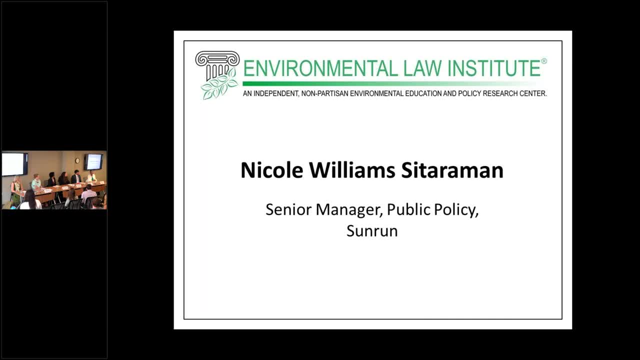 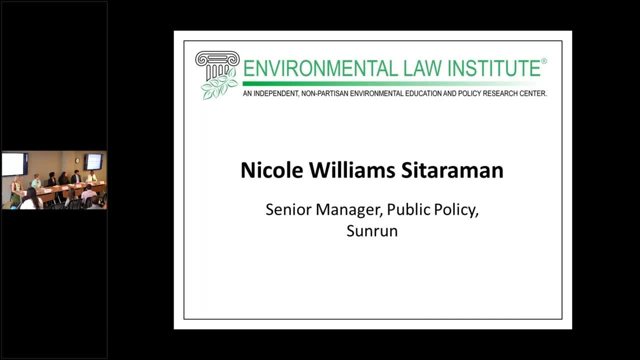 PhD in optics of all things, kind of very specific. But we've had as a family a kind of a really challenged pathway to upward mobility and getting out of poverty And you know we've had a lot of challenges over the last couple of years. 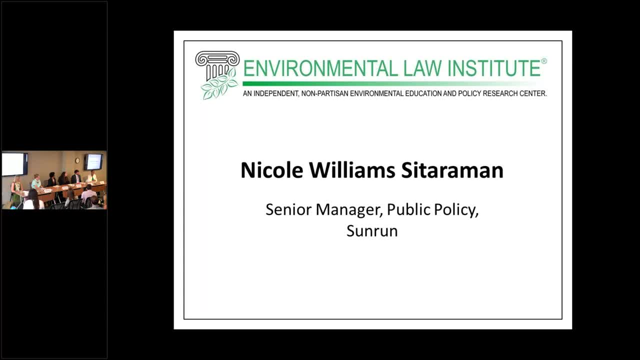 I had a mother that I've been very grateful to have, because she was a great really, because we were on welfare for much of my childhood- But I had a really resourceful and passionate mother who was passionate about education And she knew that that was our ticket out of the challenges that we were facing coming up. 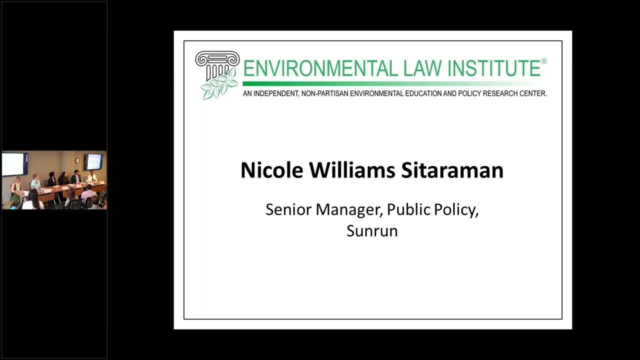 The challenges of low income communities and the experience of African-Americans in an urban America And so that that experience really has informed my, my much of my path in my career and in my life. So I got it when I was 10. I got a scholarship- community scholarship- to go to Germantown Friends School. 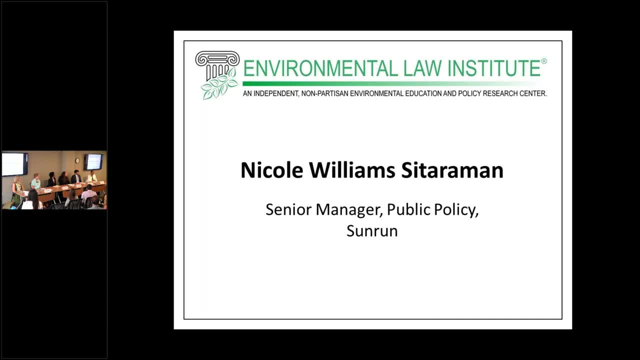 which is a Quaker school in Philadelphia, And I went to Germantown Friends between fifth grade all the way up through 12th grade. During that era, you know, a lot of things were happening nationally and locally in our in our region that really left a major impact on me. 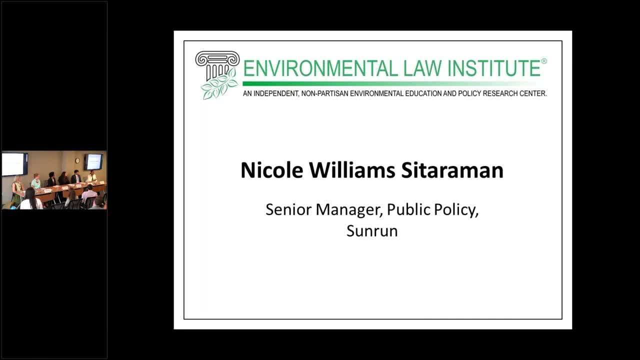 and a strong desire to pursue civil rights as a as a career. So the LA riots happened in 1992.. Philadelphia had its own challenges with a lot of kind of static and troubled relations between African-American community and the Jewish community. A lot of things happen like in the 80s. 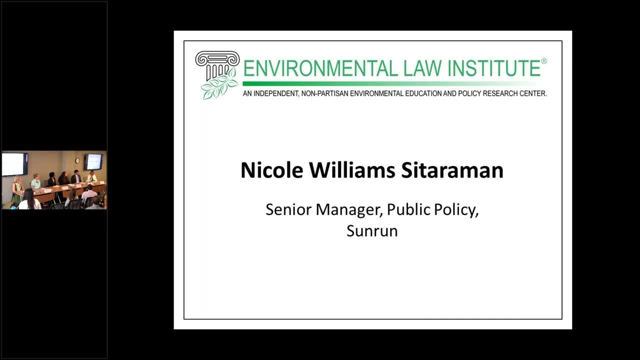 Mayor Wilson Goode, a Democrat, did like a horrendous thing. He dropped a bomb. So really, just this is an other thing. there, New York City, There was a kind of alternative cultural group called Move. They were living on Oursage Avenue in West Philadelphia. 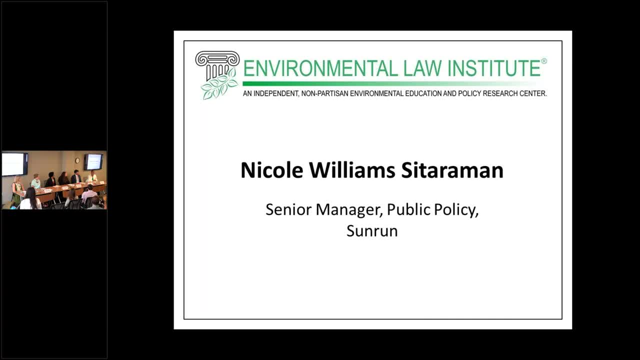 And I guess the community was very upset about their alternative lifestyle And there was a huge battle between police and this group And sparked a strong interest in human rights and civil rights. When I was 17,, I participated in a program called Operation Understanding. 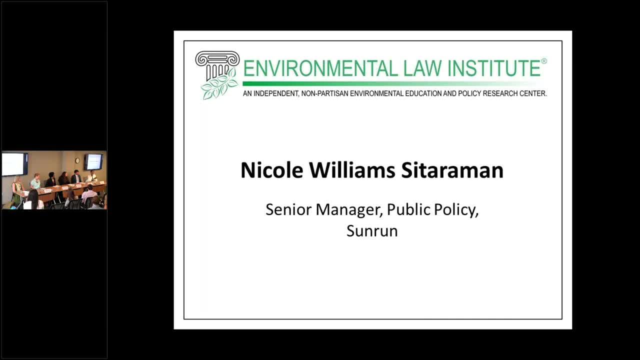 which is for juniors in high school in Philadelphia, African American and Jewish students, to come together and go on a trip to Israel and Senegal, And just for a little over a month we traveled together and talked about actually the history of our collaboration between. 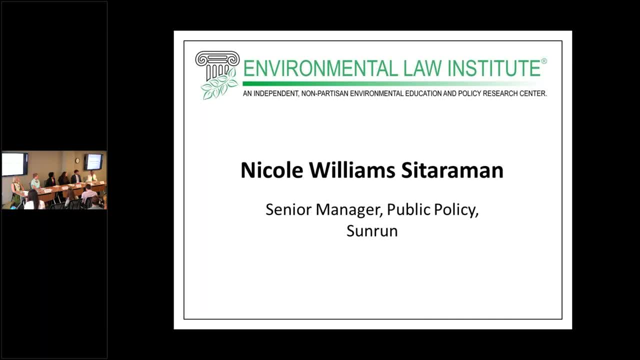 our communities on civil rights issues And the experience was just amazing. I mean, I had never been out of the country- I was 16 or 17.. And the conversations that we had about our experiences as two communities- some very common experiences of oppression and also working. 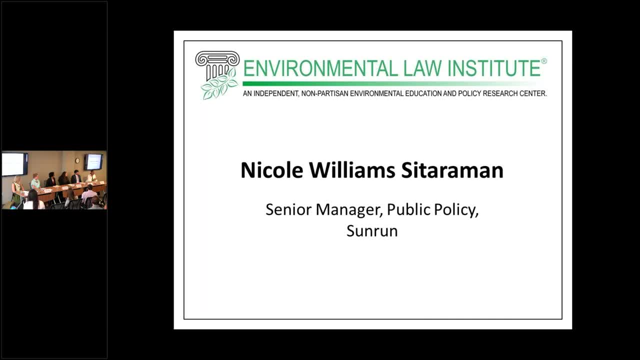 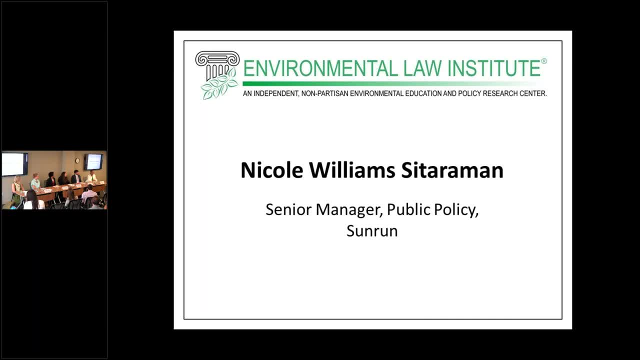 and 70s. You know, just really it was just a wonderful kind of moment for me and really helped me. you know, just continue my my focus on on these issues. So I let's see after high school. 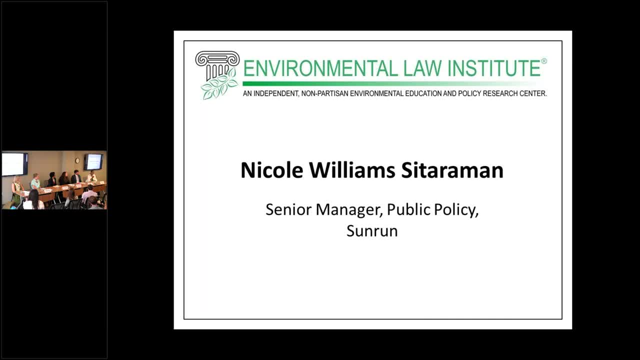 I went to Yale University. I'm the first gen went to Yale University And you would think that my experience as a first generation college student at Yale would be kind of hard and difficult, But I actually found that experience to be really enriching. I met so many other students who were 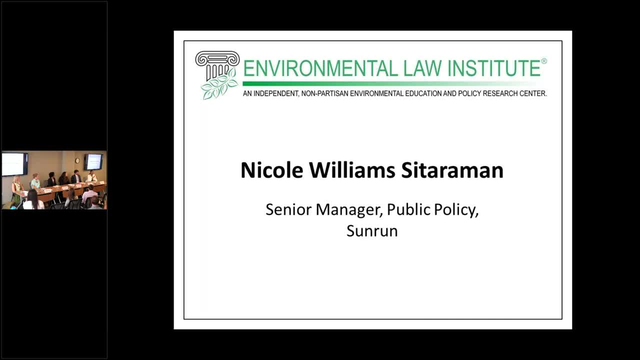 first gen going to college, coming from low income backgrounds. like one of my closest friends from college was from Appalachia, We hung out all the time. I met so many other students there who had shared experiences of coming up with very difficult, difficult circumstances and kind of overcoming obstacles and things like that and having an interest in 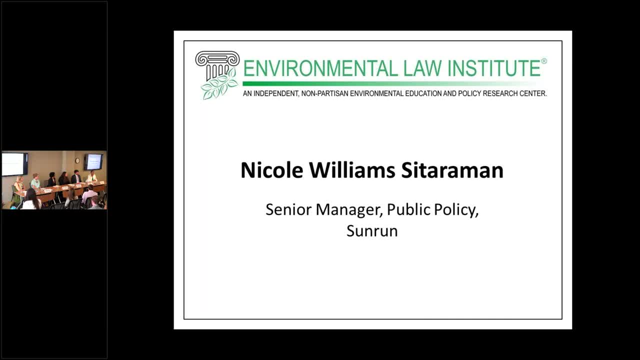 working in fields that that really helped people overcome poverty and racism. So Yale was a wonderful place. I met my lifelong friends there. We're still my friends today, A lot of them living in DC area, which is funny. so I'm working in policy So and during my college experience, you know I didn't do anything related to the 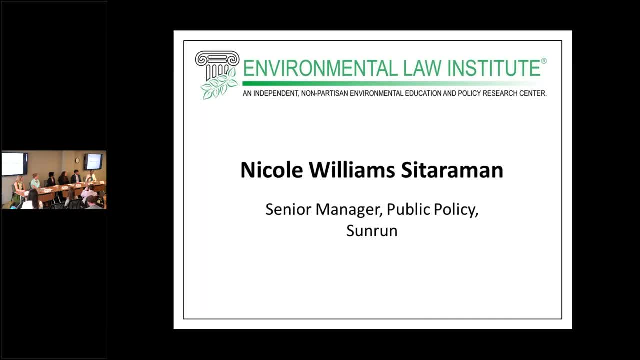 environment. actually in college, That's a theme that I'm hearing on this panel. Like I, it was certainly. I went to a Quaker school. the Quakers love some nature. I mean, they took us to campus every year And you know I developed an interest in. 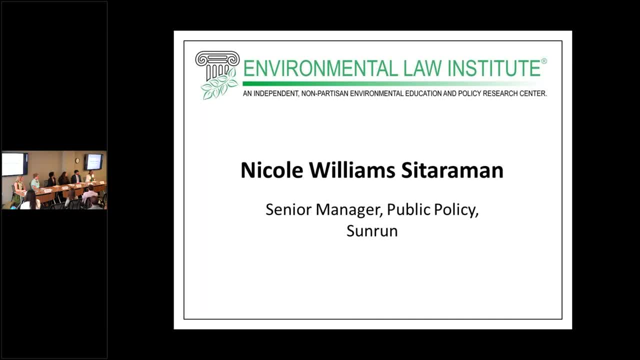 camping and things like that and appreciation for nature, but not really a focus like I'm going to work on, you know, environmental issues or I'm going to work on clean energy policy. That just really wasn't a part of my mindset just yet at that. 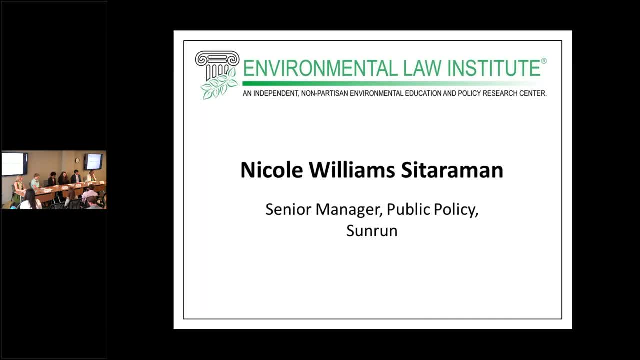 time. But you know, during college I had various opportunities to just expand on the interest in human rights at a couple of fellowships: traveled to the Netherlands, traveled to Copenhagen, did a lot in the area of human rights And I got a fellowship after graduating from college to work here at the Center for Law and Social Policy on. it was post welfare reform, So prime. 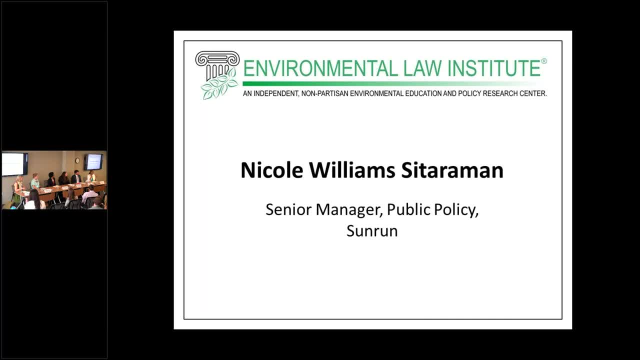 time for a lot of policy wants to, you know, figure things out. So I came here for a year to do a fellowship And that organization really introduced me to the sometimes the mind numbing and boring and very challenging experience of working on policy issues. I mean, it really is kind of, you know, chipping away at at a huge mountain frequently and it's not. 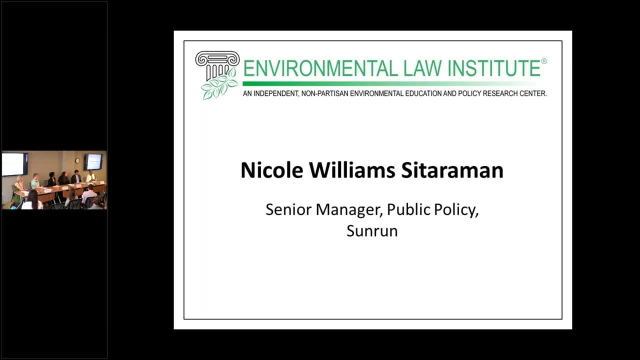 glamorous and it's not. you know, it doesn't feel like you're part of society. And then of course there was group work and social counseling, training and job networking opportunities, And so that's kind of where I got my tips and, you know, just started my career. 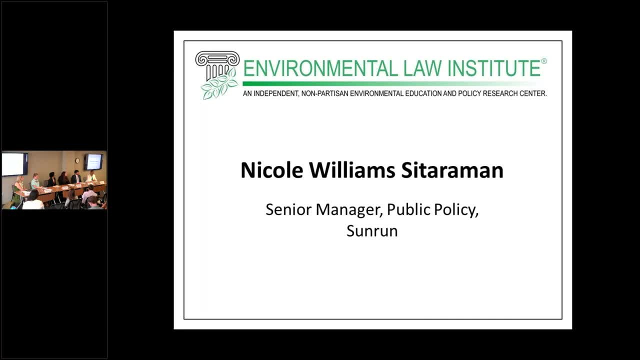 And I think it was. Yeah, that's really cool to hear this. This is one of the stories came about because I'll jump right in. I you know this is a сделали yes show, feel good all the time. it feels some frequently that you're, you're not really. 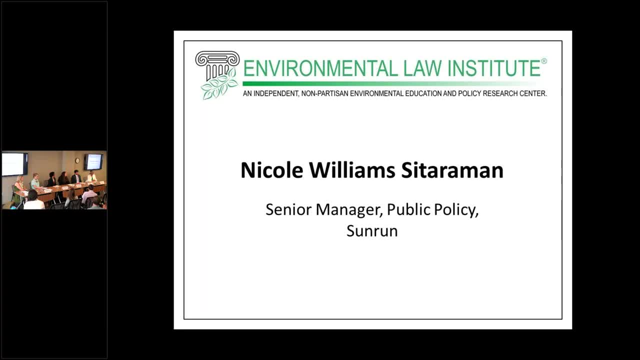 making much progress, but what I learned from that experience was really the importance of staying the course. when, when you don't get that instant gratification on issues that you're working on, I'm just really staying focused and staying connected with a community of professionals who are 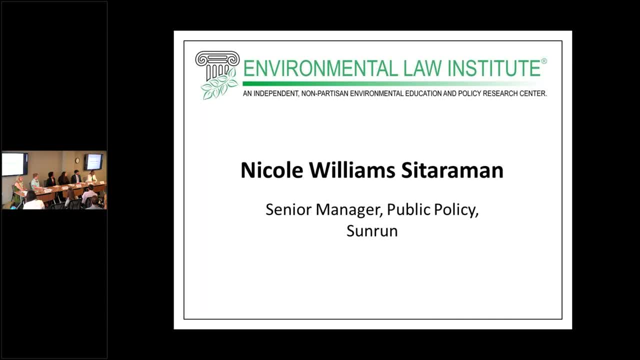 like-minded and equally passionate about moving the ball forward on the issue that you're concerned about. I had deferred when I graduated from Yale, deferred law school for a year. so after the Center for Law and Social Policy, I went to law school at Boston University and, candidly, you know, I never took an. 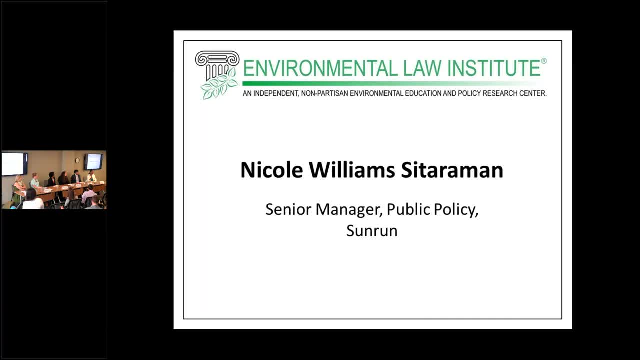 energy class ever took an environmental environmental law class. I- that really wasn't wasn't on my radar either- was very passionate about human rights issues, civil rights. I took those types of classes where I felt like I was really empowered and came to life and really excited about being in law school. 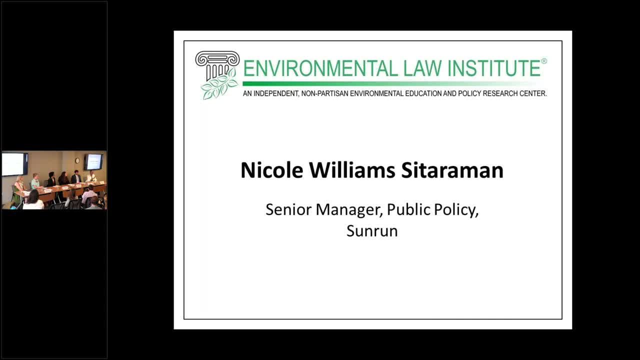 because the first year was horrible. I could not stand it. let's just keep it real. the first year of law school was really, really just felt so unnatural and so detached from from what really drove my passion. the Socratic method, I just felt, was just so antiquated and purposeless and you know, I just it just was not a fun. 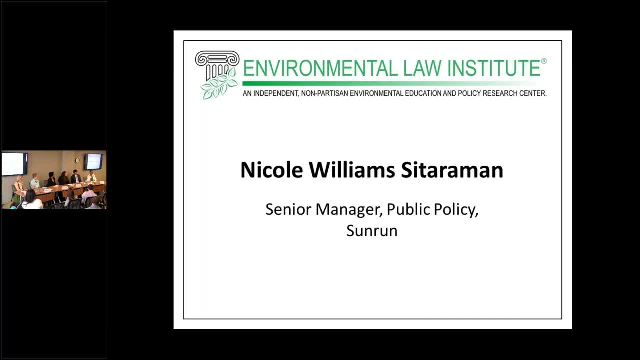 experience for me second and third year. I had more fun because I felt like I had more control over the classes that I could take and I also did clinic in addition to doing a lot of writing. so clinic I felt for for those here in the room who may be in law school on the phone or participating remotely. I I 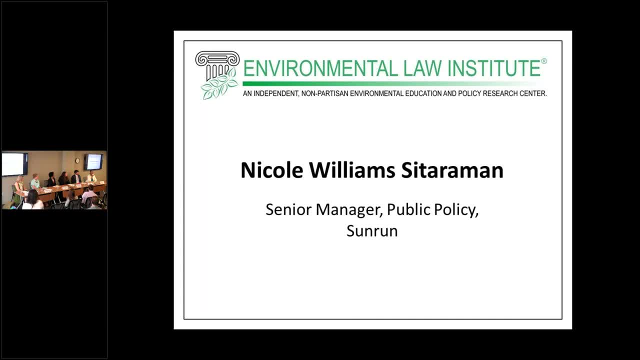 believe that clinic is a really important training experience that you can get. so a lot of law schools now have environmental law clinics or environmental justice clinics. I highly recommend that you do that in addition to journal and- and you know, moot court and things like that. but really getting 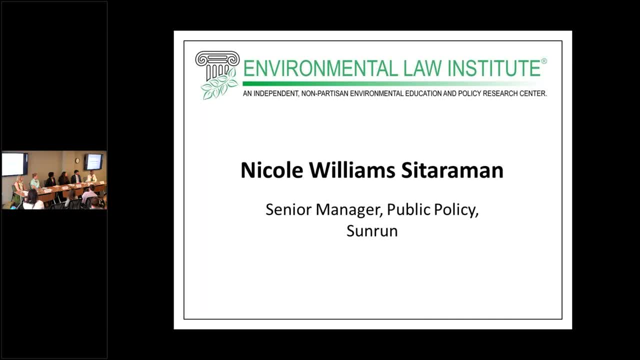 some practice. learning by doing is where I felt like I was able to get a lot of experience. so I felt like I had the most fun and I learned the most, rather than just sitting in a class or in a seminar and kind of you know, taking notes and I 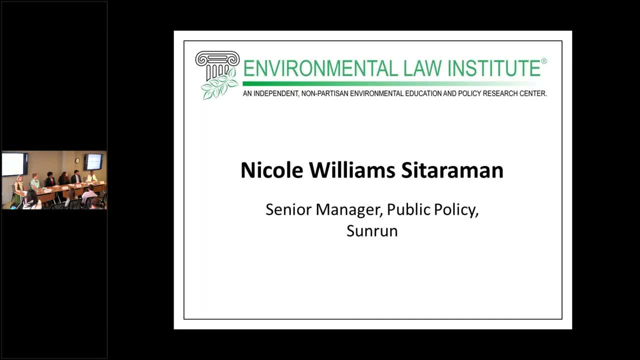 I find that for me, clinic and really being actively engaged in helping people, even as a student, was the most valuable for me. so I, after law school, I got a job. after law school, I got a job at a law school in the United States and I got an. 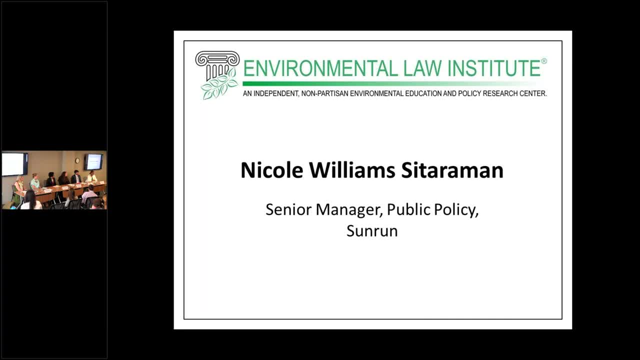 at a large firm because i had some loans to try to pay down. that's another reality that you know. people kind of dance around but law school is very expensive, as are, you know, most graduate programs very expensive when you don't come from a family that you know has wealth build up for generations. 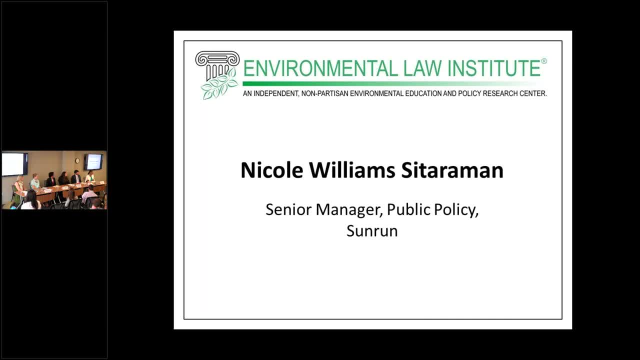 you're kind of caring, not only yourself, but sometimes you're carrying your family members as well, um, and you know you have to make certain decisions to to to make sure everybody's okay and you're okay with sally may, um, so i, so i worked for a large firm in philadelphia, um um for two. 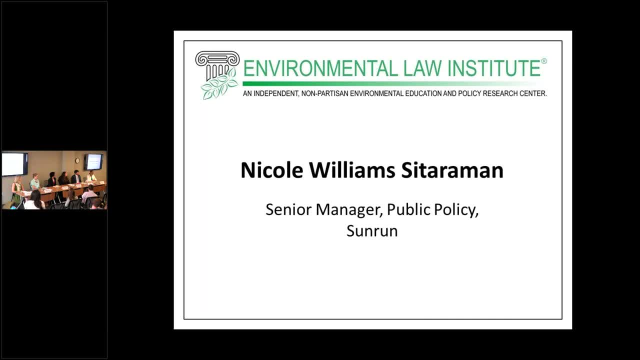 years and it was fine it was. you know, i worked in the litigation division as an associate and was paid well and was able to, to, uh, make put a little dent in my debt. um, but then you know, i just kept the the passion going. so while i was an associate i volunteered. 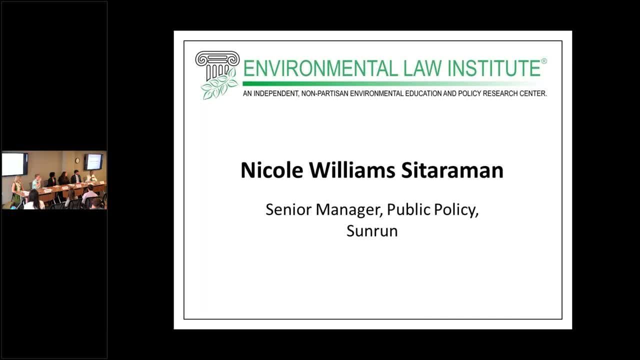 um with a variety of organizations in philadelphia maintain the activism kind of passion that's in me and um maintain relationships with um key mentors both in philadelphia and here in dc. i want to pause there. that it's really important on your path, even if it's a winding road to. 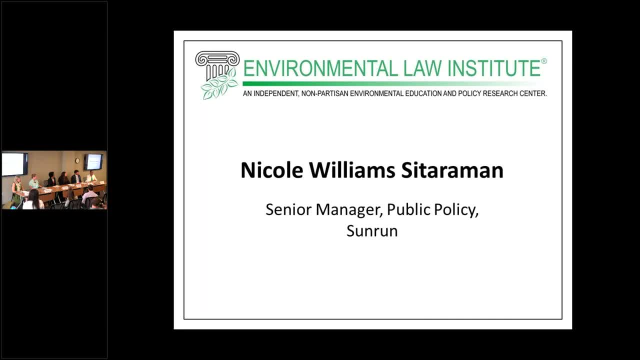 getting where you're eventually going to go with environmental law or energy policy, to keep alive um with um, either- whether it's professors or employers, folks in the community, who you're, who you're connected with professional organizations- um maintain those relationships. be, be intentional about um keeping in touch with folks, because people remember that um and they'll. 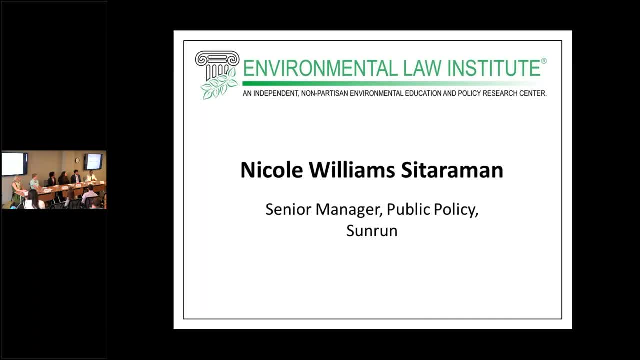 they'll keep you in mind when their openings um for good opportunities, for good positions. um, it's the old-fashioned just, you know, be friendly. you know those who. what's the scripture? you know, he who has friends must make himself friendly. you know, um, it's a really kind of um, old-fashioned. 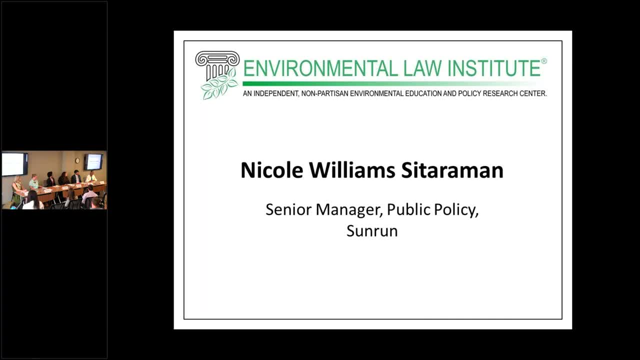 kind of um principle, but it definitely applies throughout um your career, um, so, um, so again. so while i was at the firm i i just maintained certain relationships and dialogue with folks um, and i just decided to leave after two years to come back to dc, because i love dc so much. dc is such a um. you know, people focus on the federal 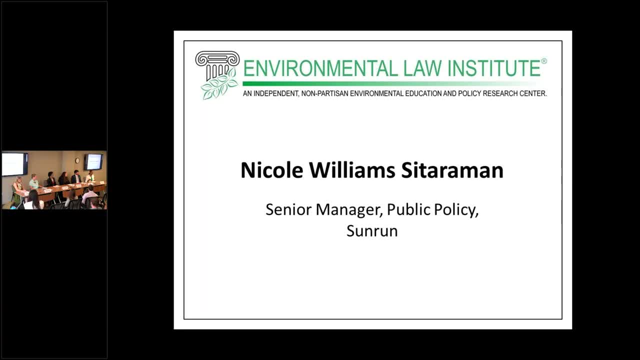 side of um the excitement that happens here, um in dc, but there's a lot happening locally in all eight wards in the district of columbia um around a variety of really critical issues affecting everyone's lives. so, um, it's just a wonderful diverse community here and i just i love washington. 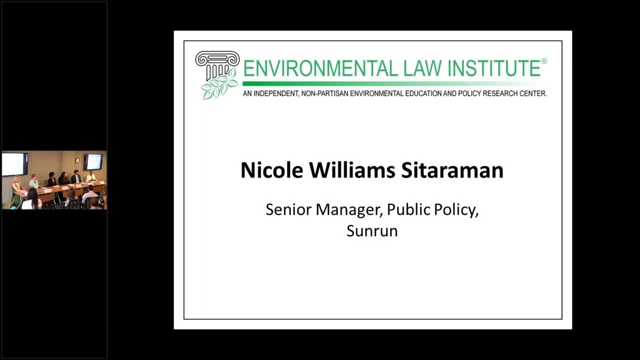 as much as i love philadelphia, um, so i came back here, um, and i got a great job at um a law firm here. civil rights litigation law firm very um. very aggressive plaintiffs. uh. employment law firm focused on um representing employees who felt that they've been discriminated against. whether. 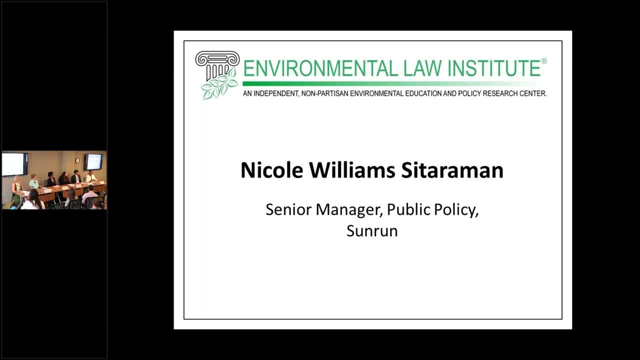 because of race, sexual orientation, whether they have been sexually harassed, um if they're going by a cycle ettling, or whether they have been uh under arson charges, or whether they've been charged with sexual assault or has been charged with perjury or um increased amount of prostitution, or uh um greater amount of sexual assault. um i just 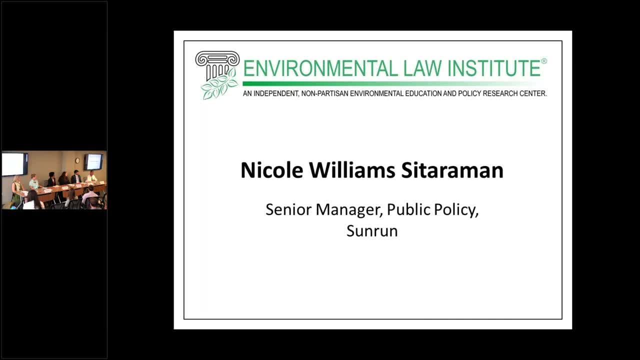 think it's just incredible- and i'm not sure i have the words, but it's um, i'm- it's hard to describe it- have a voice, have a seat at the table, and that they really brought to life the importance of everybody having a lawyer in employment situations. that that go. 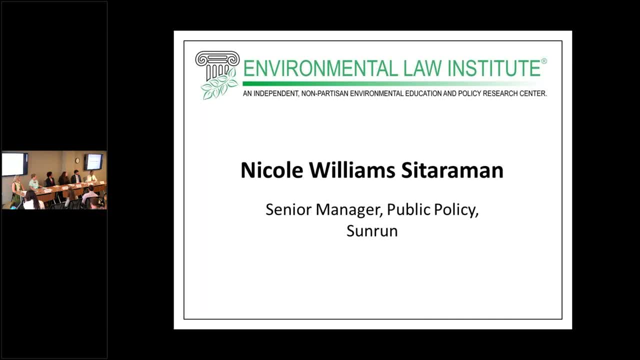 wrong. not everyone has the ability to get a lawyer. but you know, I really enjoyed that experience, really developed my persuasive writing skills again. this is kind of a very basic skill set that will carry you very far in your career if you can really kind of find your voice when you're writing. how many folks 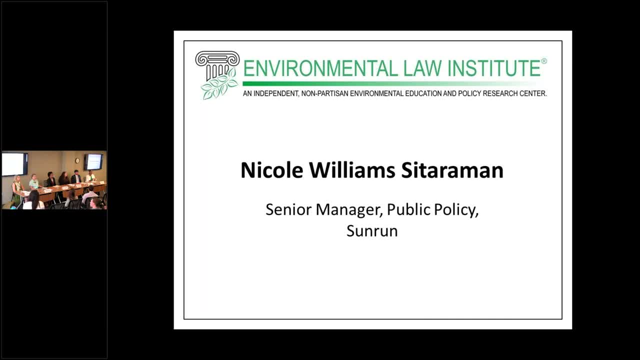 are in law school here, okay. so in law school sometimes you feel that you're kind of forced to write based on a formula for legal writing and there may be a sense that you're losing your creativity or your voice and in the writing process. but working at the firm and working at a, if you can find a good 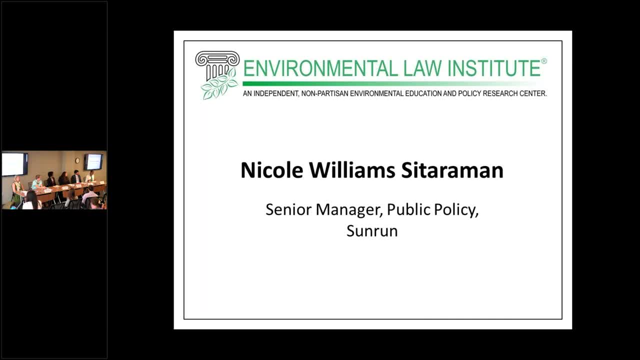 place to work, that where people really nurture your writing and your voice, I can really bring dividends for you, for your career. so this firm, that's what I found and that's what has carried me. I worked there and I represented a couple of whistleblowers at nuclear power plants, at a nameless company in the 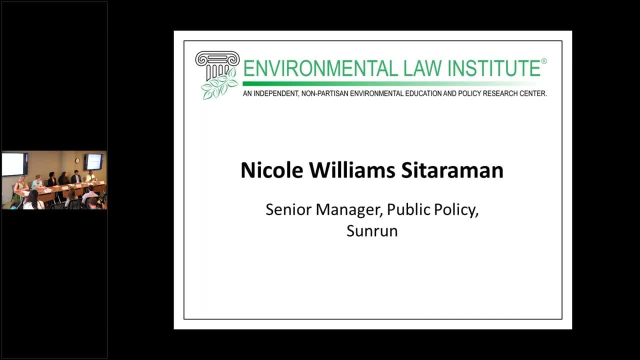 south utility representing employees who complained about public health challenges and the company overlooking some things and were retaliated against because they raised these concerns. and that experience really introduced me to to the impacts of corporations on public health and in the environment. you know, I think it's really important for me to be able to be able to be able to. 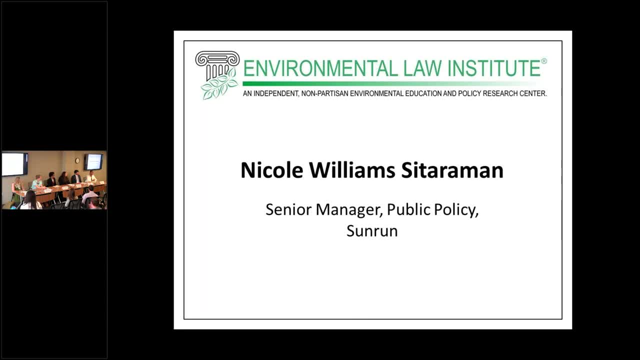 you know, I think it's really important for me to be able to be able to be able diversified in an environment and a lot of different communities. while I was diversified in an environment and a lot of different communities while I was at the firm, I also volunteered with the DC chapters of the Sierra Club and became 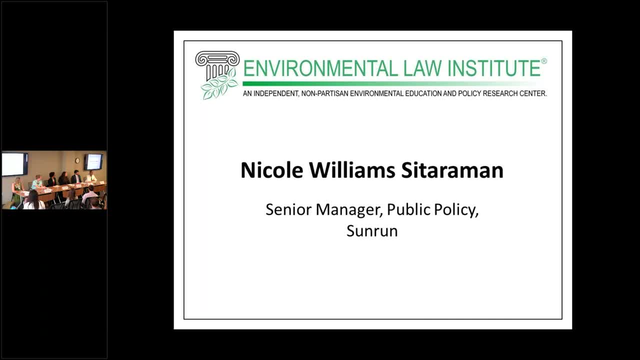 at the firm. I also volunteered with the DC chapters of the Sierra Club and became very active in their energy committee and just developed an interest in merging civil rights with an interest in environmental issues and actually just decided to take the plunge and and jump into energy policy and 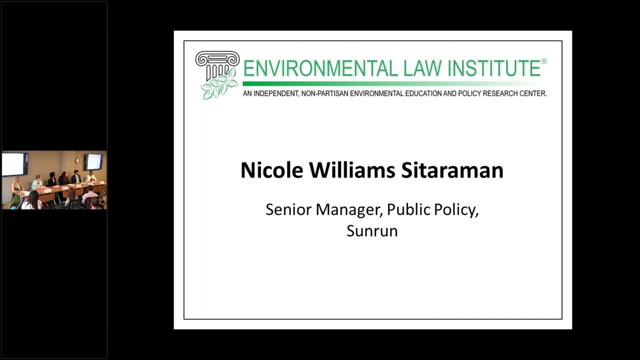 merging my civil rights background with a focus on energy justice issues and make a career shift. the relationships that I established while at both at the firm and at the Sierra Club and at the Center for Law and Social Policy- kind of my worlds- all kind of came together to make that transition easier and that's. 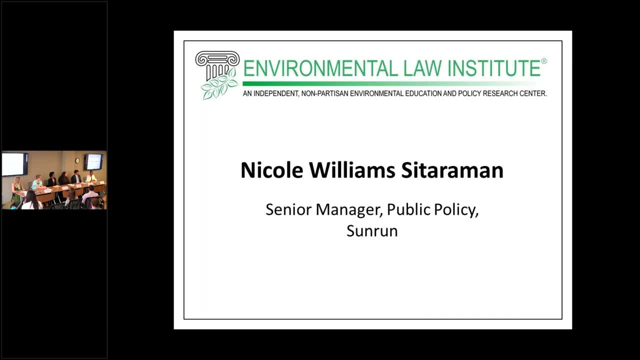 why I emphasized the relationships and through making that shift, I ended up at the DC office of the People's Council, which is the ratepayer advocate for all DC utility consumers, and worked on renewable energy policy for DC, advancing community solar aggressive RPS renewable portfolio standard, which I'm 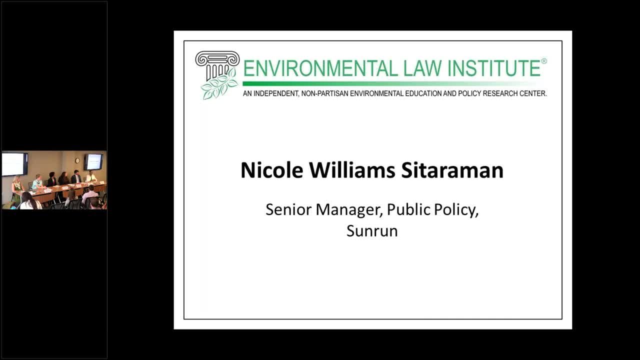 sure you all are experts in focus on renewable energy as a tool for consumer empowerment. specifically, DC is a solar or solar. this is a solar city, not referencing the company, but really focused on expanding access to solar to more consumers. and the People's Council, who I work for, was 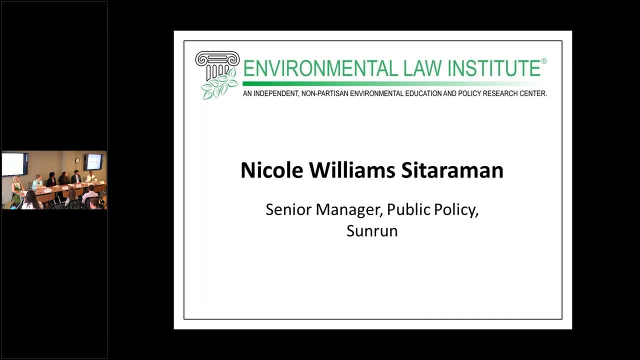 very committed to that, and her role is to look out for all residential and small business consumers and make sure that utility rates are reasonable and just, and so part of that that, that mandate, is to look for options legislatively and before the Public Service Commission to make sure that all consumers have access. 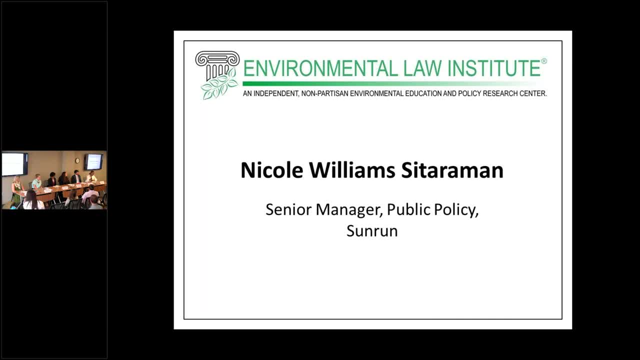 to clean energy, which the city is very committed to. I'll fast forward because I'm I'm rambling, but after several years at OPC I had developed a lot of great relationships. I had done a lot for the city in terms of advocating for great legislation, representing our office at the 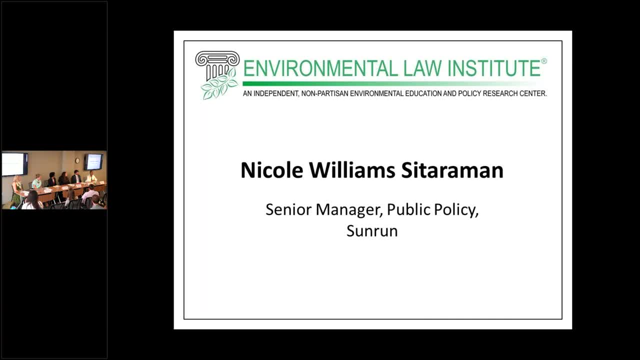 Commission, and so I decided to. someone had tapped me on the shoulder about an opportunity at Sunrun, and so I applied and got the job. so so now I'm representing the solar industry before a variety of regulatory legislative officials and advocating or improved rules and regulations to facilitate consumer access to solar. 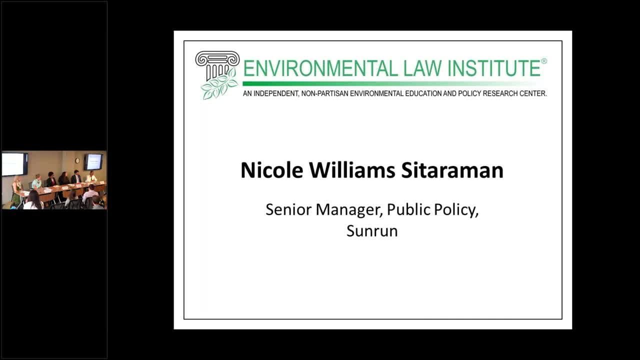 as well as battery storage, And I look forward to the questions. I'm sure there are tons for all of these wonderful panelists, But one of the things that I wanted to end with was you know the focus. my focus has been on kind of consumer rights. 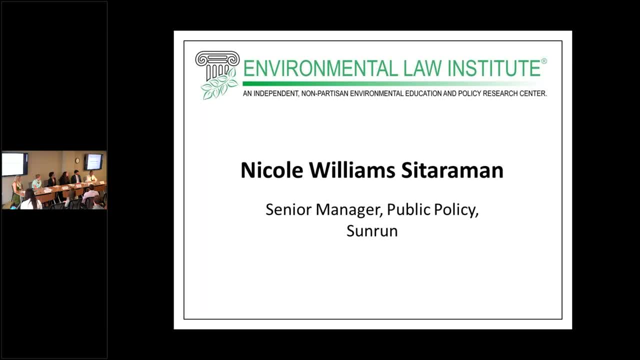 and civil rights and consumer choice And I'm so glad that, Demetrius, you shared that. you know your political affiliation. that's one of the challenges in the clean energy space: that it's way too polarized. The conversation is ridiculously polarized. 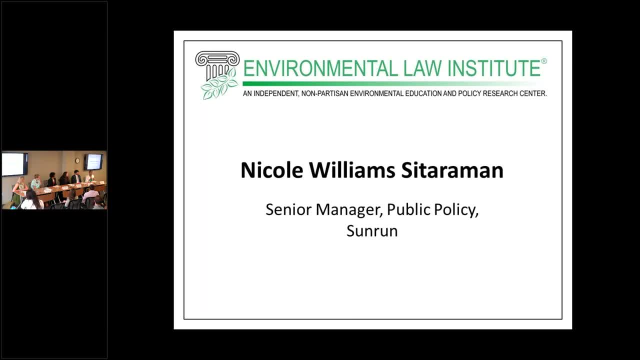 And I would say that you know, one of my closest allies and friends in the clean energy movement is a Republican, an African American Republican, who is very passionate about the consumer choice aspect of bringing on a more kind of solarized energy delivery system. 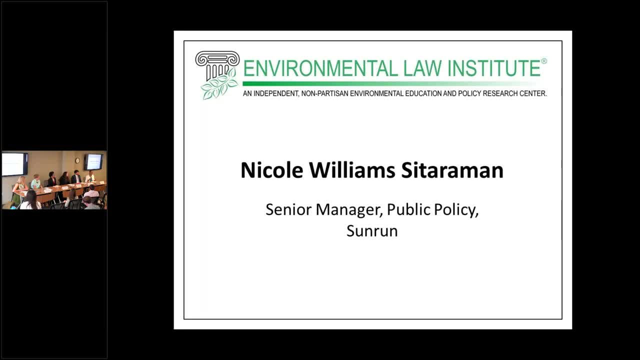 And there's just more that we need more of that, more conversation around the fact that our environment- you know, clean energy- really should not be about your political affiliation. So I'll just end there And thanks for your time, Hey, thank you. 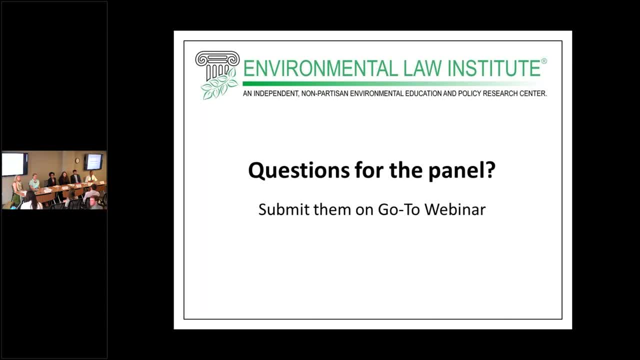 I'd like to start in the room And then again, as a reminder, if you're online, just submit your questions through the questions box on GoTo. Does anyone want to start us out? Thank you, Hi. I'm Ray Matthews. 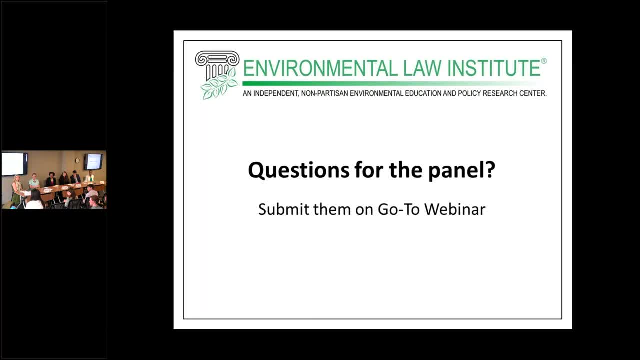 I'm a fellow at USDA and I've been in the agency space at USDA in the park service and the forest service for about three or four years now as a fellow In between times to grad school here in DC for energy policy. So my interest in my undergraduate degree was in agriculture. 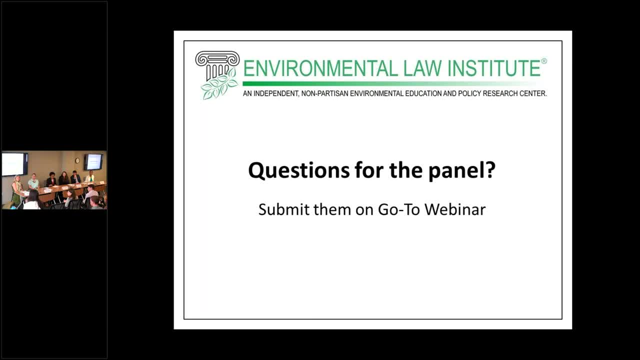 And so I have a huge interest in development, agriculture, environmental policy, environmental justice, energy, And I'm at a hard time. I'm interested in going back to school and get in law school And my questions have been answered pretty much from everybody throughout the panel. 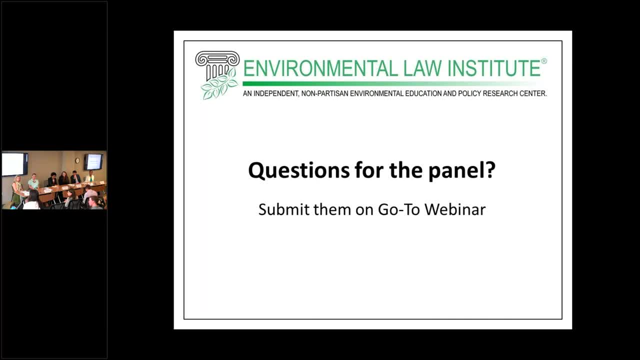 So thank you for that, But I want to see if I can respond. Thank you, I can respond specifically about your experiences in agency or in Congress or in a firm around environmental issues and law and how your experience has been different for those who had those different experiences. 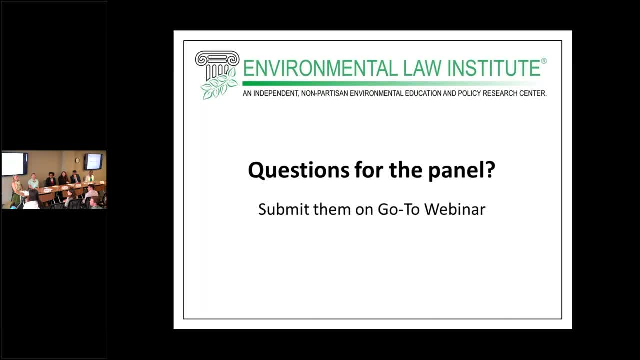 And I think typically Demetrius and Stacey and Nicole. Yeah, I'll try to kick it off and interrupt me if I'm not getting to the point you're looking for. You know, I've had just different experiences really almost day to day in some of the same jobs. 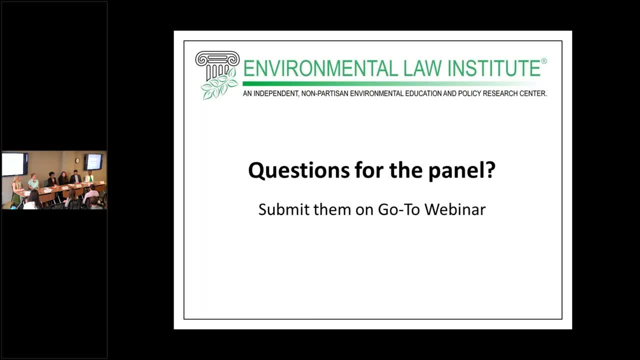 What's important today, particularly in a political world, is not important or as important tomorrow and a new issue kind of overtakes it. So working in congress looks a lot of what's kind of the most important, the issue du jour, and you know what you know. unfortunately, a lot of times like 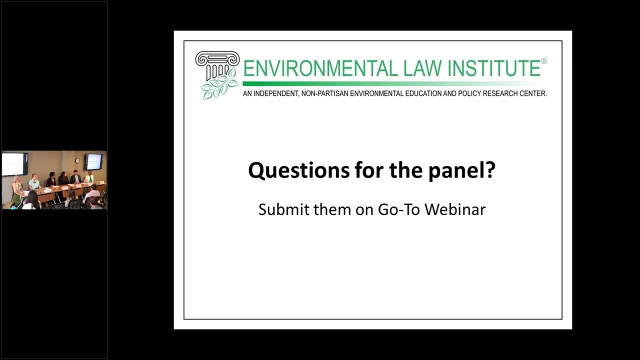 Nicole mentioned it's: what fight are you in? I wish we could do a little bit less of that and I think there's folks interested in doing less of that, But, as you can see, in the country I mean, there's polarization right. 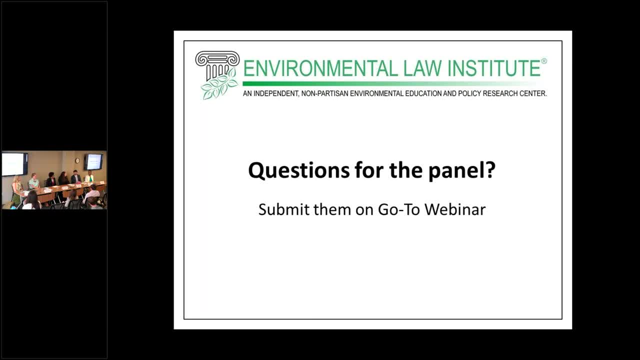 And in order to be here to fight for what you believe in, or what your constituents believe in, you have to get elected and you have to, you know, cater to those bases. I think it's a little more consistent from the outside perspective, because when you 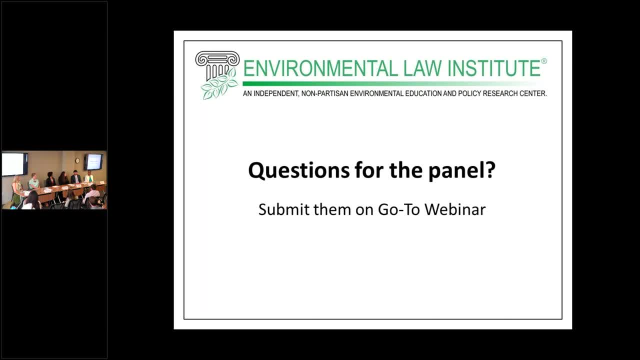 have clients, you're you know whether you work in solar, for oil and gas, for chemicals, for whoever it may be, there is kind of a consistent mission and vision and purpose. So it doesn't matter who's in the White House, doesn't matter who's in the Senate or the 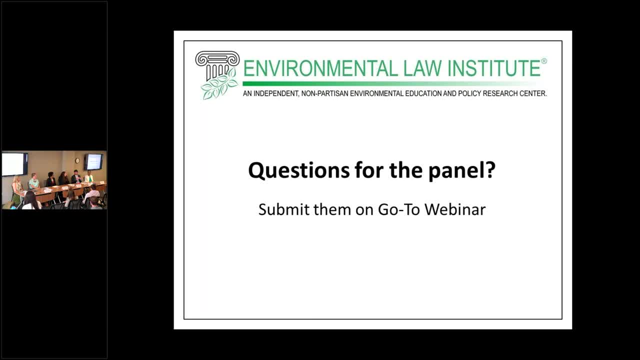 Congress, it doesn't matter what's important, You know, If you're on the front page of the newspaper today, you're kind of moving forward a little bit more with those issues and a little bit more consistency. I think from my experience. 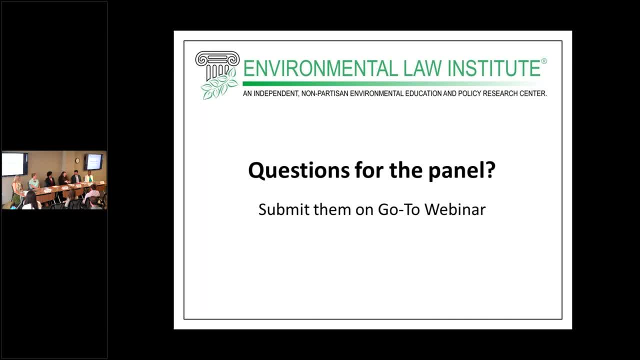 Yeah, and I would sort of actually in some ways echo that, but sort of from the perspective of the agency, where I do think if you're working in the private sector and you know, let's say, at solar, you have your clients or even a nonprofit where you kind of you have. 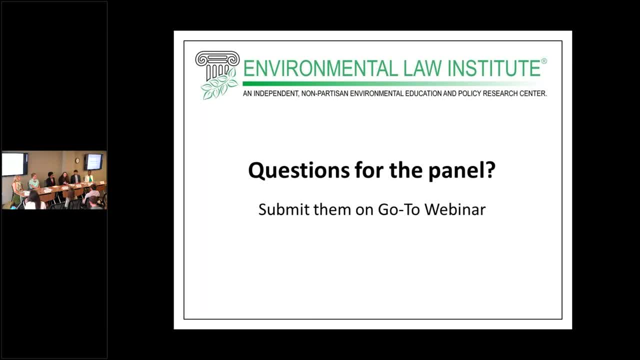 your mission and no matter what's going on, you know you're sticking to that mission. Government is different that way, And I think one of the things I've realized- You know I was basically a law clerk and an intern under the Obama administration and 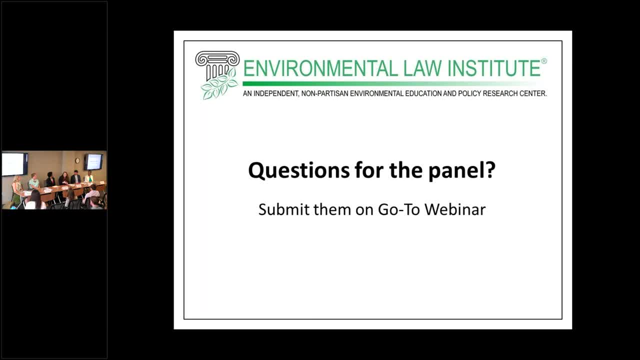 now I'm an employee under the Trump administration and I'm in an office that's independent, so I'm a little bit, you know, insulated from it. But one of the things I have observed is that, you know, there have been radical policy shifts. 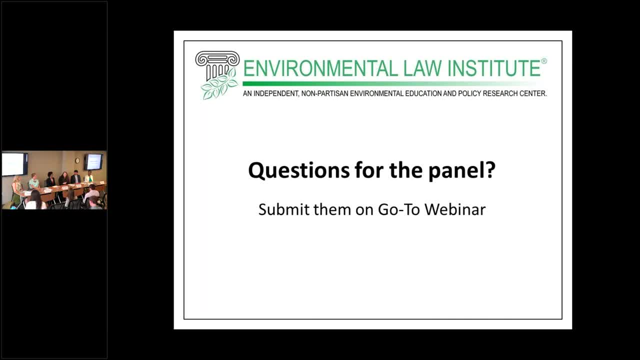 and changes, especially in the environmental space, And so I think one of the things to know, going into it as a career employee is: if you're thinking about this especially for a long term career, am I okay with that? You know, am I comfortable with that? 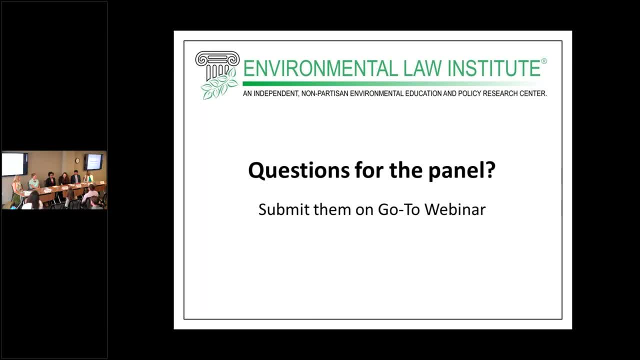 You know what I'm doing today. I might be undoing tomorrow or doing the opposite of it, And am I going to be okay advocating, you know, positions that differ wildly from my personal beliefs? I think that's kind of one of the things to keep in mind. 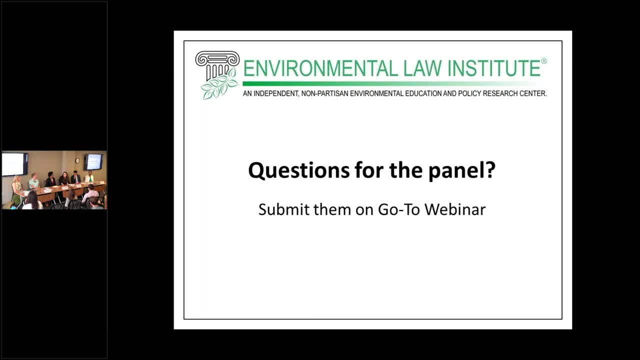 And I think this might be sort of an extreme you know version of what's happening. I think this particular transition from administration to administration has been maybe a little bit more pronounced than others, But I do think that's something to keep in mind. 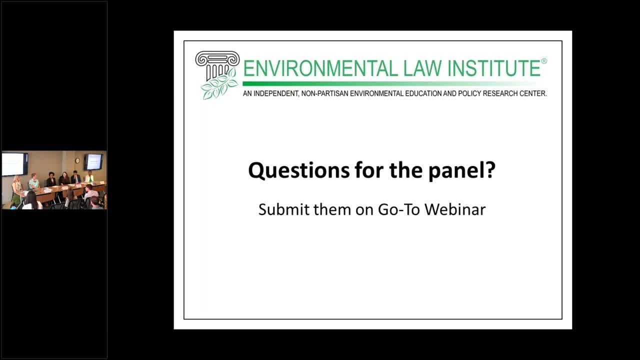 And so you know, if you're looking at, let's say you know USDA and things of that nature- like, well, what are the policies now? Am I okay advocating for those policies? And then you know, if that shifts, am I going to be okay advocating for something different. 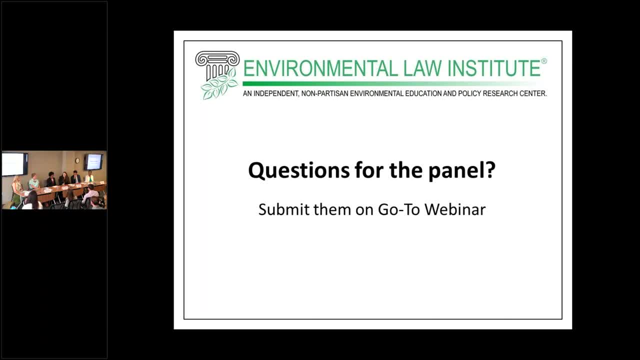 And so to me that's kind of the biggest thing, Yeah, And I think, something that is sort of unique: Of course, if you come to an OIG then you're sort of insulated. so I just- I would just echo what my colleagues just said- 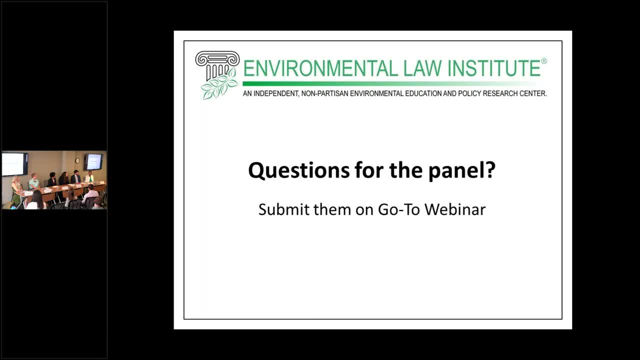 And the theme of being nimble is really critical, particularly in this space. Certainly, you know, Maintaining a close, maintaining your own kind of integrity and sense of purpose and what you want to accomplish, is really critical, but things do change rapidly. 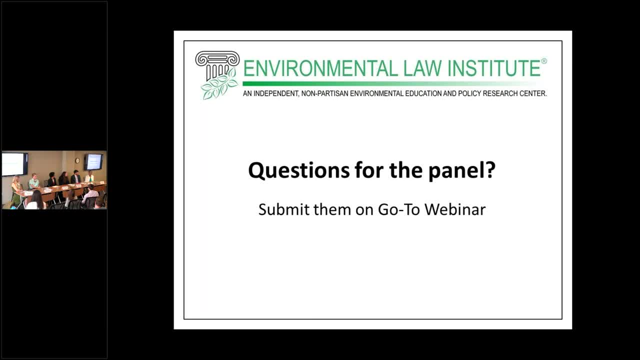 Even within, in my space, within the solar industry, not everybody's always aligned on the path forward and how to, how we want to get more solar to more people. So So being nimble, Being open, Being open to different perspectives as well. 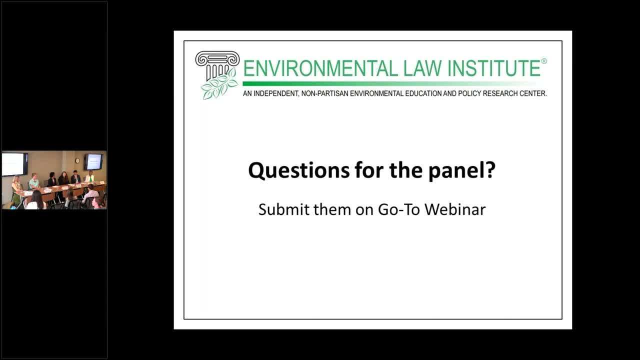 But yeah, That's all. Do we have another question in the room? So I had a question for Colby, Just because your experience sort of seems like it was. you stayed in one organization for a really long time, which is really cool. 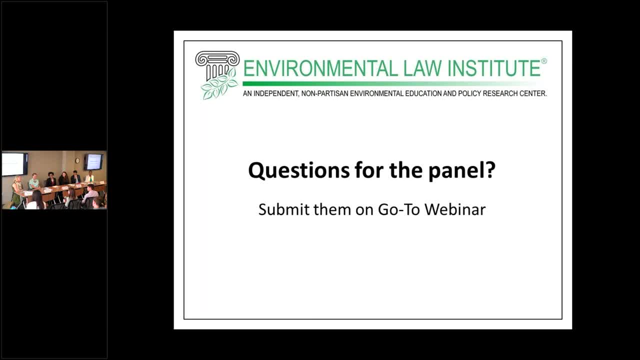 Yeah, And rare, Yeah. So do you see that as like a benefit of your career trajectory And could you just talk a little bit more about how that has impacted? Yeah, Sure, Yeah, Yes, It is very rare, But people I'm not rare at National Geographic. 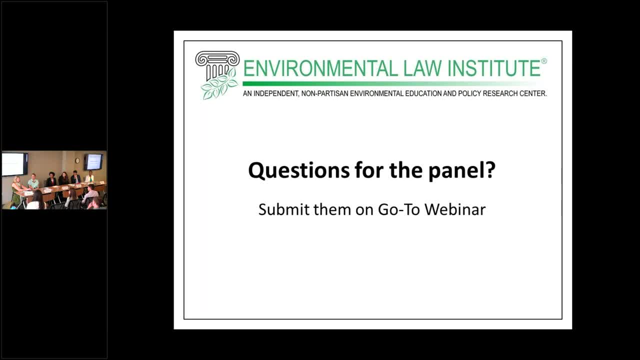 A lot of people have worked there for like 30,, 40 years. I'm, like you know, still. I'm still in the lesser in terms of number of years. So it's a little bit different, I think, when you're kind of working in the bubble. 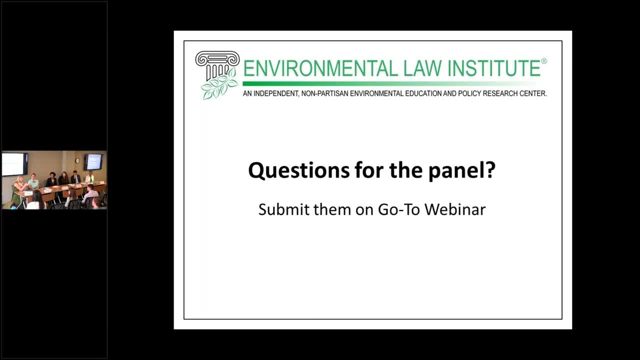 But then when a lot of my friends and you know, just hearing everybody else's career trajectory, you know they're doing the two to three year stints. I think one thing when I went back to school to get my MBA I was kind of like this is: 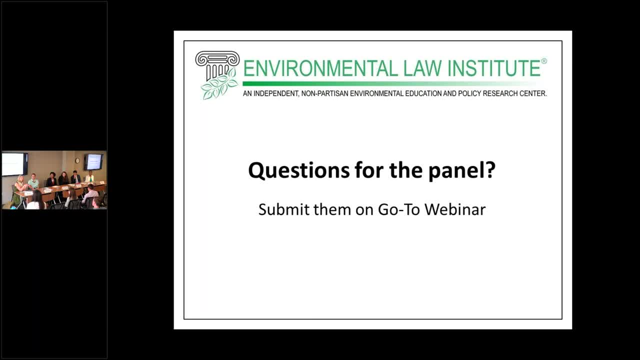 going to be my pivot point out of National Geographic. Maybe I'll do something else. work at a whole profit company, try something else. But because there has been so much change and turnover at National Geographic, it actually opened up a lot of doors for me that I didn't realize would be there when I started 11 years. 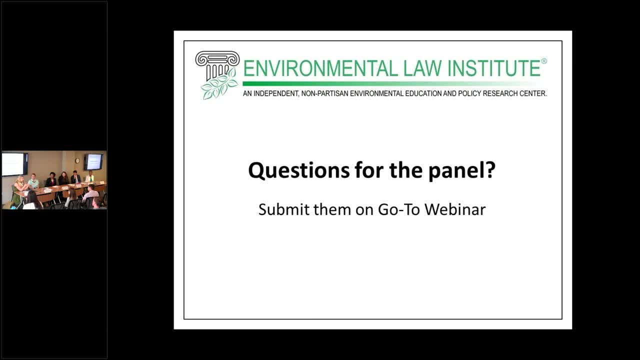 ago. So I think, depending on where you are in the organization and what's happening, change can be a good thing And it can open up a lot of doors Because people work there so long when we kind of separated into two companies, they 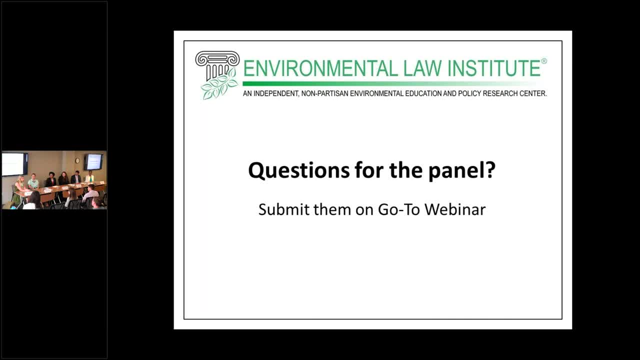 offered early retirement packages for a lot of people that had been there for those, you know, 30 to 40 years. We still have some that have stuck around because they really like live and breathe. National Geographic: They say they look like yellow blood, you know. 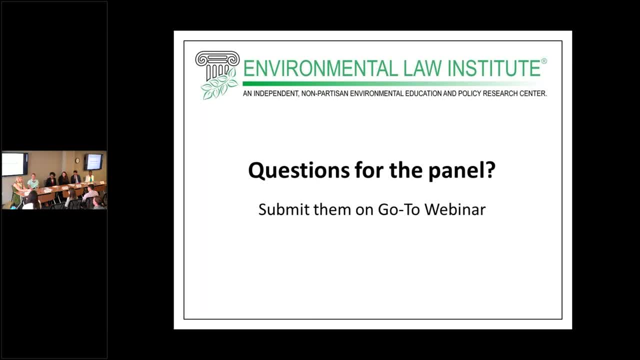 And so it's been an interesting transition, but at the same time it has opened up doors, And so I kind of see that continuing to happen. now It's just kind of a new age there. So I mean, I don't think that's definitely the right career path at all organizations. 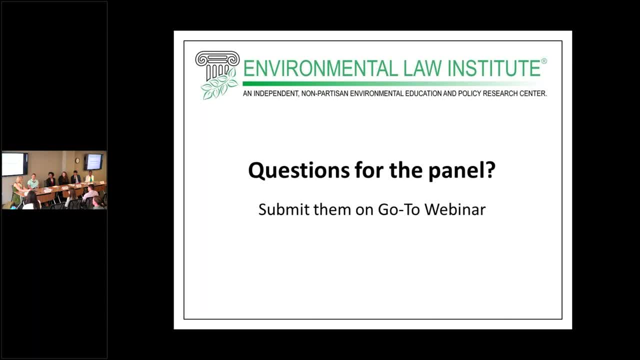 It really just depends on what's happening and where you see yourself going. Thank you, We're going to take a quick question from the web and then we'll go back to the room. So someone online said: first I wanted to say thank you to all the panelists, especially. 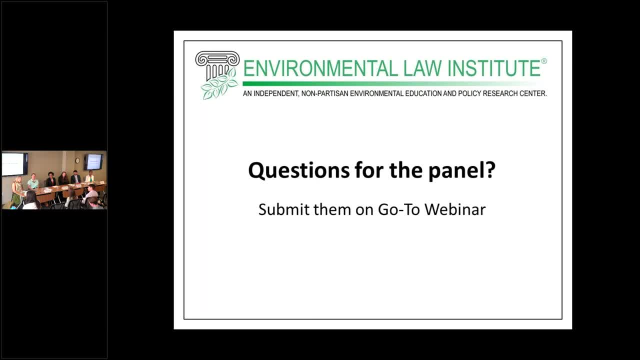 Nicole. As someone who has recently graduated with the JD slash LLM, I appreciate her candidness on the subject. What advice would you give a researcher? I'm a recent graduate with degrees in environmental law who wants to transition from working as an environmental policy fellow in a federal agency and wants to enter the private or 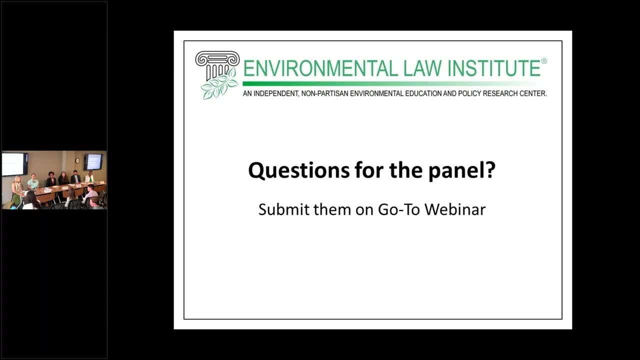 nonprofit environmental arena, specifically with environmental justice issues? That's a great question. Thank you for posting the question. I actually- this is a subject that I just had breakfast with someone about- who's trying to make the transition out of an NGO. 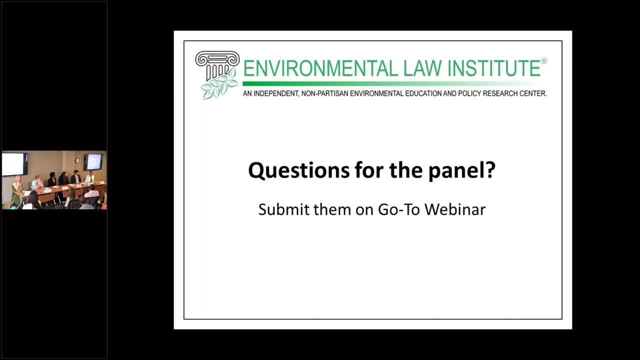 And I think that's a great question, because I think that's a great way to get an NGO into the private space focused on clean energy. The best advice that I would provide is to one, on a very practical level, go to where. 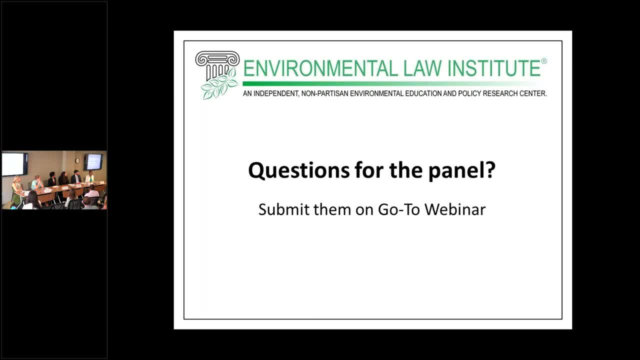 these organizations are hanging out. So if you're interested in the solar industry, go to Solar Conference. Go to Solar Conference, Just rub a whole lot of elbows. Another space that I think that people kind of overlook in terms of building relationships in a variety of spaces. in this field, the regulators have their own get togethers. 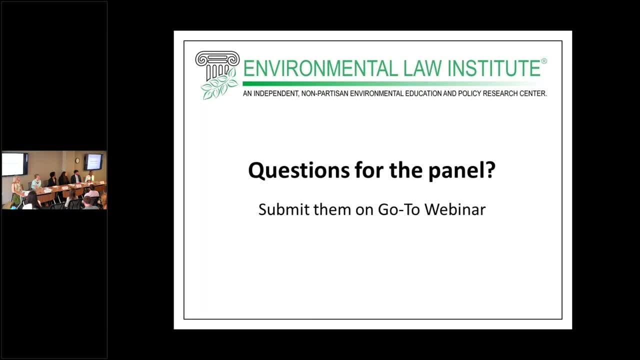 And sometimes those get togethers are open to the public. I would encourage folks to get to know some of the regulators. This is in most fields. A lot of this is relationship driven, So you get all your skills and credentials in school and you do all your internships. 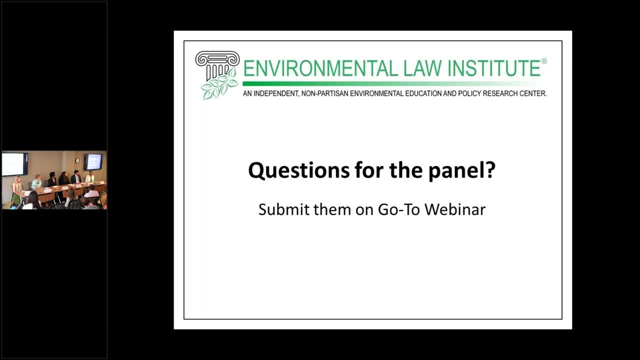 and fellowships and such, but a lot of the way that people get these jobs is because they know someone. It's a message that I'm- you know that I'm raising, both with respect to diversity issues but in general, kind of trying to help the industry move forward. 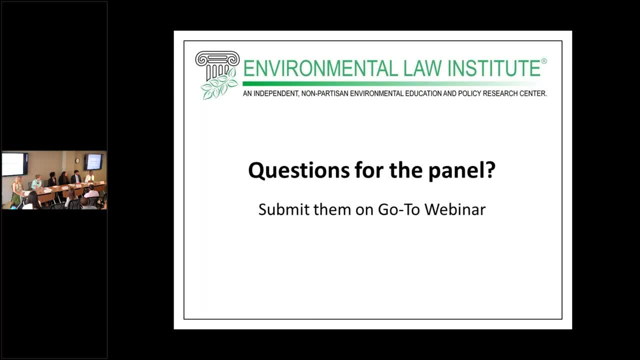 So I think that's a great question. You know, I think that's kind of what's happening in the industry is that the industry is moving itself forward to open the door wider for more people to get in. So that's, candidly what has worked for me in terms of making a shift from one space. 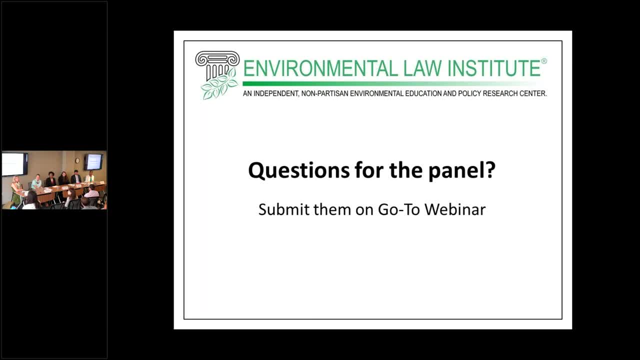 to another. Great Thank you. We have another question in the room. Hi, my name is Deepthi Bansal and I'm a rising 2L at GW here in town And I just had a question. I know one of you mentioned that. 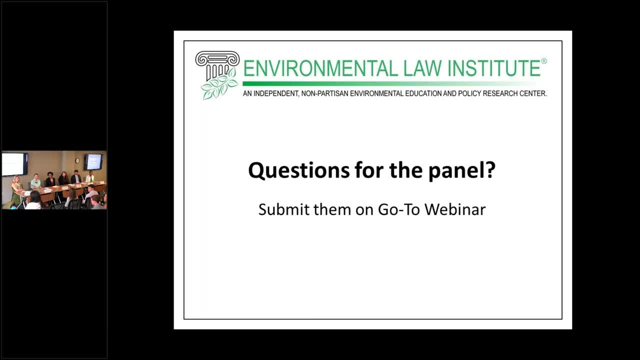 your dream job has changed over time. I'm just curious to hear what are your current dream jobs. if you're not already in it, I'll start, but I'm not going to be the only one that goes. So I would like to be in a position where I'm running, I'm like focused on the wildlife. 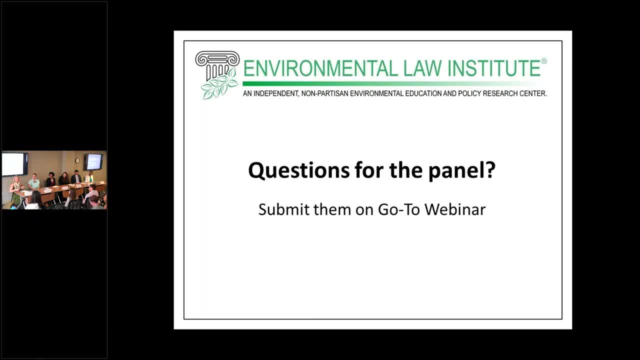 land, so where I'm running like I'm the VP of programs for some sort of impact-oriented place. I also think it would be kind of fun to get into the sustainability world Margot, So like working at like a well-known brand that we all know and making sure that they 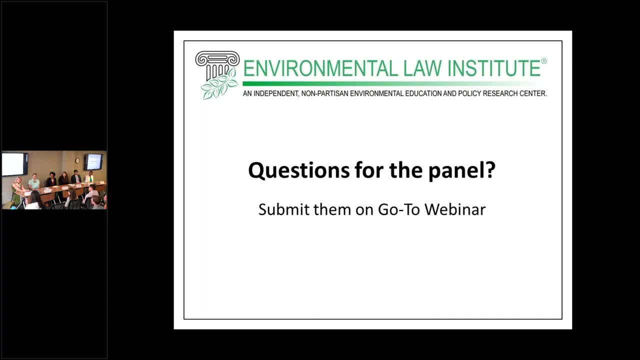 are. you know that everything that they're doing is going to be- you know, going to be- successful. So like we're doing the sustainable thing, but then also like we're giving, making sure that, forming partnerships, let's say: 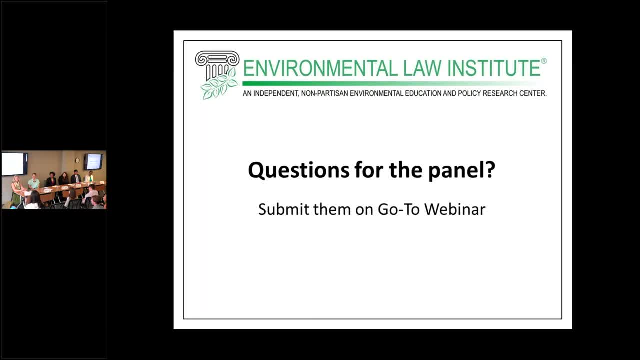 So, like I'm being at the National Geographic site, a few years ago, we did a partnership with Tom's Tom's Animal Initiative and they kept the Big Hats Initiative, which is one of my big projects, And so they made backpacks and shoes with animal print on them, and it was this really. 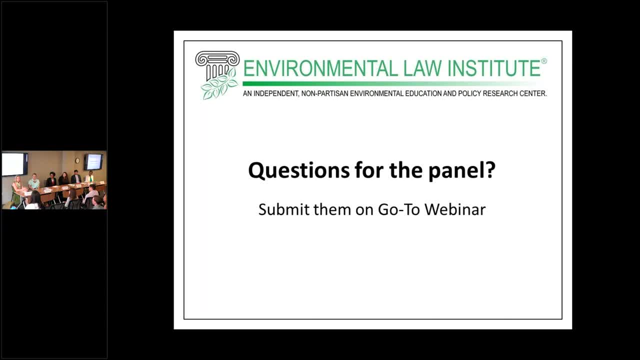 cool, fun way to get the message out. I think it'd be neat to work on the Tom's side of that and run that side from like a big company or organization like that. My dream job is super similar to that. I. in the future, I'm really interested in potentially moving to the private sector and 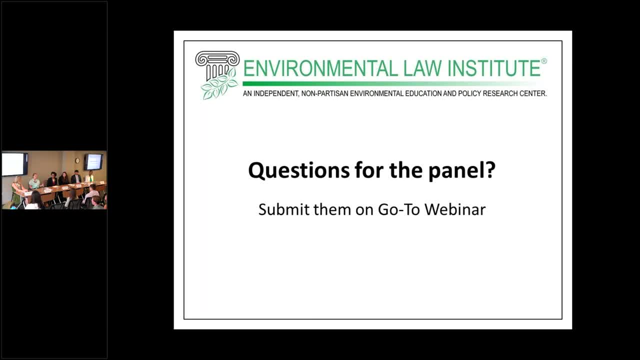 like many years down the line, perhaps being the director of sustainability at a big brand, so that I can kind of combine the partnerships stuff that I work on now with some of the direct supply chain experience that I have and work on building out corporate policy directly instead of working in an advisory capacity. 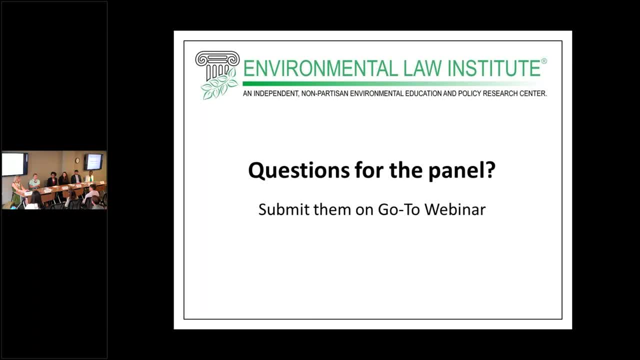 For that, and it's also really interesting how much collaboration there is between the public policy, NGO and corporate sectors around sustainability issues. So it would be really awesome to be in the middle of that vortex, kind of as the choir conductor for all that stuff. 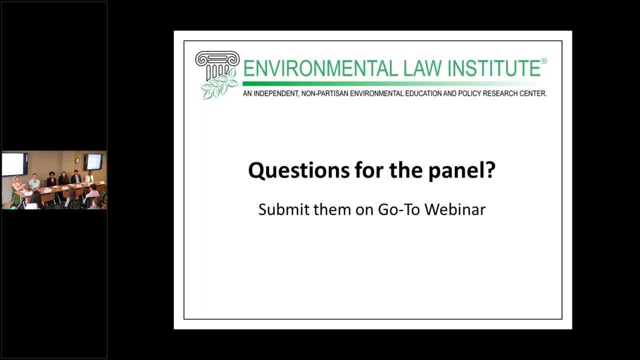 Oh, that's a. that's a tough question. That's a great question, Thank you, Thank you. So my dream job would certainly build on the skills that I have, the basic science knowledge that can inform, hopefully continuing forward in environmental health policy. 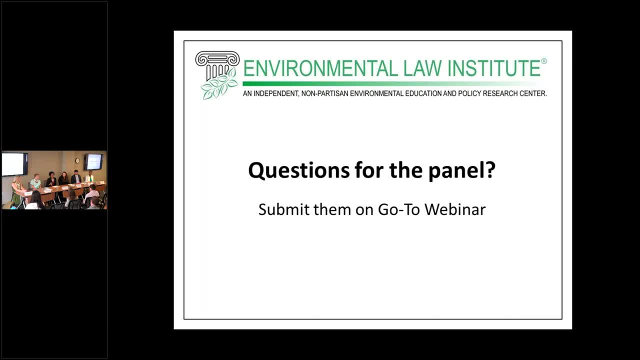 Also, I have a secret love of graphic design. Something could incorporate that. I don't know how I can weave that into something, but any opportunity to get to use that side of the brain, It really frees up my creativity and thought on this side of my brain as well. 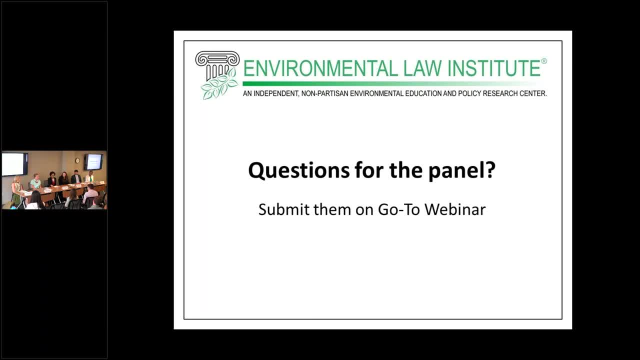 And then I would love to be able to engage environmental justice communities directly and effectively and continuously and be able to make sure- and we work to do that, but ensure- that they're at the table and that their expertise is utilized to inform future decisions. 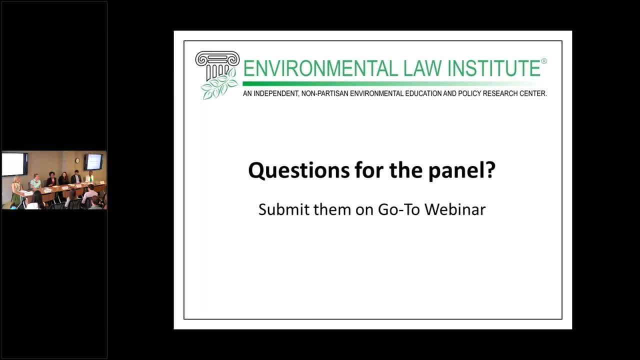 And, ultimately, my dream. I hope that's what I'm trying to achieve and where I can really truly feel like I am protecting the health of people all across the nation. I always thought I would probably kind of want to be in government forever. 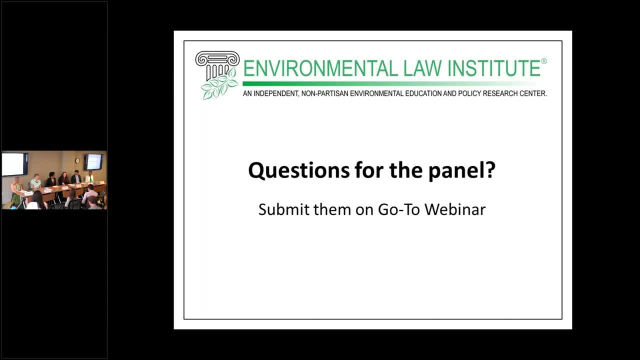 That's sort of what I thought even in law school, that I really liked it And I wanted to kind of be aware of policy is really getting made. That's definitely shifted over time, I think certainly recently too. I've begun to kind of reevaluate long-term what I want. 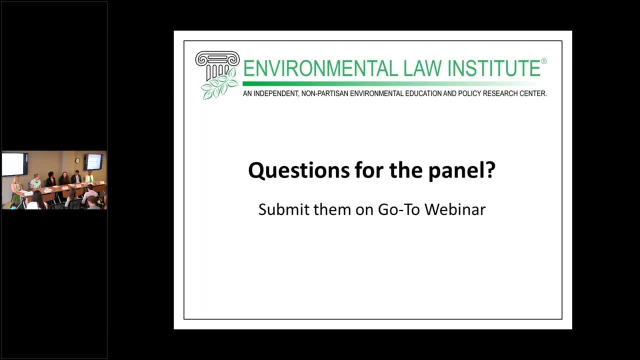 And so you know, similar to what Colby and Margo were saying as well about the private sector. I think there's so much innovation that's going on in the private sector right now that I can see myself potentially moving there. you know, down the line And I think also to some. 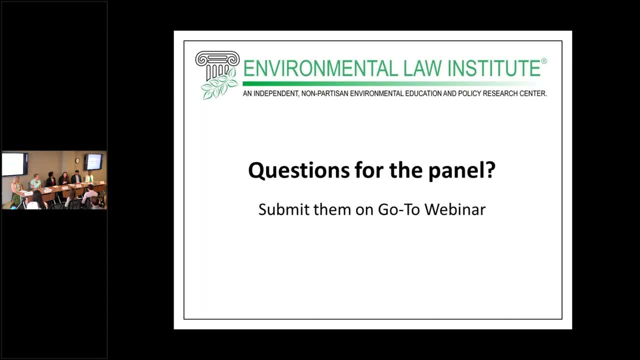 degree. if you're at a company or something, you can take ownership of things in a different sort of a way of an initiative of a project, where in government you know there are these huge bureaucracies and unless you're at the very top it can be a little bit harder. So I don't entirely 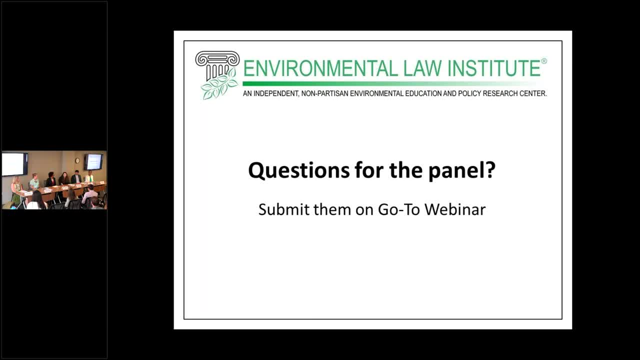 know yet what I want that to look like, but I think it might involve, you know, the private sector or possibly maybe moving to the Hill or something like that. But yeah, I think, you know, long-term it's kind of evolving, I'll be the one to say. for me it's constantly changing And some 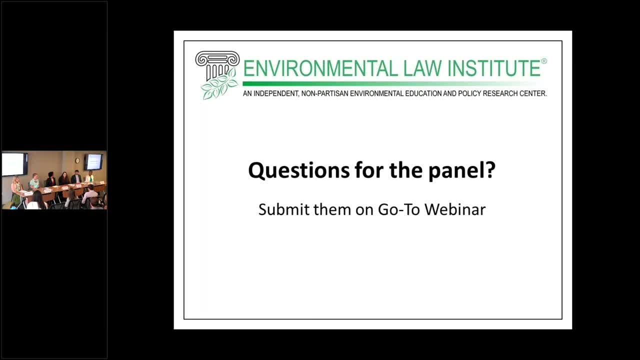 days I think I want to do one thing, and then, when I grow up, and other days I think I want it to be something else. So, yeah, Yeah, Just to piggyback off what Stacey said. I mean, I didn't make the 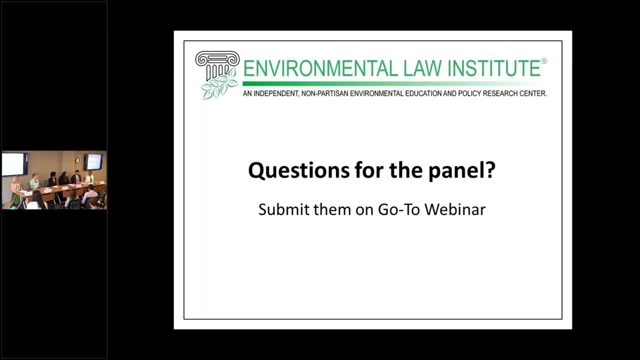 comment, but the way that it hit me was personally I don't know. I mean I never thought I would have been happy doing. I mean I absolutely hated Chemistry in high school and college and growing up. If you told my chemistry professor that I 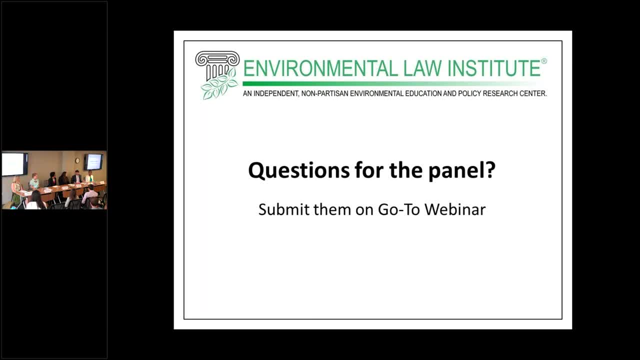 helped write the law that regulates chemicals. she might move to Mexico or something to get away from it. So you know it's just an evolution And what I like today, you know it can change. Yeah, I would agree with that actually, because 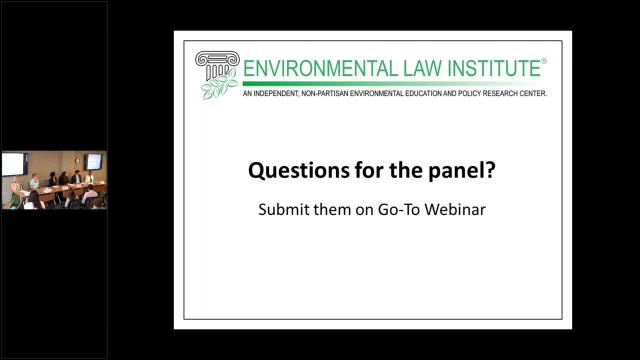 I guess I'm reaching a certain age where I'm kind of, you know, letting things flow And I used to be very driven when I was younger, but I'm a little less now. I'm certainly driven by the issues that concern me and facilitating a cleaner planet and climate change and consumer empowerment things. 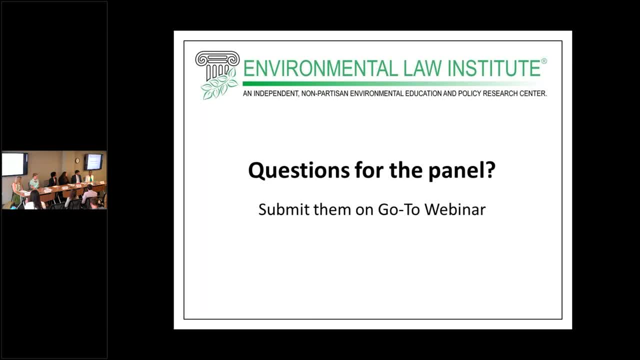 But I'm realizing that there are many ways to address those issues. So I'm kind of. my dream job is to be able to do that And I'm kind of you know, I'm kind of you know, I'm kind of you. 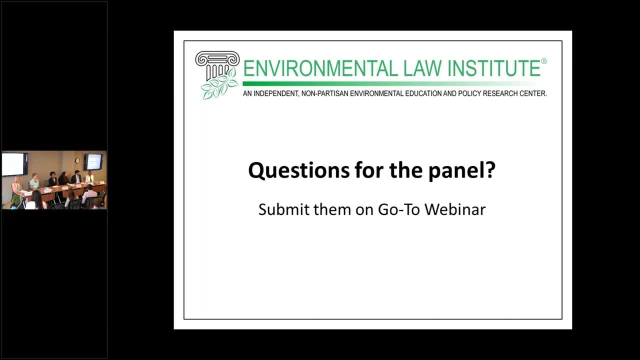 know having a job as one that pays the bills and enables me to take great vacations and where I'm also doing good for people in the planet. And just I'll kind of revisit it for a second kind of what Nicole was saying, too like I think. 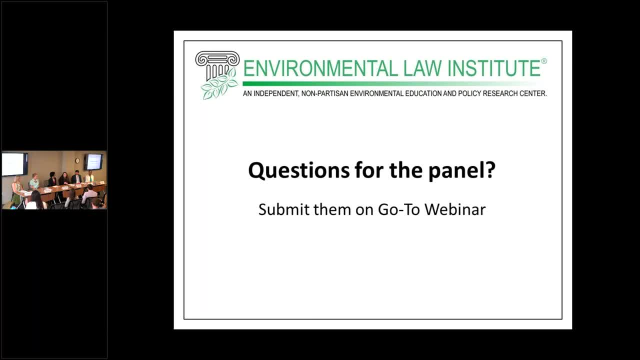 that's what it is. It's about finding something where you can have an impact. So for me, if that's staying in government, I'm happy to stay in government. If it's leaving at some point, I'm happy to leave, And so I think probably a lot of us feel the same way. It's like where we can have the most. 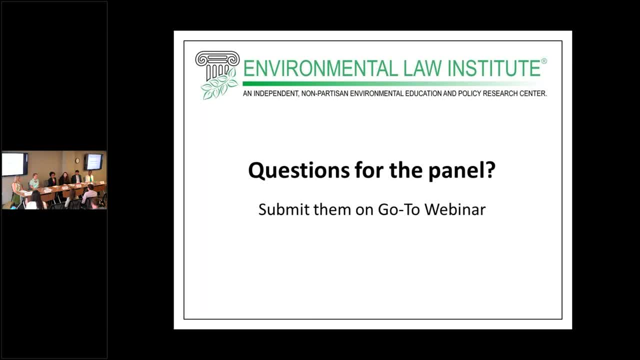 impact about, on the things that we care about, And yeah, and I would just plug also in the line with that that, um, there's a lot of really amazing organizations sounds like. for example, Nicole is involved in a lot of stuff as extracurriculars throughout, like being pop at the Sierra Club. I. 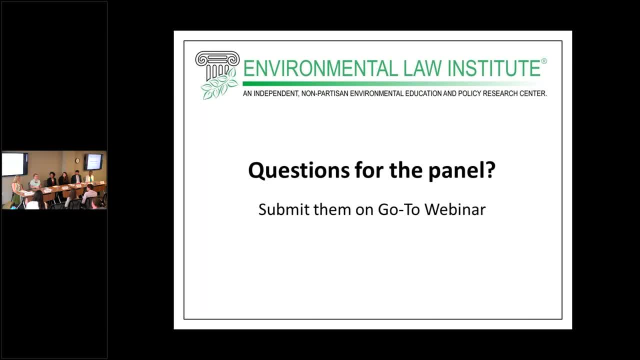 manage a community orchard in DC in my spare time because it's like away from you literally get my hands dirty and work on urban agriculture here and to connect to community that experiences student security through that. so you shouldn't limit your thinking to your impact just for your job. there are so. 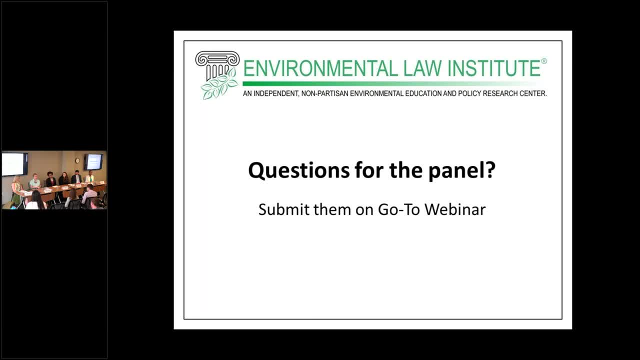 many amazing ways for you to impact the issues that you care about in many ways, and a lot of them will end up surprising you in the way that they do end up connecting to your career in the long term through the relationships or the skills that you gain there. great, thank you. so we did have another question from 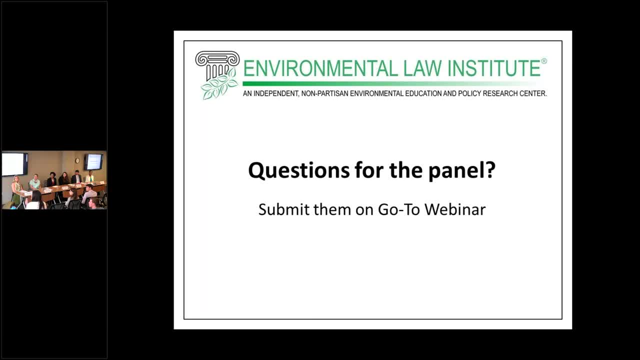 the web and it was: how important has mentorship been in your career and how did you go about developing relationships with your mentors? I'll speak, I think very important and still developing, I think, are the two things. so I do think it's really important to find, you know, a couple key people who will 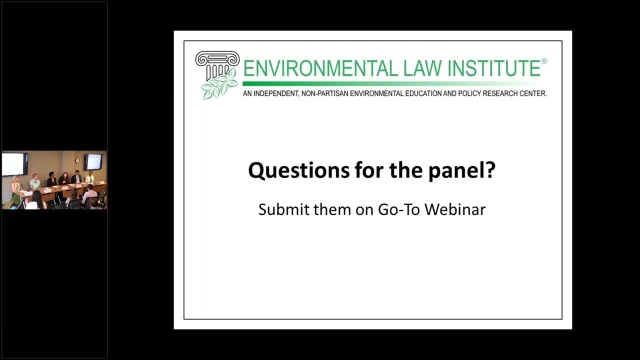 sort of like be your advocates, who know you, you know, know your work like you know you're, you know like you get along well with, you know you're like you get along well with you know you're like you get along well with, who are willing to go the extra mile for you. you know whether it's a 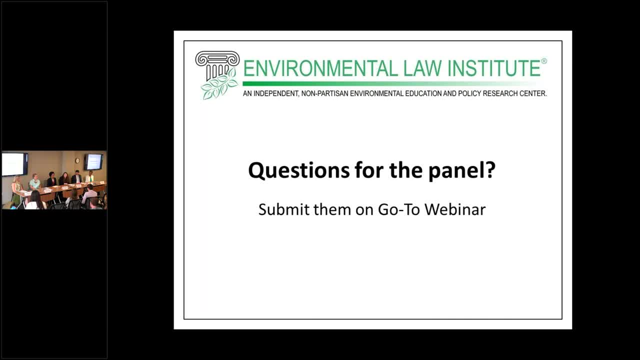 recommendation or, you know, sending a you know job your way, or asking about opportunities that you might not know about on your behalf. I mean there's a lot of different things, but I think just just finding those people who you can really rely on for sort of candid advice, I mean to me that's sort of the biggest. 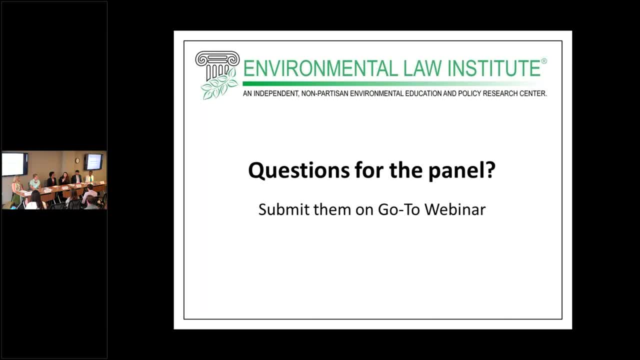 thing and how to find them. I think it depends. I mean, you know, I know people where their professors or their closest mentors. for me it's been some supervisors I've worked with who were just amazing and just felt like my biggest cheerleader. so I've stayed in touch with them and I think it's really 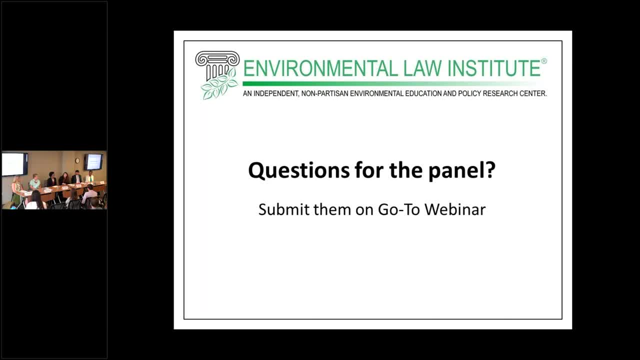 important to have those people who are just amazing and just feel comfortable picking up the phone, whether it's about you know a job, a career path, whatever it is, or you know, if this is where I want to get, is this the right path- and just those people who will support you. and I think it's kind of a strange way to say. 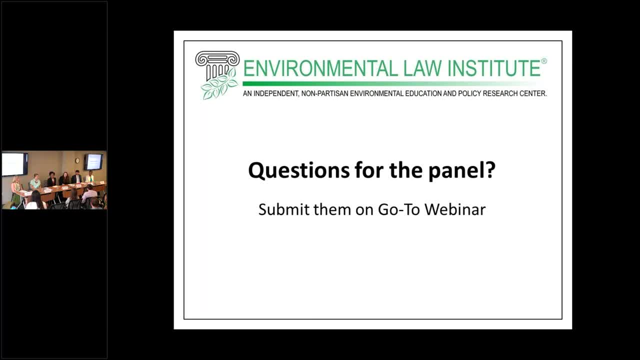 it, but I think you'll know them when you find them like there are some people who you'll just click with and are happy to meet you, you know, before work, after work, you know happy to take a few minutes during their hurried lunch break to talk with you. so I think it's very valuable and I think it's really important to have. 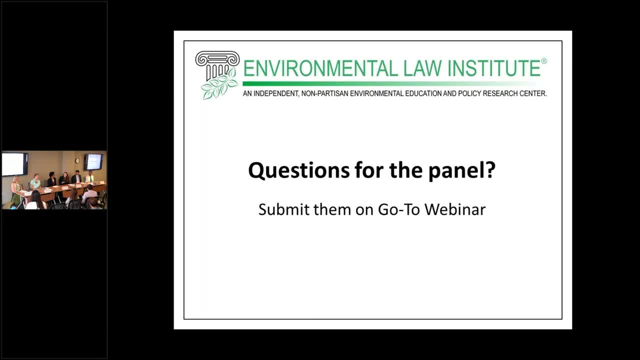 people like that. I think that's a powerful tool for you to be able to connect with and to be able to keep in touch with them. but yeah, I think it's that kind of thing. you can sort of find them anywhere, but just you know, hold on. 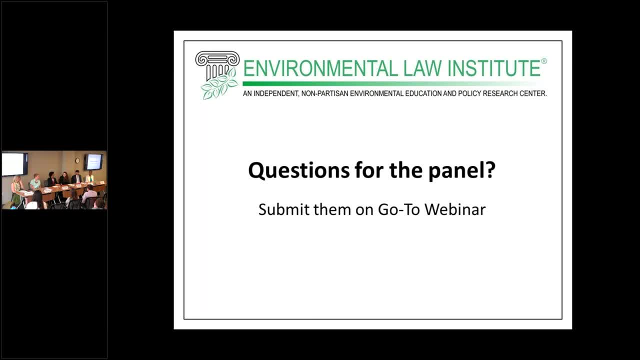 to them when you do. I completely agree. I, when I was in grad school, I had mentors that were fantastic mentors and it was situational. it was because I was in grad school and this person was my advisor and I told you about one he picked up on. 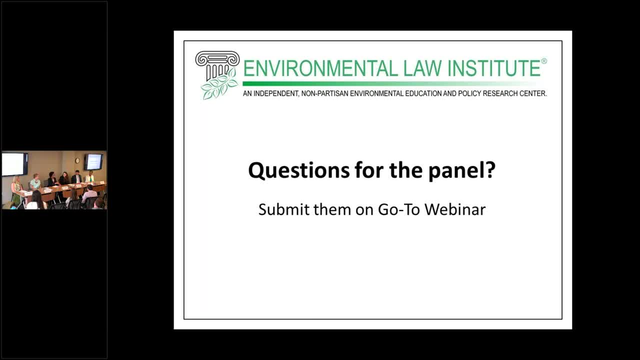 a mentor of mine, um he, when it was time for me to um do my uh, apply for my degree, so you, you have to finish that semester- i said, is this the right time? can i finish this in this amount of time? and he was like, yeah, maybe it's gonna take a lot of work. i don't know what that means, but i went ahead and 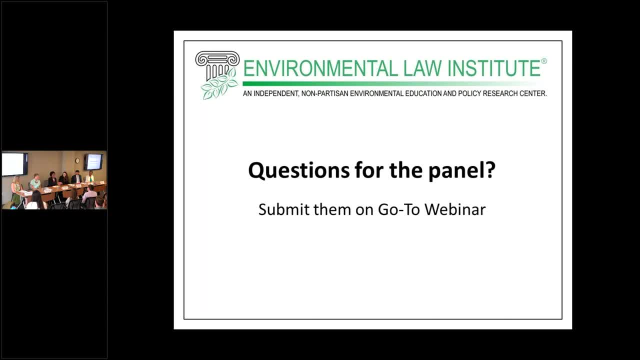 i applied and i could see that he was actually working just as hard. he was putting in as much as i was putting in to help me get out the door. um, mentors, open doors for you. and then my- uh, my mentor into my post-doctoral program. um, i learned through his example very much, so i saw how he 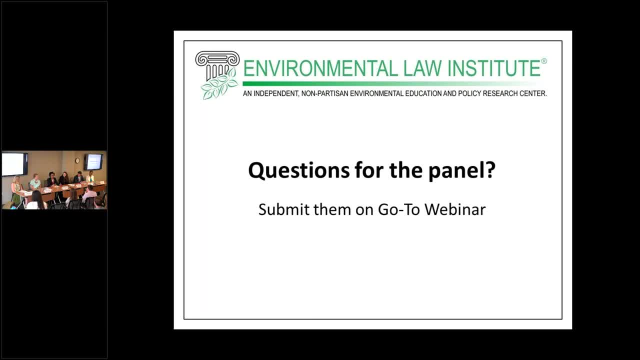 not to tell you, i'm not to have a social life, but worked around the clock and put it, put everything into it and that showed me, okay, this is what is expected to me, to make it to that next level. now i'm at the point in my life and these people are. i'm still in constant contact with these mentors, but now i um. 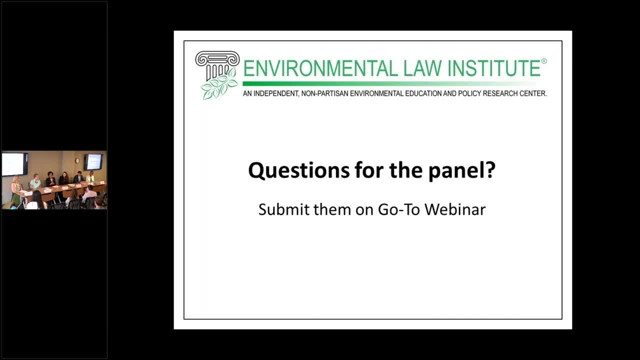 i was given some really good advice by my aunt. she was like you need some mentors, um, that are like you kind of age, um kind of gender wise, uh, you know, um social settings similar to you, have your educational background but are advanced, um, you know, they're at the level that you want to be. 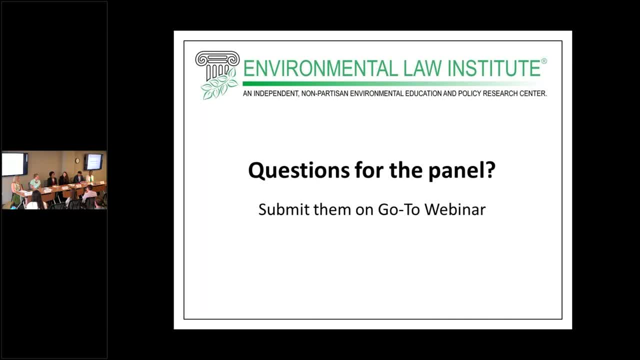 uh, to kind of help show you the ropes of how to get there. so i'm recruiting folks and- and i i have a couple great mentors in that space right now as well- and are really giving um, it helps to see people that that, uh, you can really identify with, but that can also have been there. 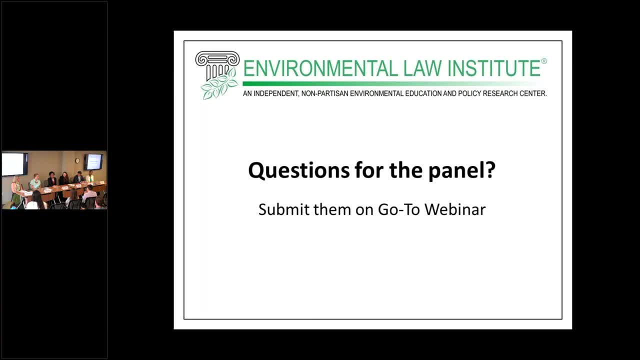 and done that and really, uh, it helps. so peer mentoring is kind of what i'm looking to right now, i think, just to really quickly build on what natasha said: be eager and show your interest. i think that's a huge part of it. i mean, you can go through an internship and you can sit in the office and 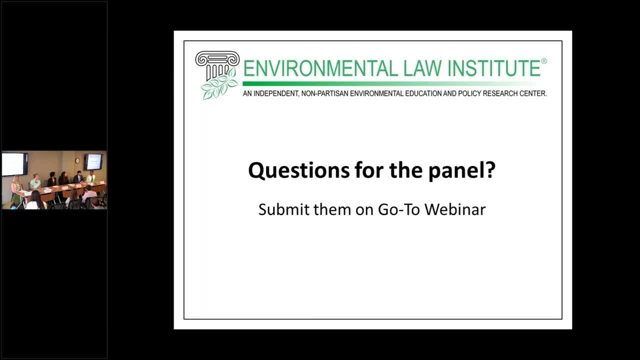 and not talk to anybody or not not let people know what you're really interested in. i know it's uncomfortable and i know folks don't like doing it, but go knock on a door, ask a question. tell people what you really believe in and what you're really interested in, because 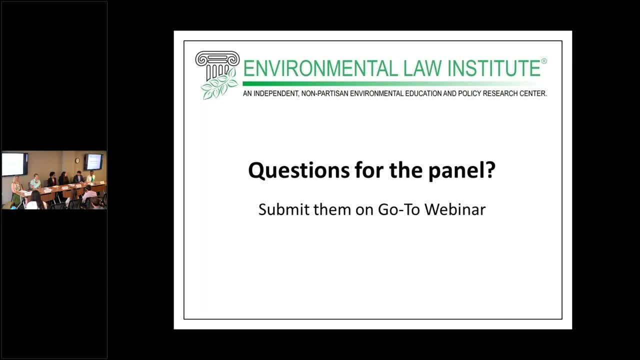 when they see the passion in you. that's when you know you find that mentor who wants to give you that you know level of work and help back great. thank you so much. i think our panelists will be here for another minute at the conclusion. if you have any questions, you'd rather ask them. 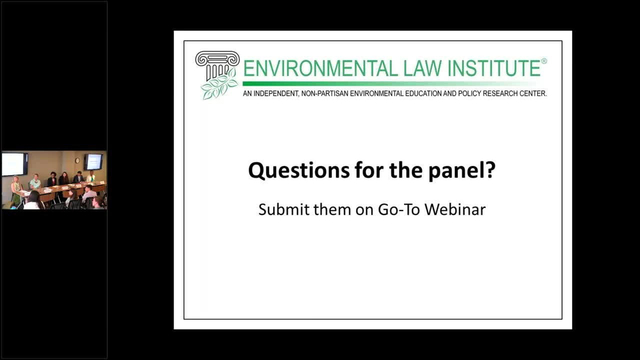 one-on-one, but thank you so much to our audience for joining us here at eli today and also on our online web, and thank you for your thoughtful questions. we hope you'll continue to think about the many varied roles and paths and environmental law and policy as you move forward in this sector. eli's annual summer school series is a couple more. 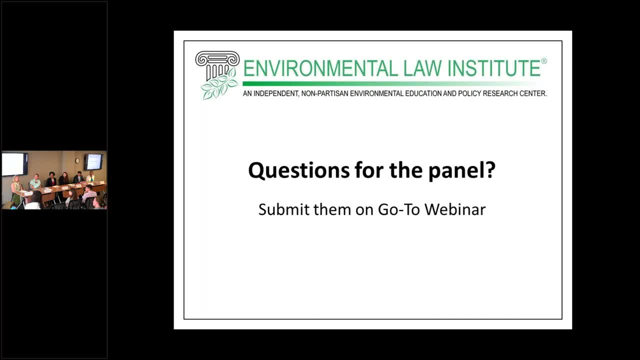 series to offer an introduction to the legal and policy foundations of environmental law in the United States. The series of brown bag seminars are taught by experts in their fields and we hope you'll be able to join us for later sessions on the major environmental statutes, starting with. 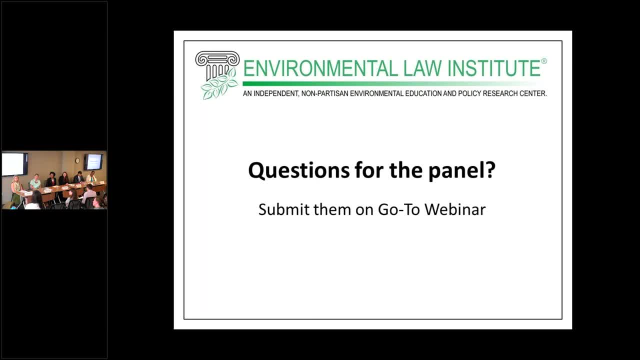 NEPA, ESA and fundamentals of environmental law next Tuesday. Register today for this and the other sessions on the Clean Air Act, Clean Water Act, TSCA, RCRA, CERCLA and land use law. We're so grateful for your participation in today's summer school and I hope you'll join us.